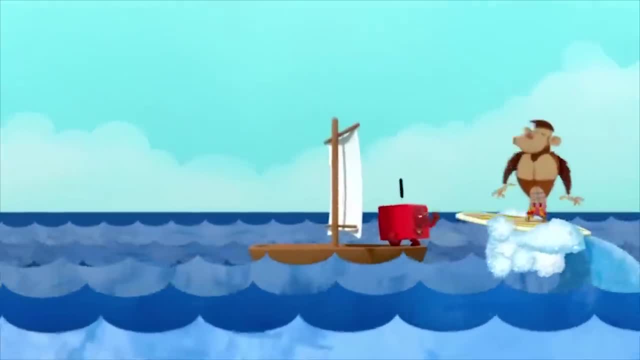 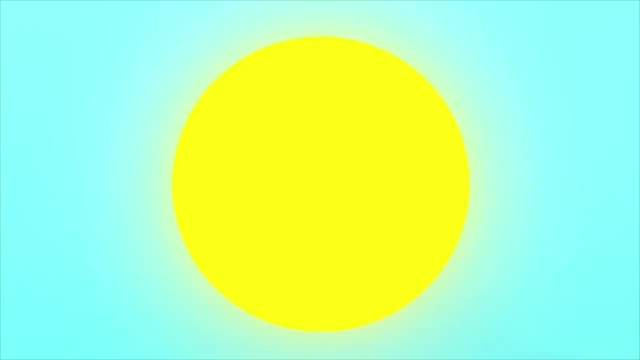 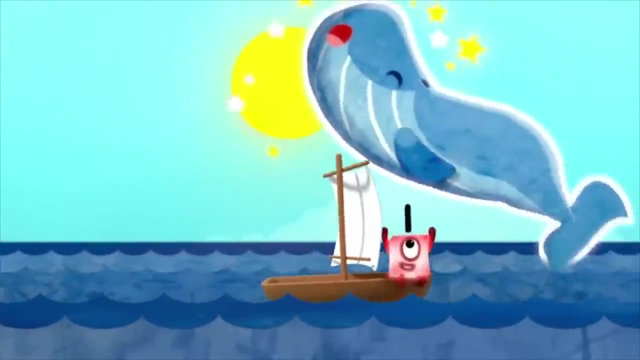 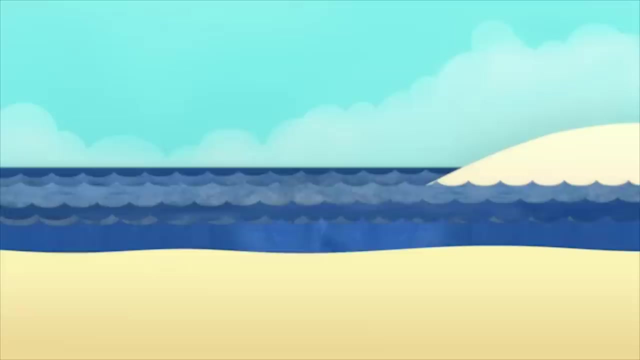 One whale swimming by one surfy chimpanzee- one wonderful world and one me. One one sun, one one sea, one one whale, one one chimpanzee. one wonderful world and one me. When you start to count, I'm the right amount. I'm the first in line. 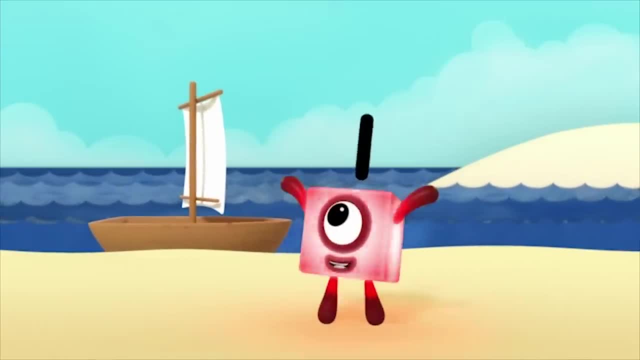 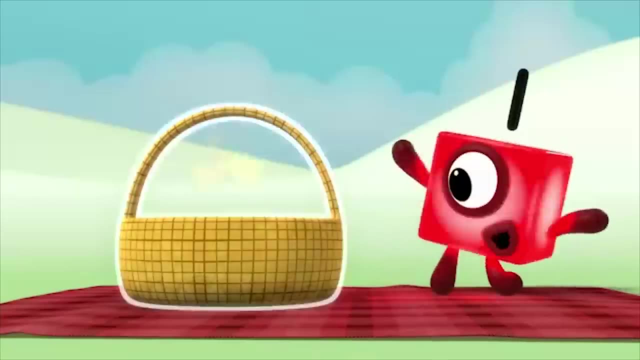 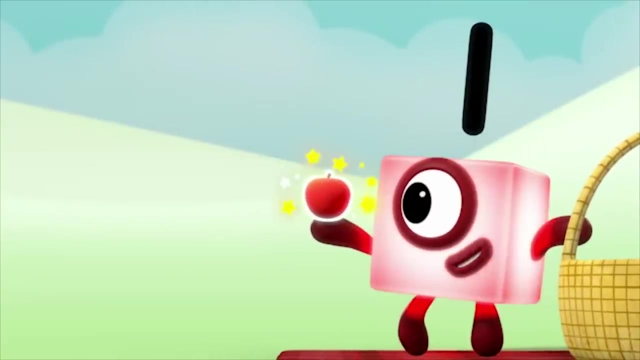 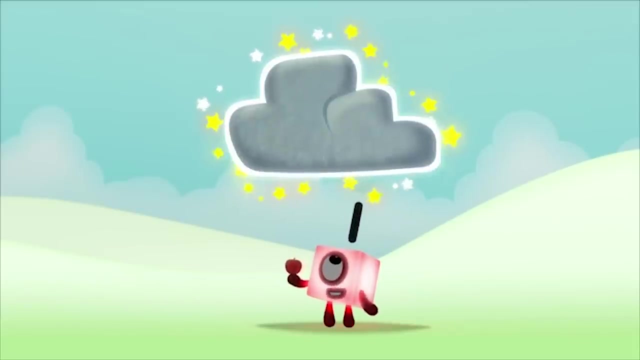 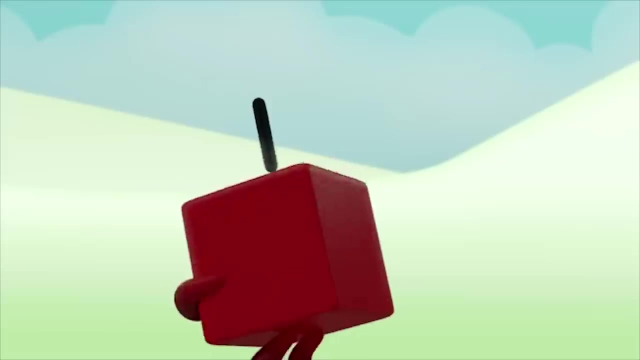 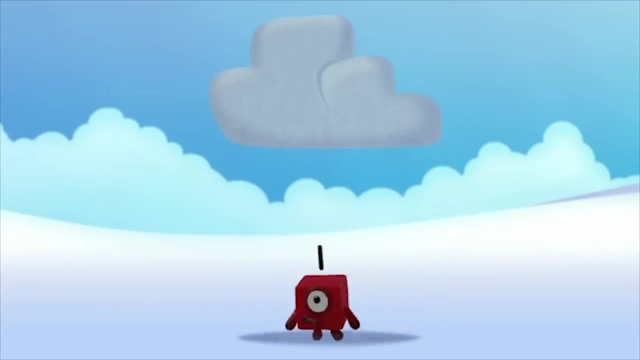 You can count on me. I'm one in a million, I'm one of a kind. Oh one one blanket. one one basket, one one apple, hello apple. One One. One one cloud, oh one one raindrop, ah-ha. one one umbrella, oh oh one one wet me. 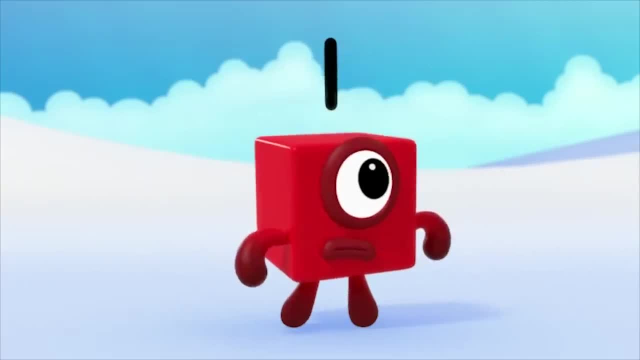 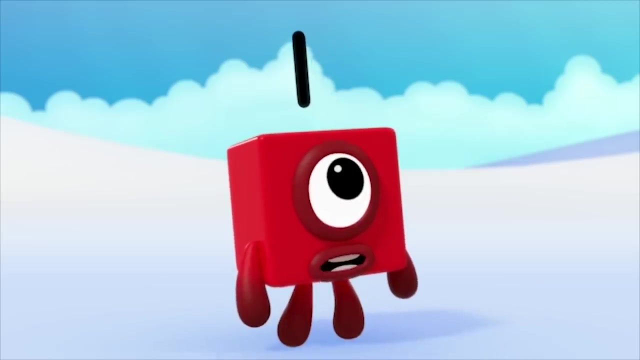 Did you see that, Hello? Oh, It could be lonely If I'm the only one. it might not be much fun being a single figure, But I'm number one and I'm winning. I'm only at the beginning. 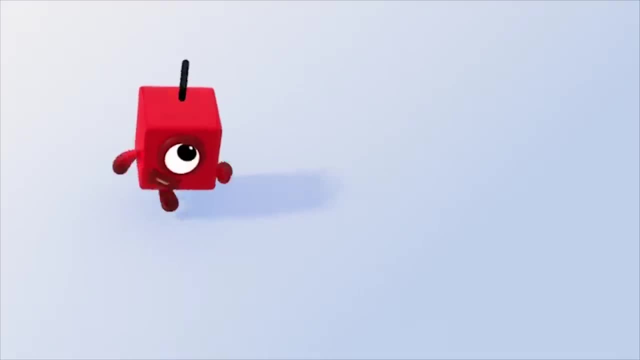 I could be the start of something. maybe I could be part of something bigger. One mountain to climb, one step at a time, One, One, And I'll always be the first in this race. One, One smile on my face. 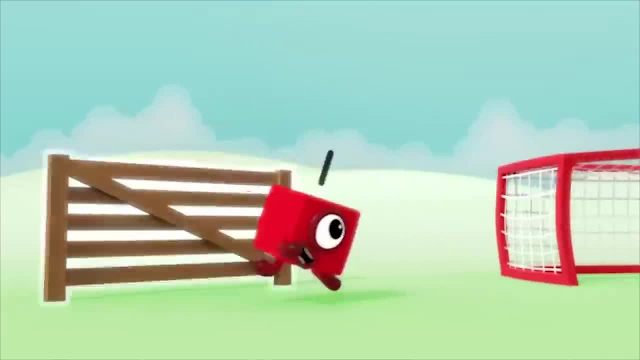 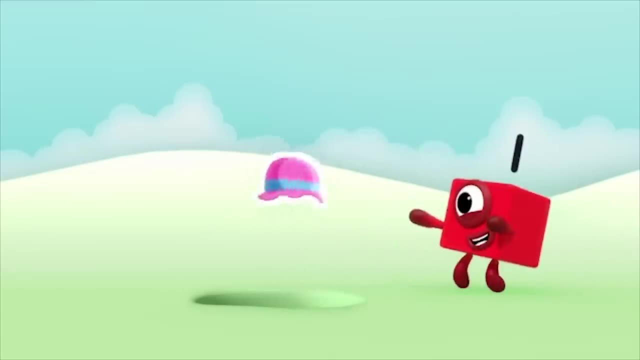 One bat, one ball, one box, one boat, one gate, one goal, one goose, one goat, one cat, one cow, one cake, one cat, one hole, one hop, one hen, one hat One wonderful, beautiful view. 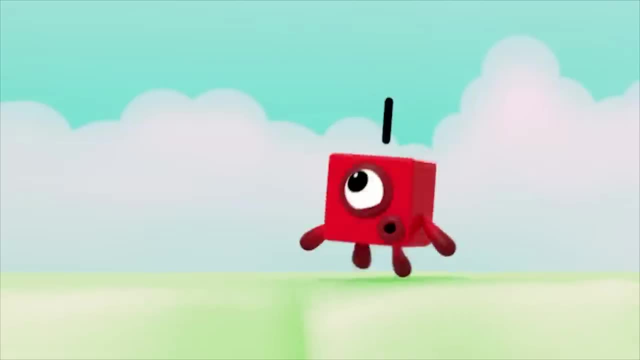 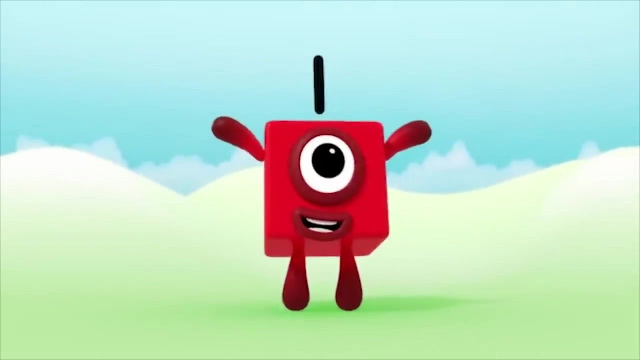 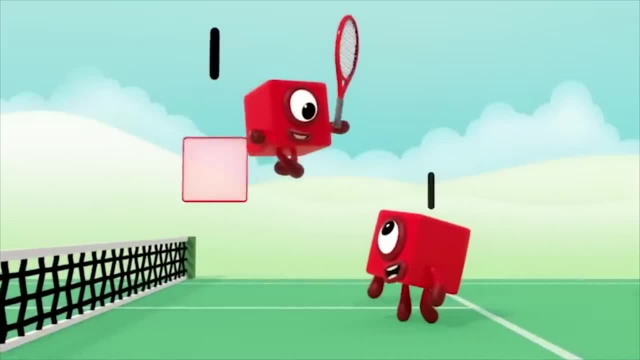 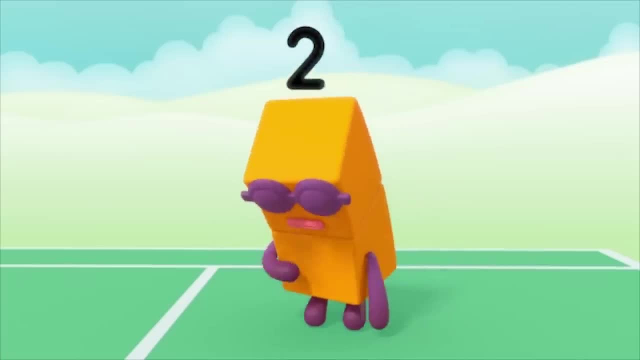 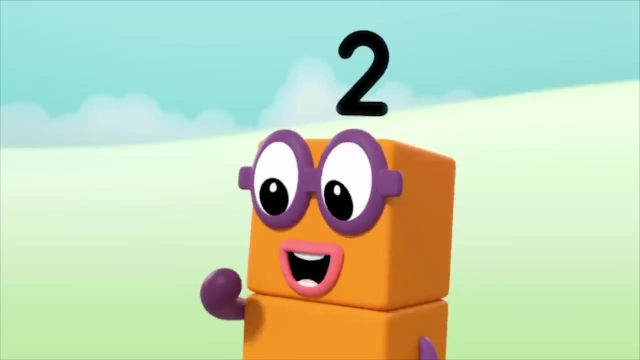 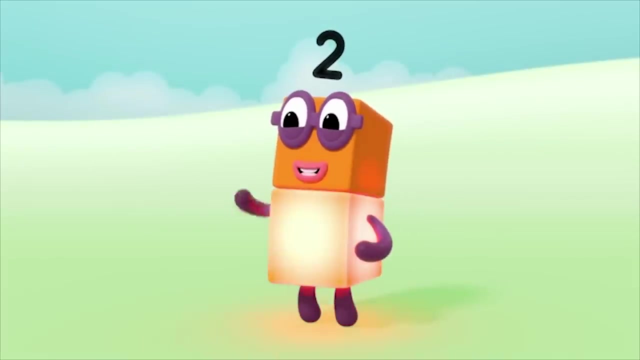 It's working. One plus one equals Two. I am two. How do you do? Where did they go? One and another one turned into me. They didn't go anywhere. One, two, Two blocks. I'd like to meet one. 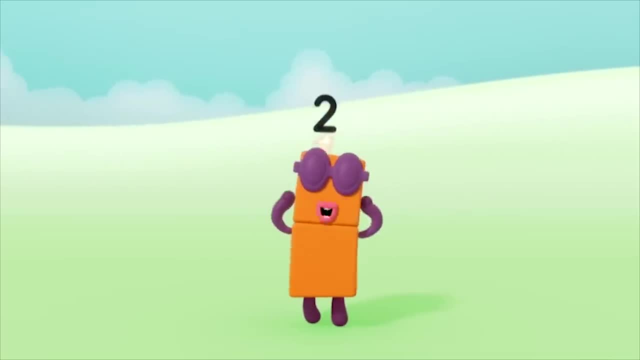 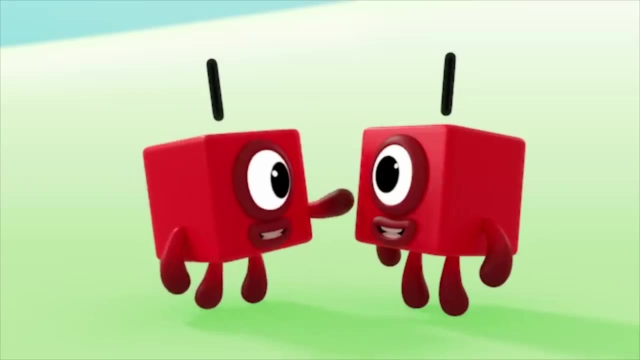 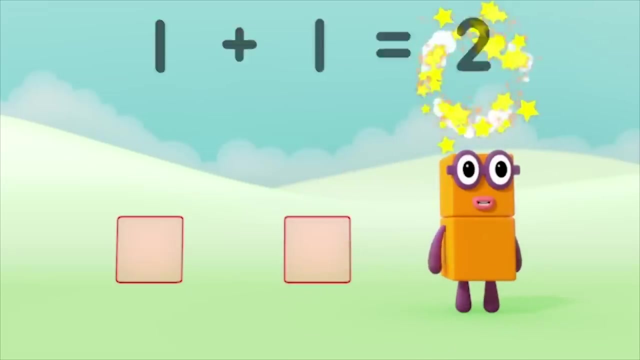 It would be nice to be her friend. Two equals One plus one. Wow, Did you see that? Let's do it again. One plus one equals Two. I am two. How do you do? Oh, Oh, Two equals. 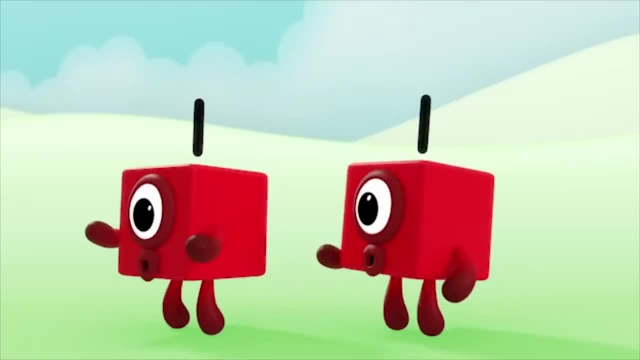 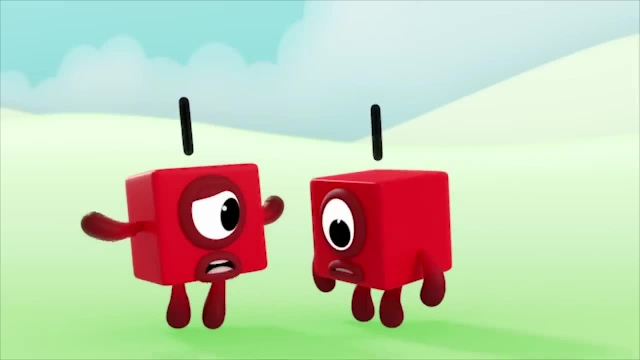 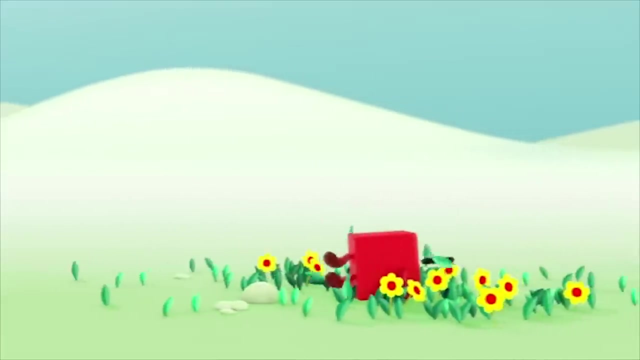 One plus one. Pleased to meet you too. two, Oh, We already tried that. What I need? another idea Got one, Oh, The magic mirror. Oh, Oh, Let's do it. One plus one equals Two. 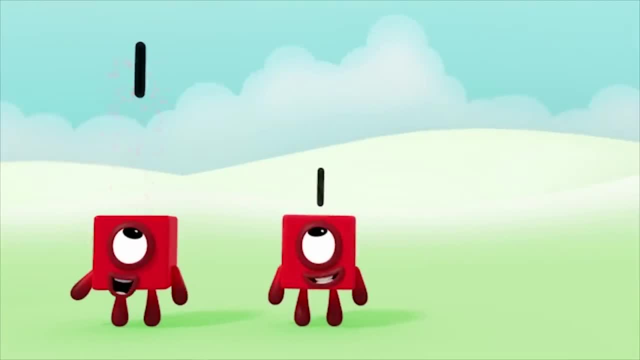 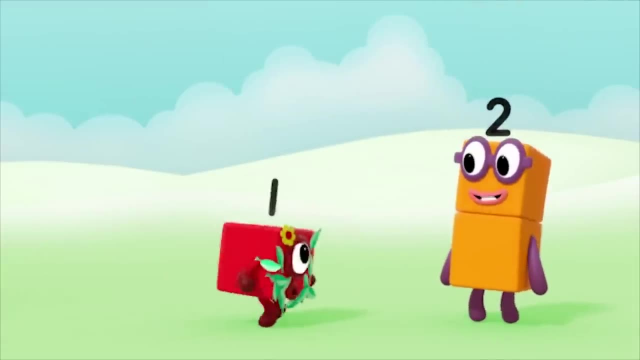 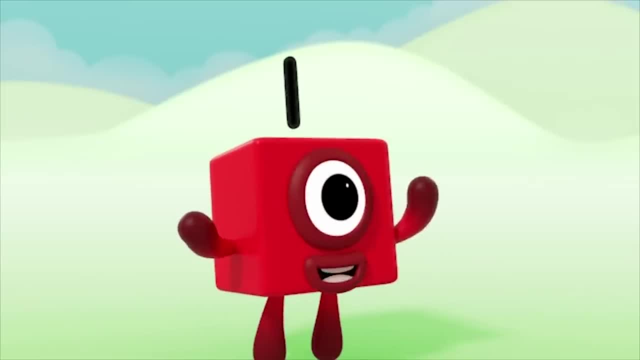 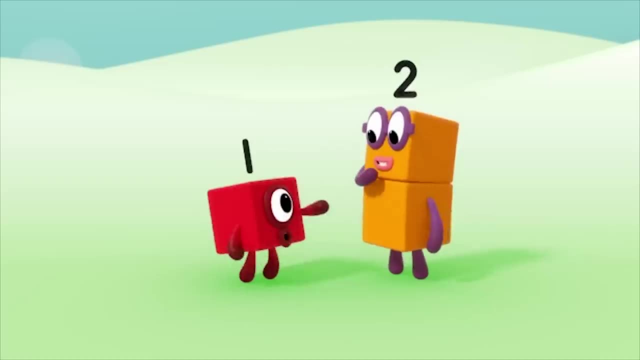 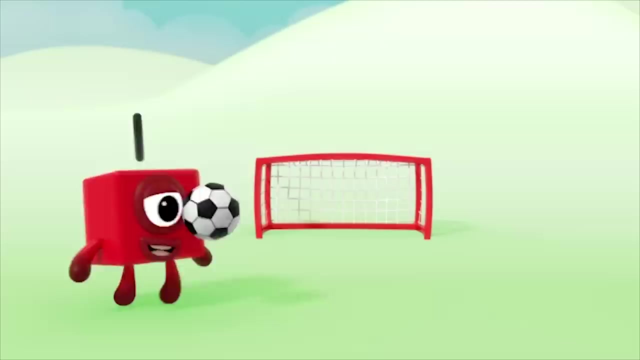 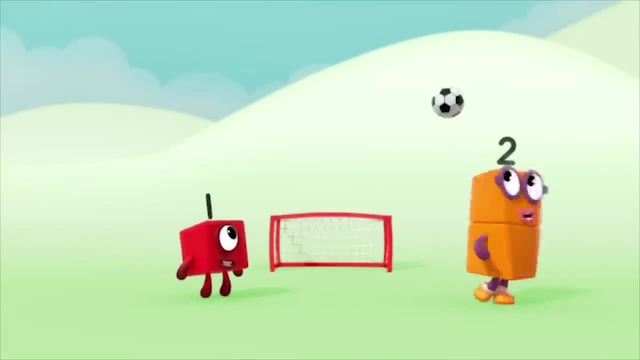 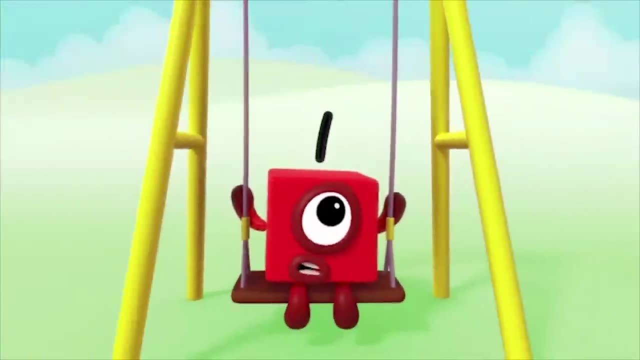 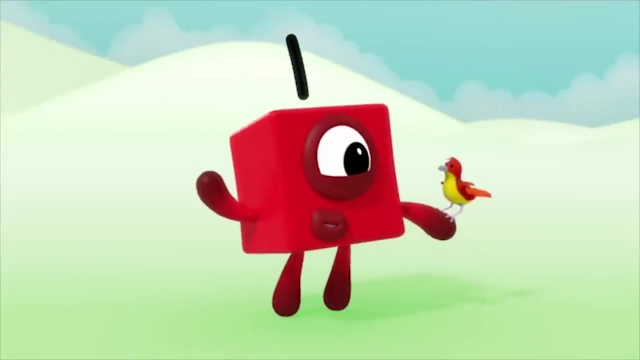 With two you can do a one, two, One, two. It's more fun to kick a football When there's someone there to kick it back to you. With one, the swings the pouring Cause. you need a friend to give you a push. With one, you can get a bird in the hand. 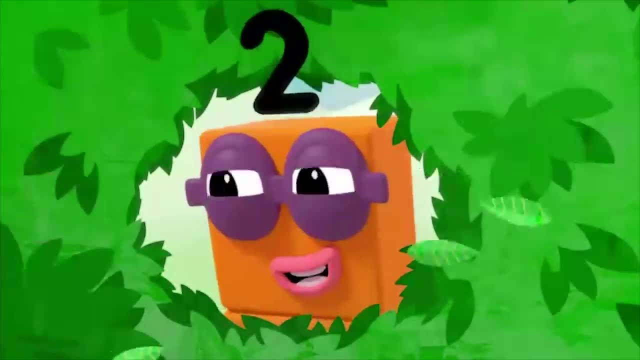 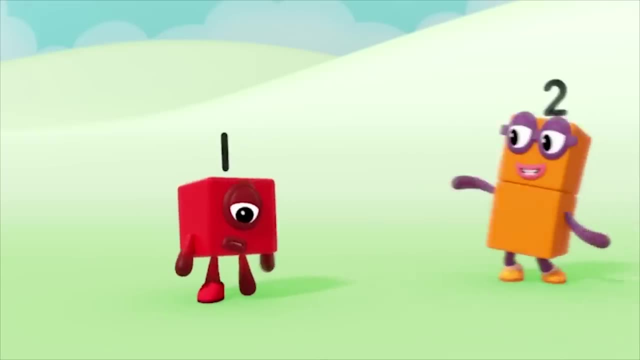 Oh look, there's two in the bush. One shoe just won't do. you'll end up all lopsided. One, two, two shoes you can use to dance like I did. One wing tied with string, no point even trying. 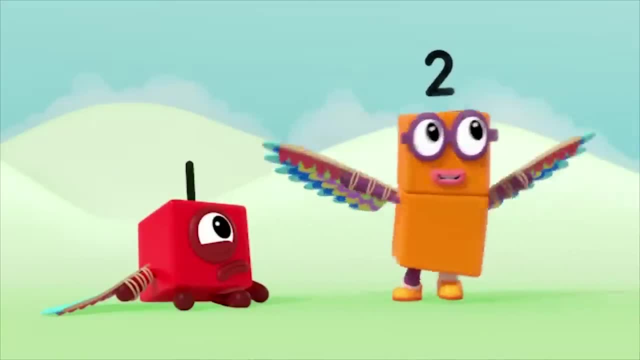 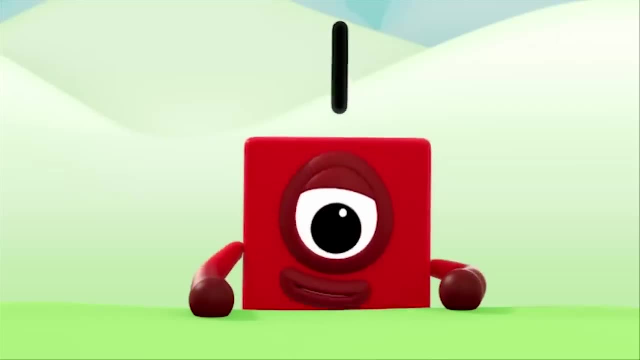 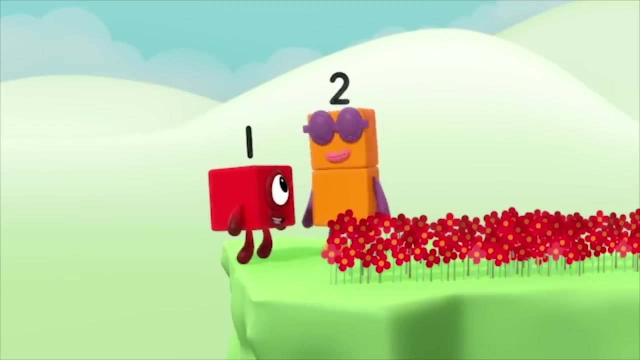 One, two, two wings and zing, you'll soon be flying. With two, you can get a leg up. With two, you can offer a hand. With two, you'll never be fed up, Cause there's always someone to understand. With two, you won't. 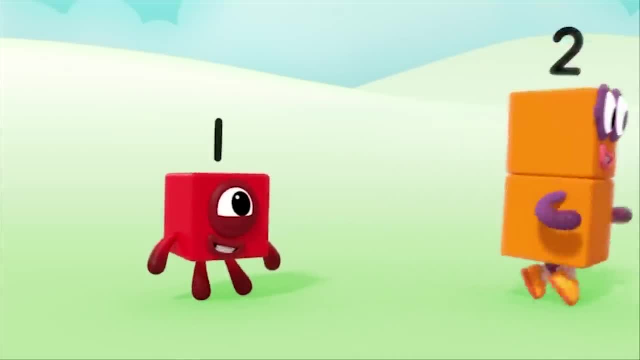 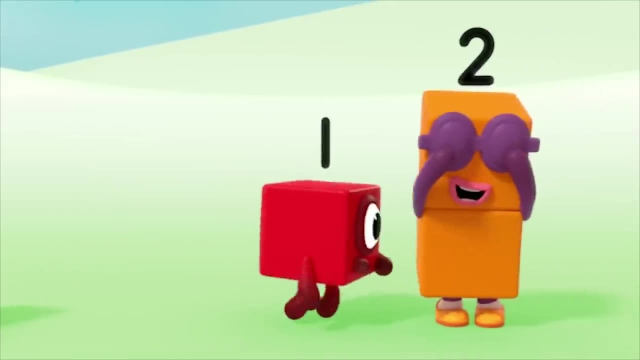 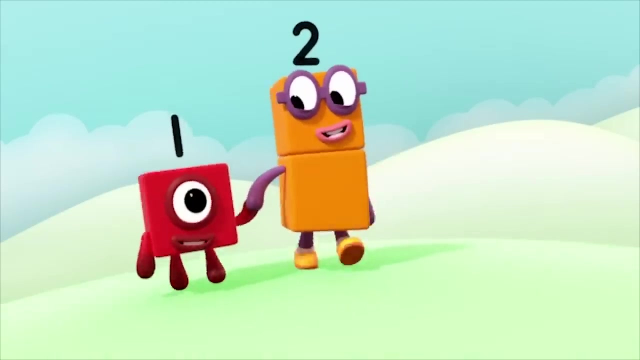 You won't be lonely and you're never gonna have to pretend. With two, you can play hide and seek. With two, you can find a best friend, Cause everything is better with two, The two of us together, just me and you. 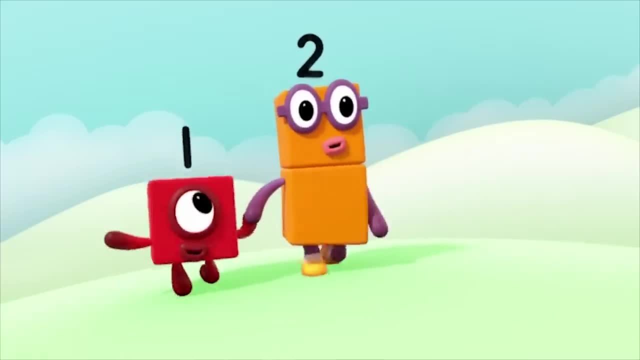 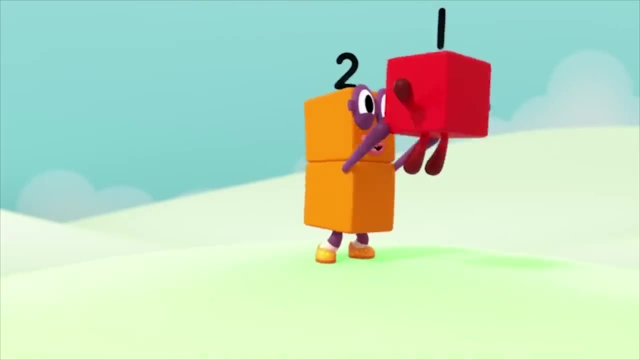 Imagine all the crazy things we can do with two. With two With you and me and me With you and me and you With two, we'll see what fun can be With you and me and me and you, And all the things we can do with two. 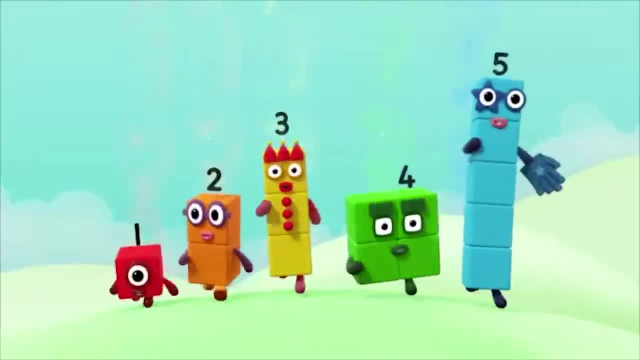 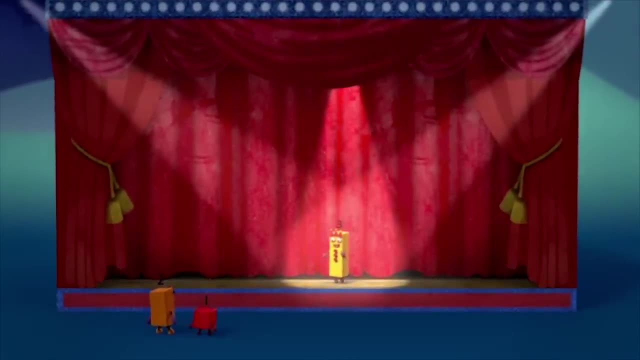 Best friend. Best friend, You can count on us. we're the number box: One, two, three, Everybody. look at me. I'm here to entertain you with this funky melody. I'll juggle three balls in the air and everyone will cheer. 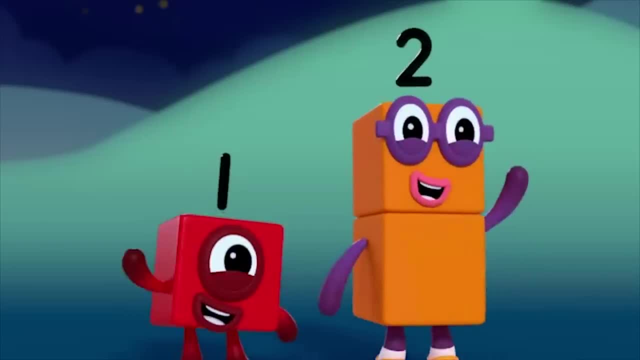 Yay, Everything's gonna be alright. now. number three is here. I'm in tic-tac-toe, I'm in ready, steady go. You're gonna have to count to three to get three in a row. You'll find me hiding everywhere you look. 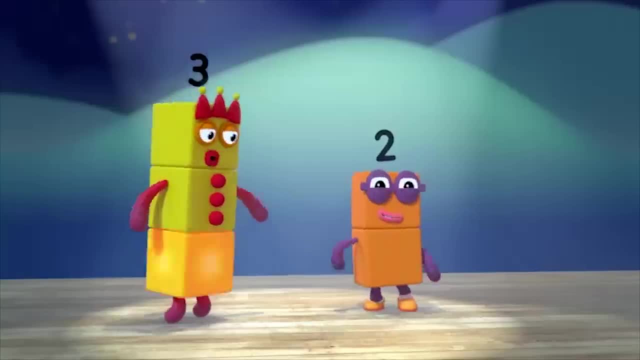 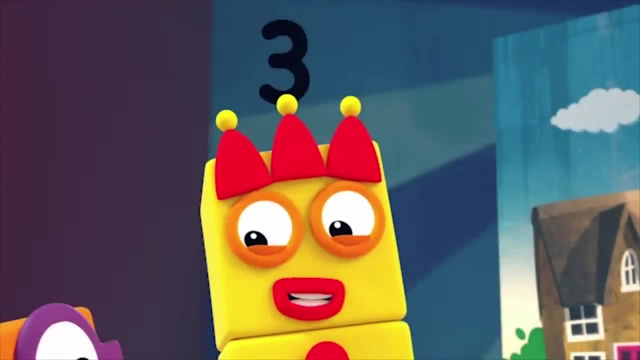 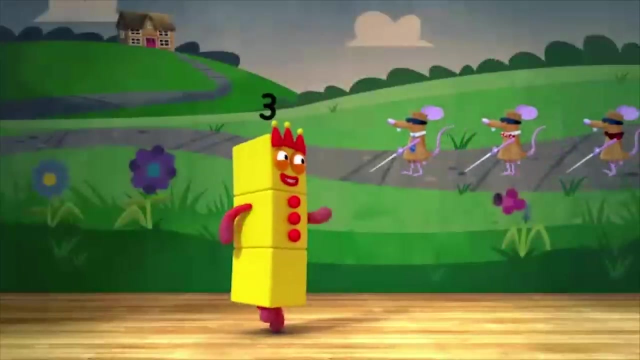 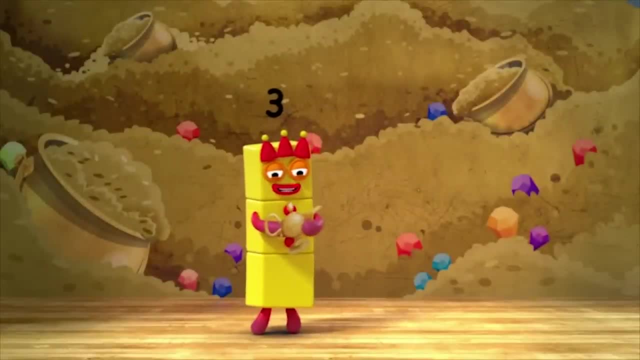 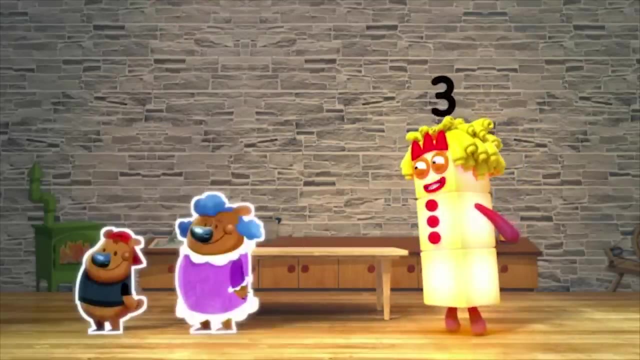 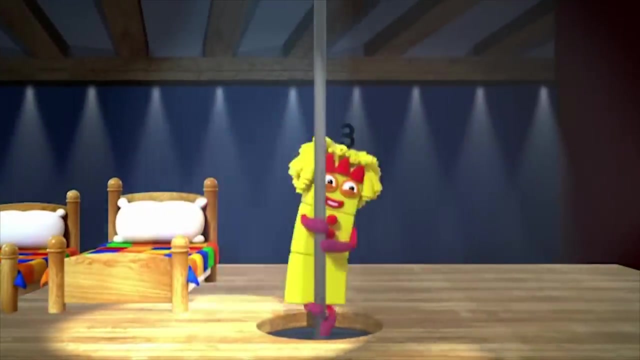 Three wishes would be nice. You should try and try and try again. That's my advice. Goldilocks came across three bears: One, two, three, Three balls, Three chairs, Three beds Upstairs. I'm here, I'm there. 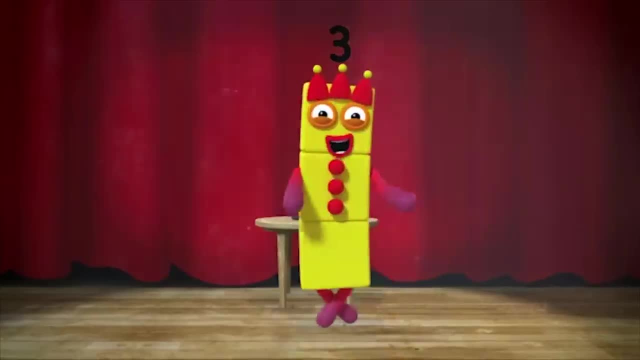 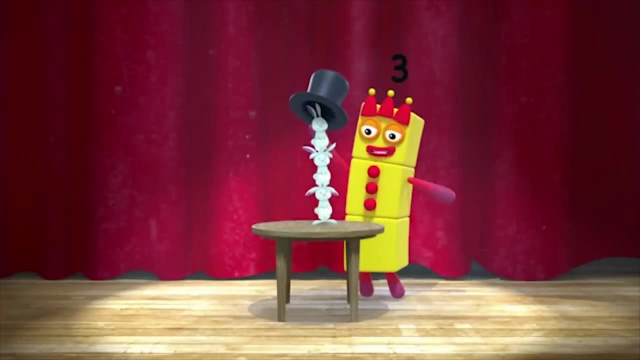 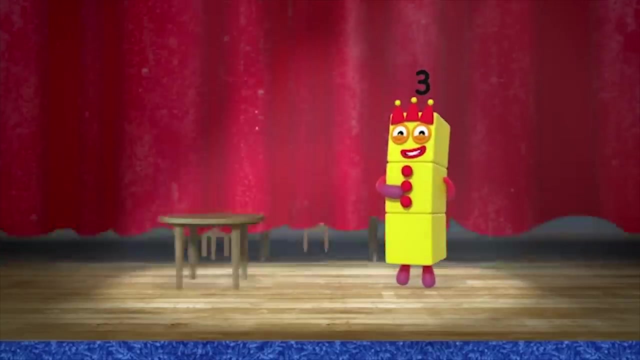 I'm everywhere. One, two, three, Everybody. look at me. I'm here to entertain you with this funky melody. I'll pull three rabbits from a hat and make them disappear. Everything's gonna be all right now. number three is here. 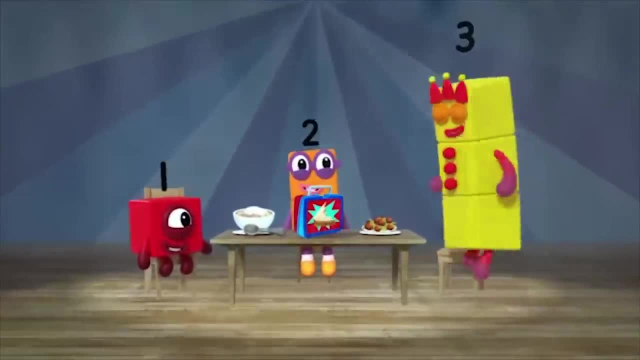 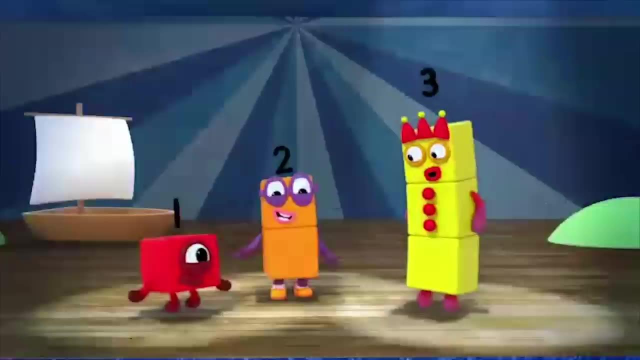 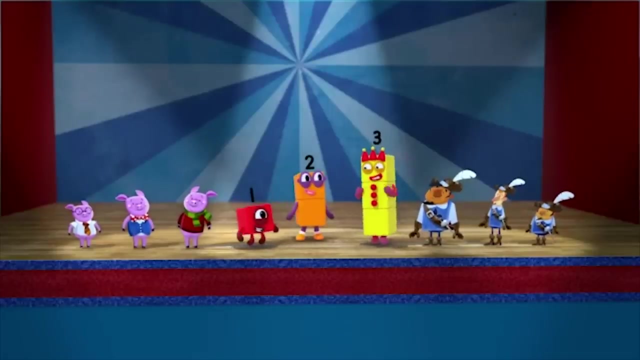 Three meals a day, Three sections in a play: Beginning, middle and an end. That's the only way. Everybody better give three cheers, Three little pigs, Three musketeers, One, two, three, Can't you see? 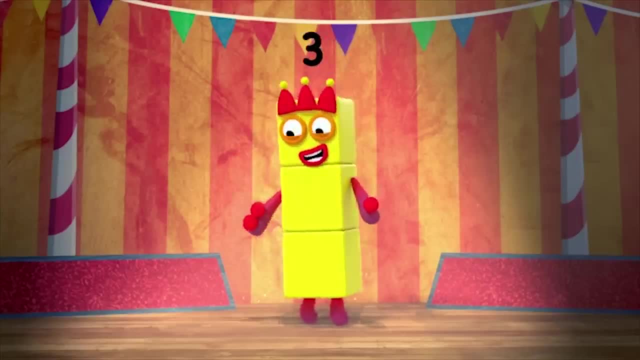 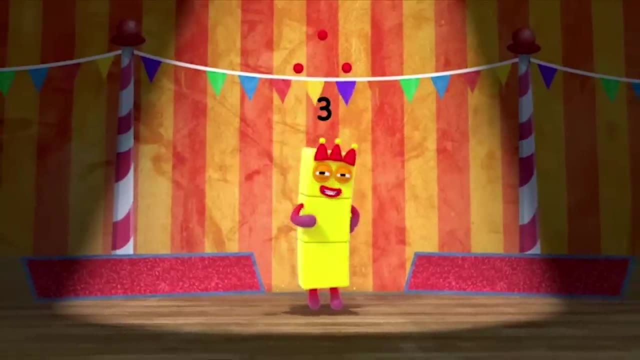 I can keep three balls up in the air: One, two, three. Sometimes they get stuck up there. One, two, three. The juggling balls can be your guides: One, two, three To make a shape that's got three sides. 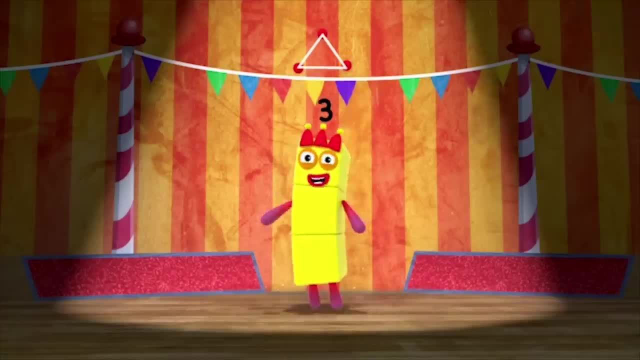 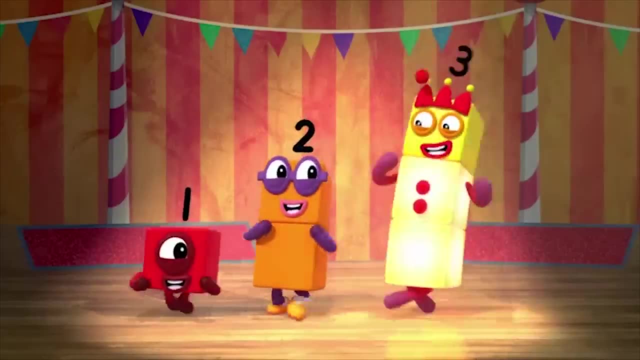 One, two, three. Do you know what it is Bingo? It's a triangle: One, two, three. Everybody, look at me. I'm here to entertain you with this funky melody. You can count on us with another box. 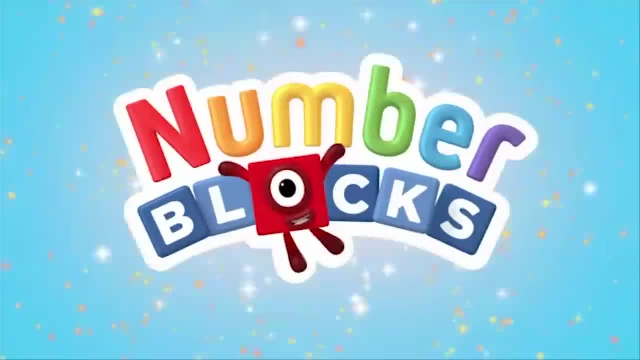 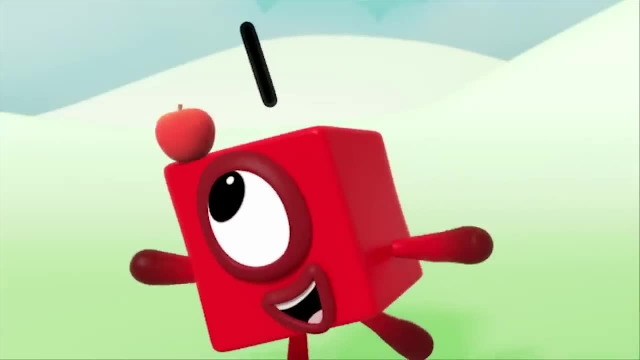 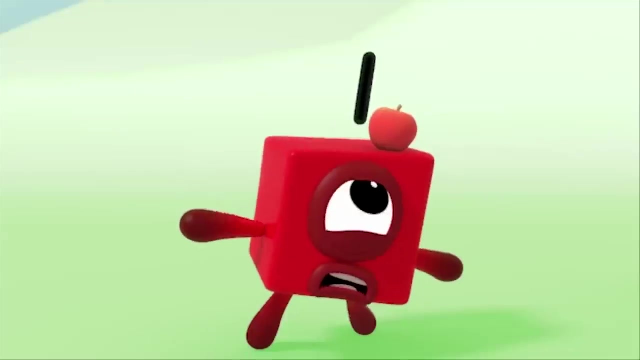 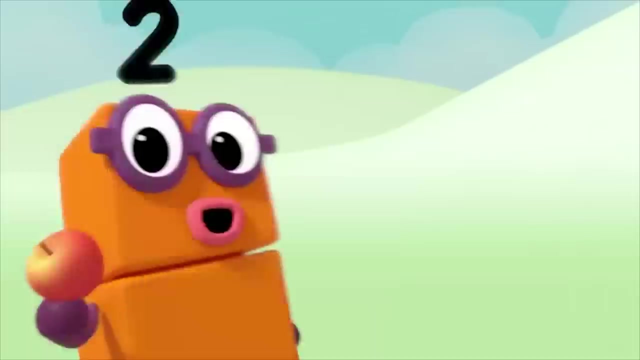 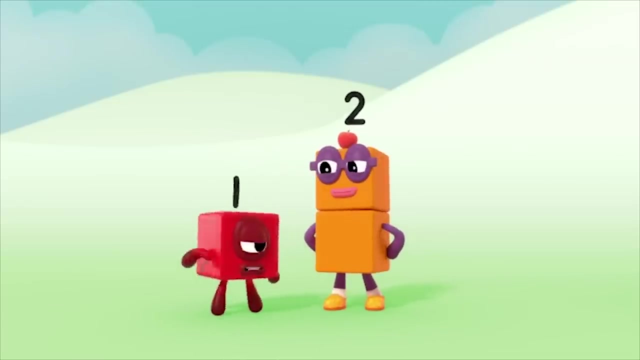 Let's play apple on top. Oh, Three simple rules: Apple on top, Don't let it drop. Now try and swap. Hey, Ah, Ah, Ah, Ah Ah Ah Ah. I can't reach. I'm smaller than you. 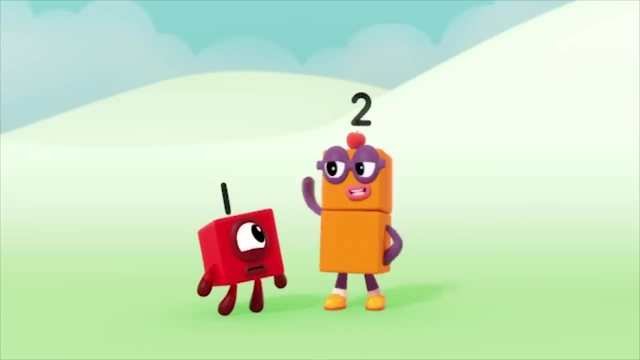 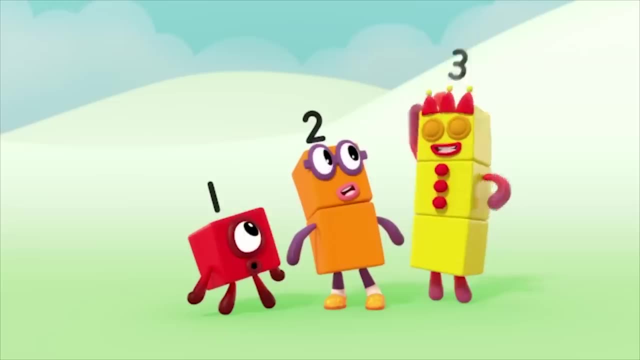 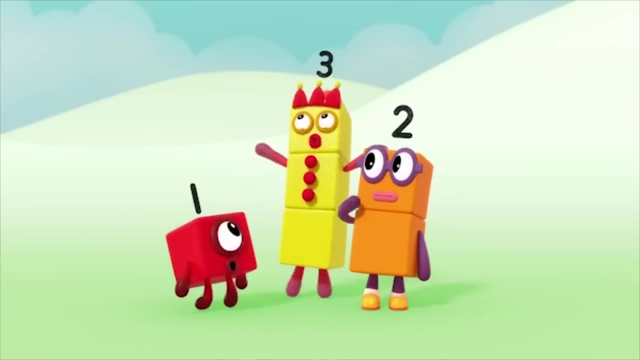 I'm the smallest number, Then I'm bound to win. I'm bigger than you- Oops, Silly me. I'm bigger than one, but smaller than three. I'm bigger than both of you. I'm the biggest, So I guess I win again. 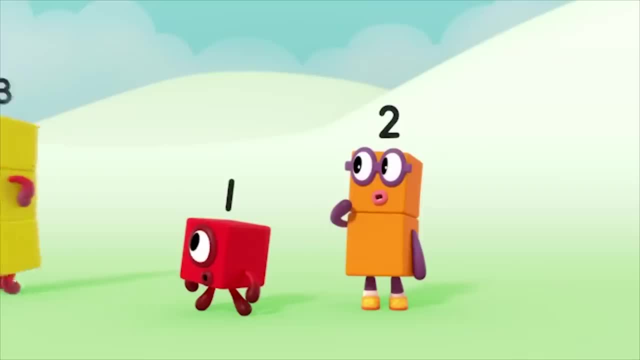 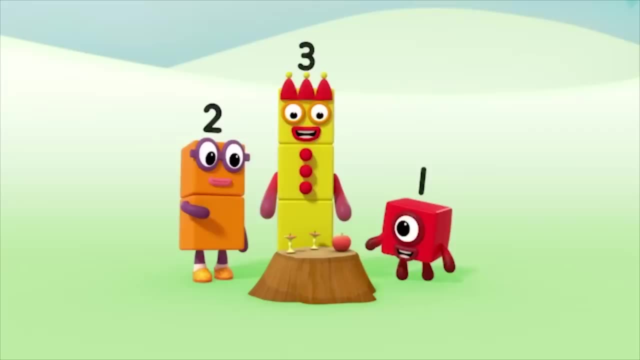 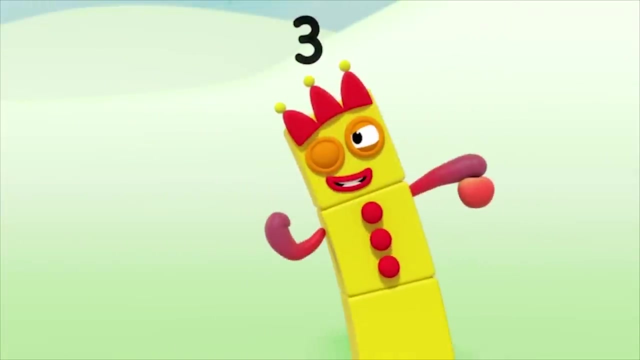 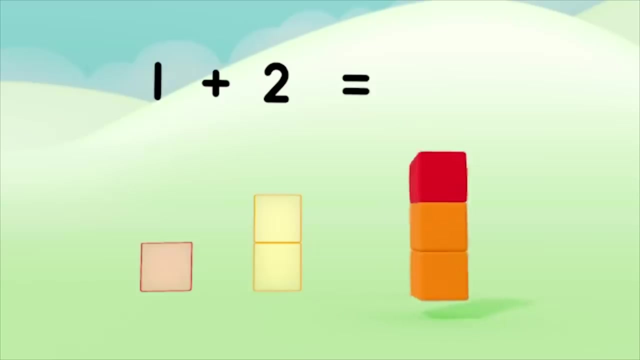 One, two, three, Two apples gone, One apple left. Surprise, It's the final game, The biggest surprise wins. One plus two equals three. One, two, three, Three equals Two plus one. Very good, You win best surprise. 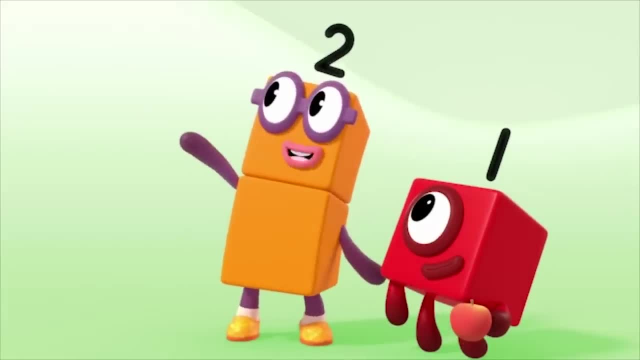 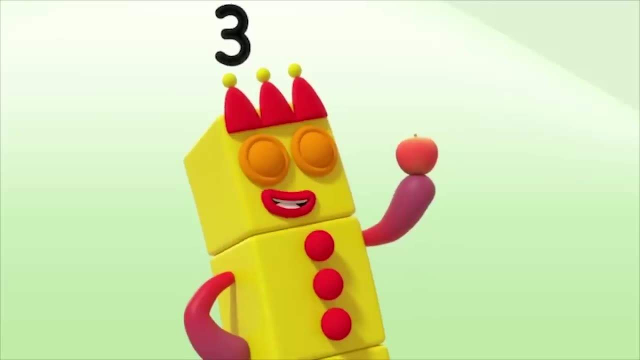 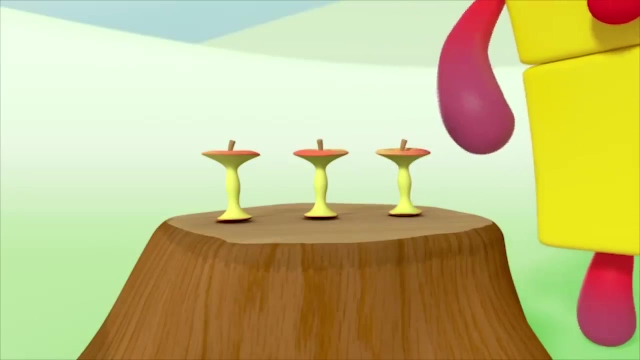 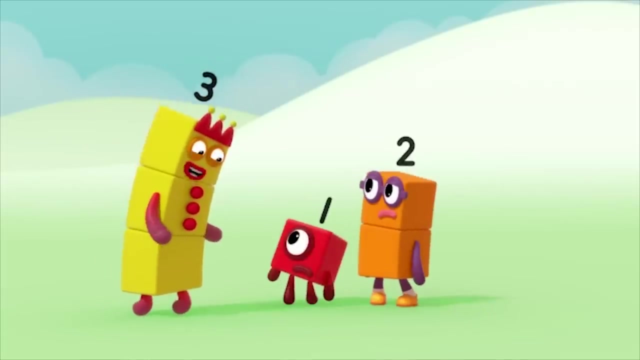 Three, One, two, three, All for me. Oh, that was the last one. Aww, Mmm. Oh, don't be sad, Don't be mad. I'm not mad. Don't be sad, Don't be mad. 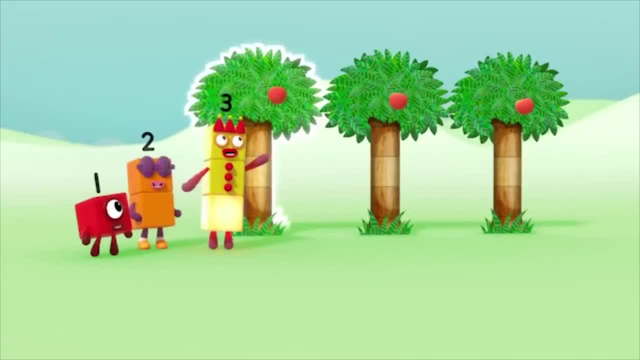 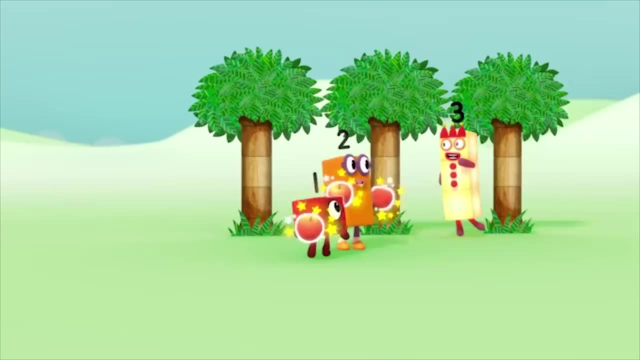 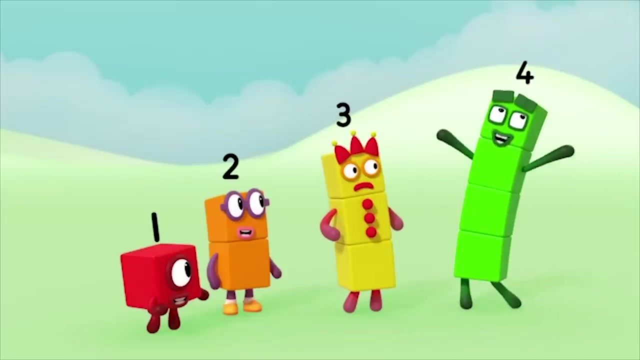 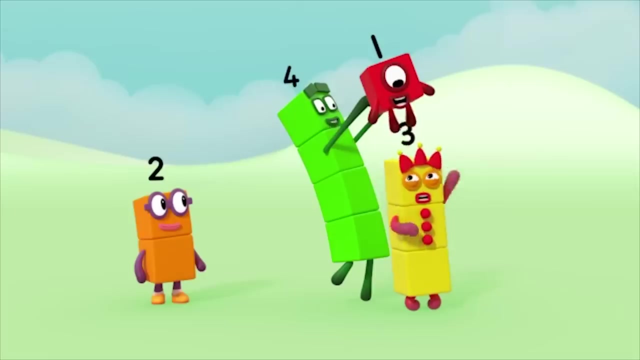 Be glad. One, two, three, Three trees With one, two, three, Three apples. You can count on us with an Outerbox. I'm four. Have you met me before? I'm one, more than three, Ooh. 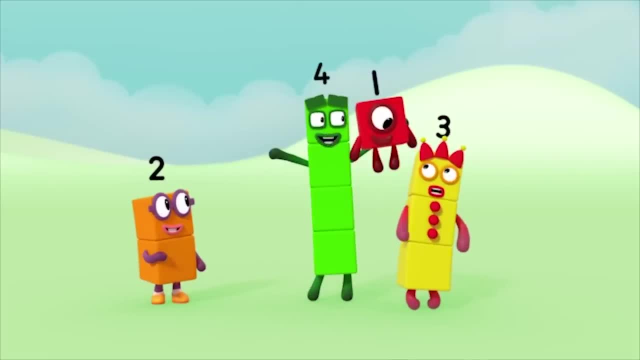 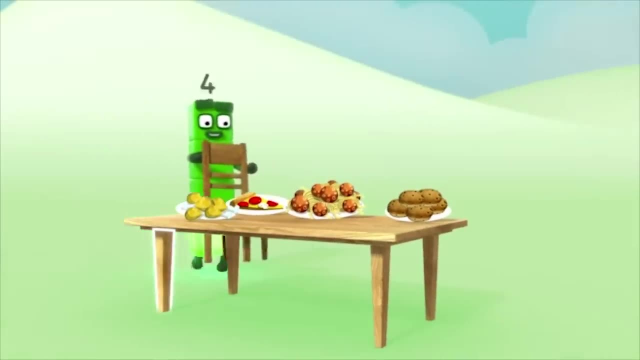 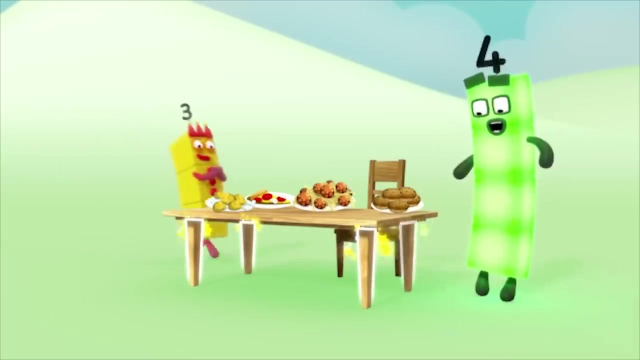 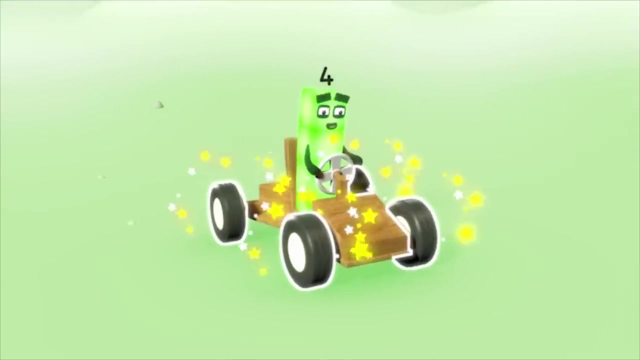 It's a shame to see Three plus one equals me. I'm four. One, two, three, four, Four legs on a table. One, two, three, four, Four legs make the table more stable. Oh, One, two, three, four. 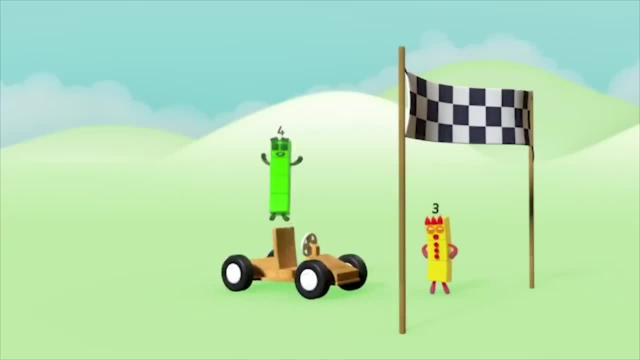 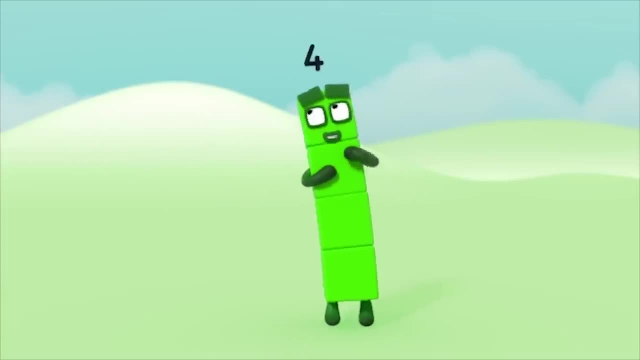 Four wheels on a go-kart. Without four wheels, you know go-go-kart, We'll be stuck right back at the start. I'm four. Have you met me before? I'm one, more than three. That's when to see. 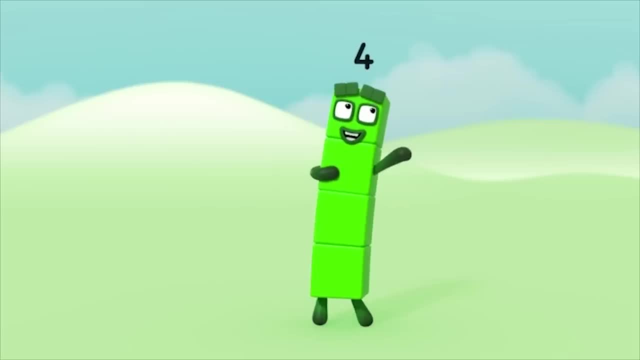 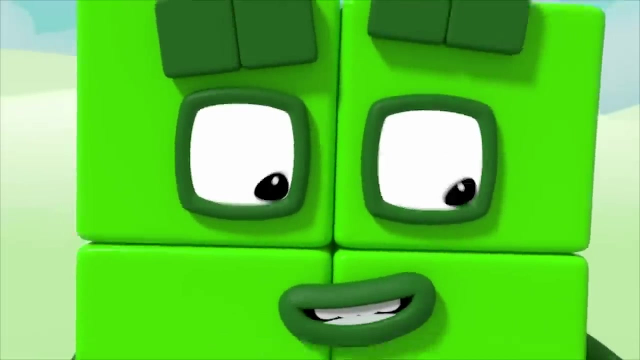 Three plus one equals me. I'm four. I can be thin and tall, I can be low and long, I can be shaped Like the letter L, But the best shape of all is stout and strong. What shape is this, Can you tell? 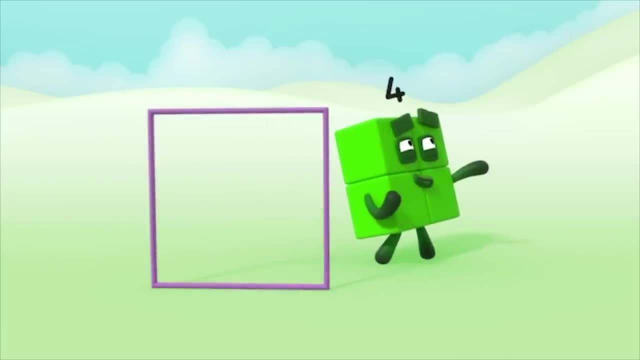 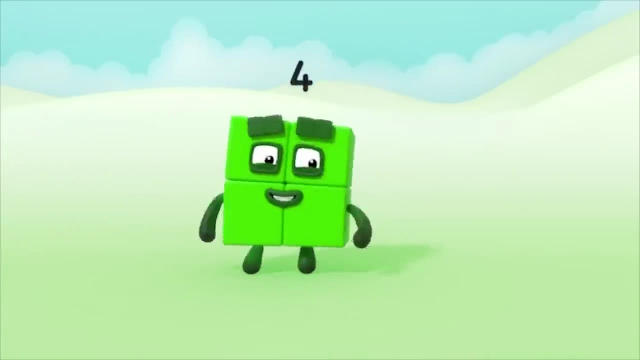 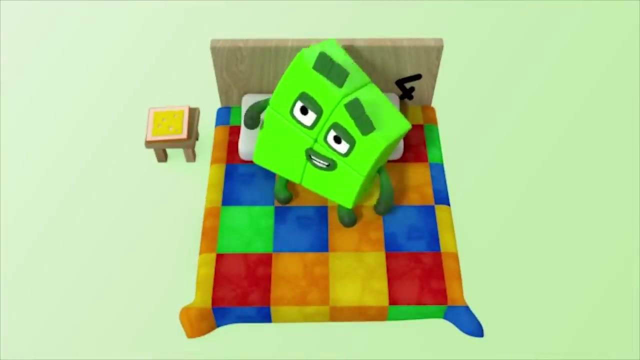 I like to be square. I like to see square things everywhere. Anywhere there's a square, you'll find me right there. Square cheese on square bread, Square quill on a square bed. Square is where it's at. of that you can be sure. 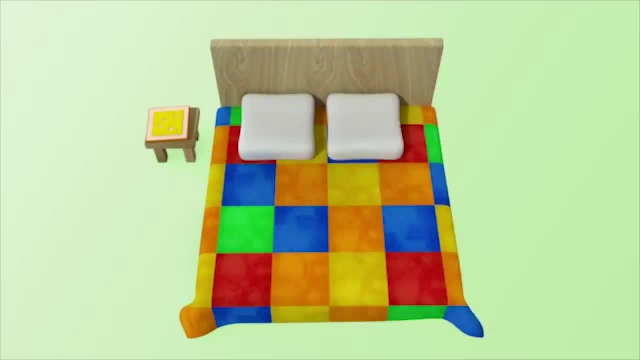 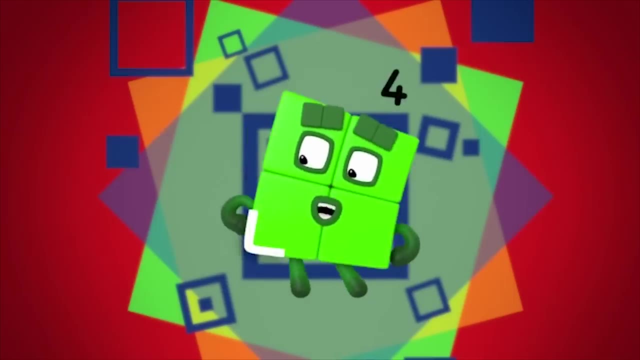 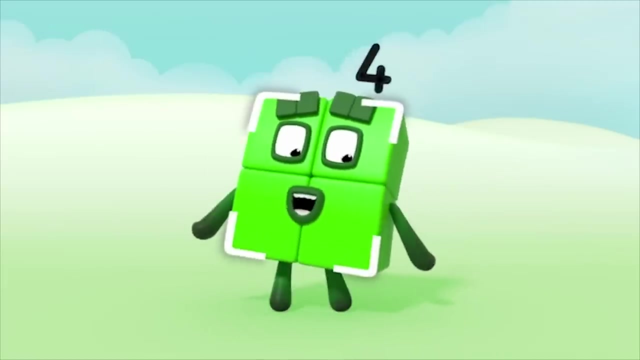 Anywhere there's a square, you'll find more: One, two, three, four, Four sides. One, two, three, four, Four corners. Square is the shape for me. It has four corners and four sides, you see. 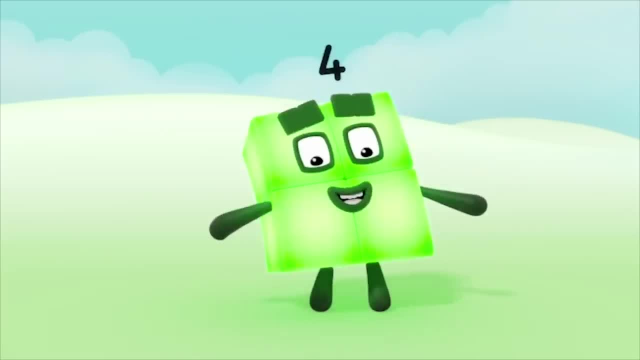 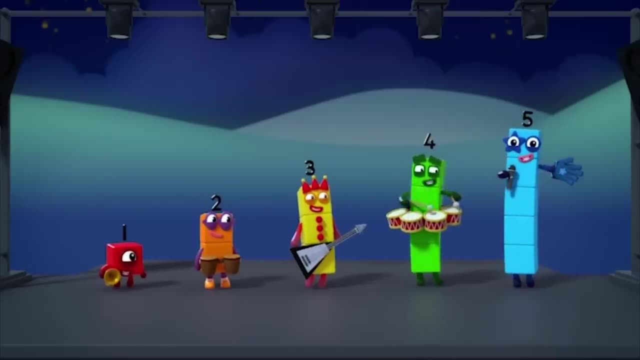 When four blocks make one big block, I'm solid as a rock. You can count on us with an autobox. Five members in my band: One, two, three, four, five. Five fingers on one hand: One, two, three, four, five. 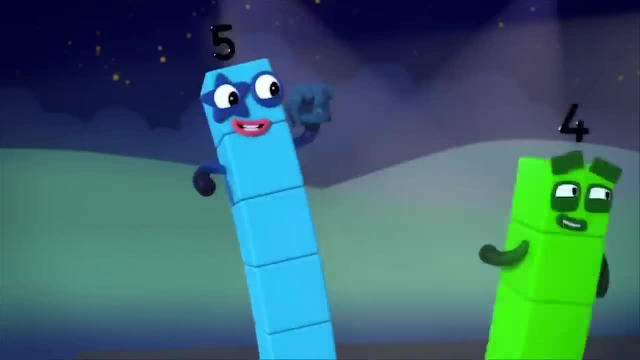 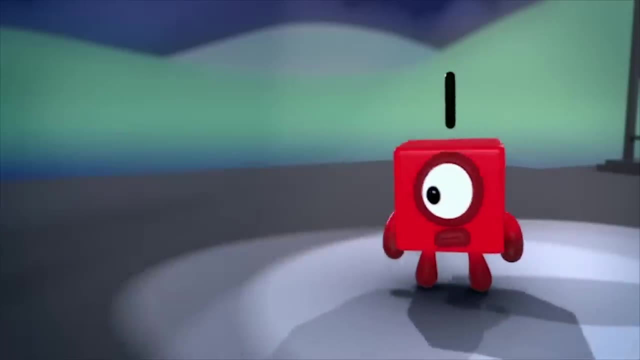 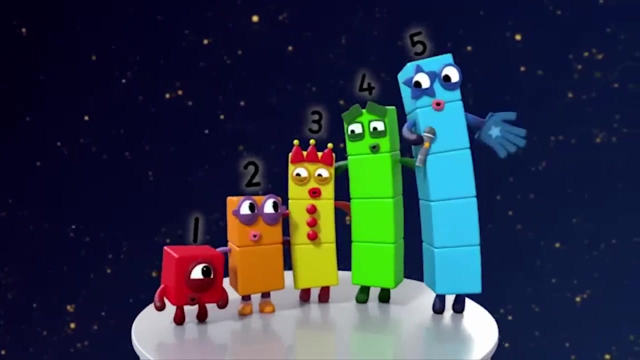 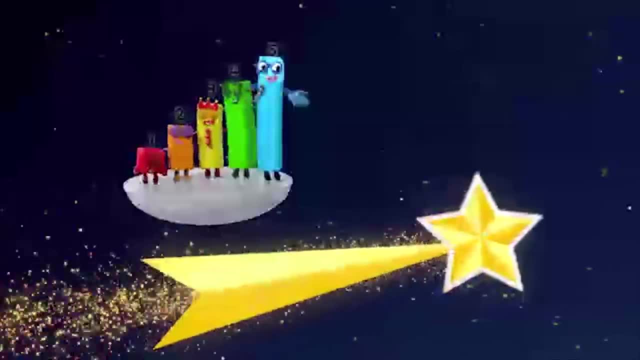 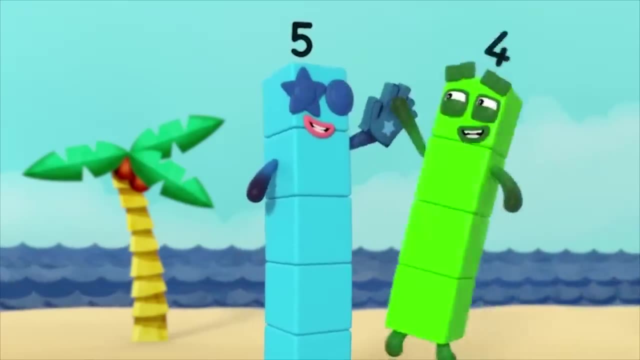 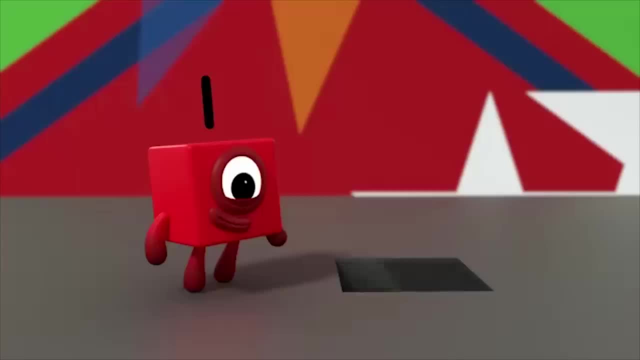 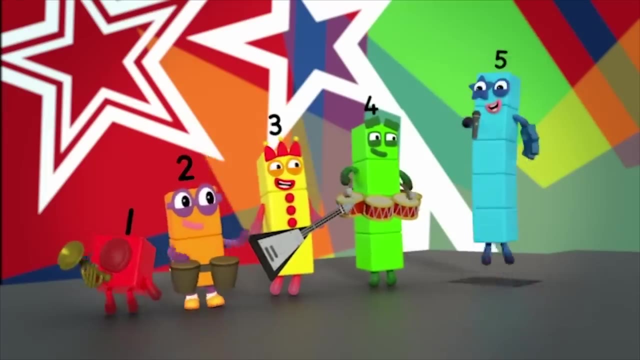 High five, High five To the side, up above, down low, too slow. High five, Ooh, I feel so alive. You know that you've arrived when you're with number five. Five fish fingers on a plate: One, two, three, four, five. 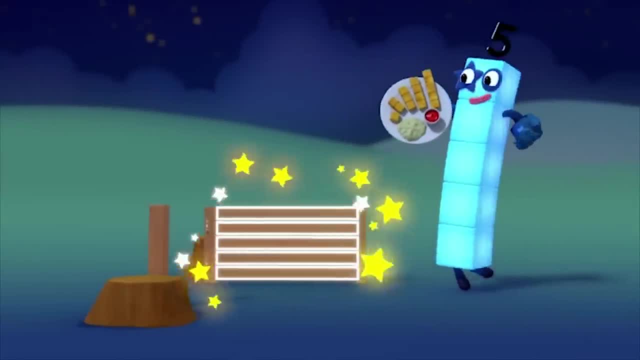 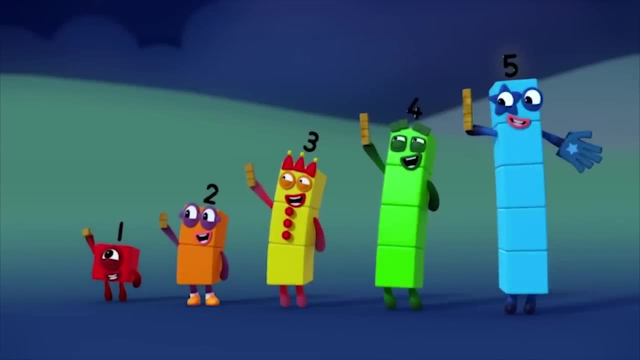 Five bars on a five-bar gate: One, two, three, four, five, I'm five. Ooh, I feel so alive. You know that you've arrived when you're with number five, I'm number five, and I hope you understand. 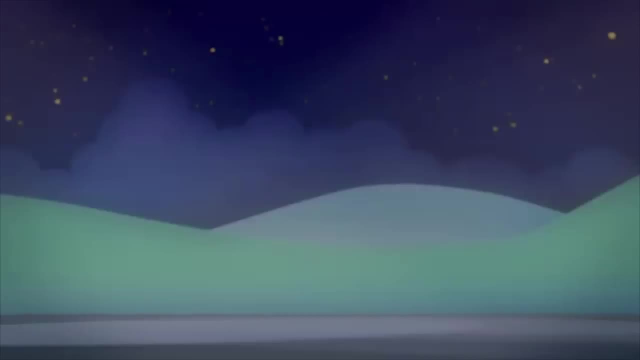 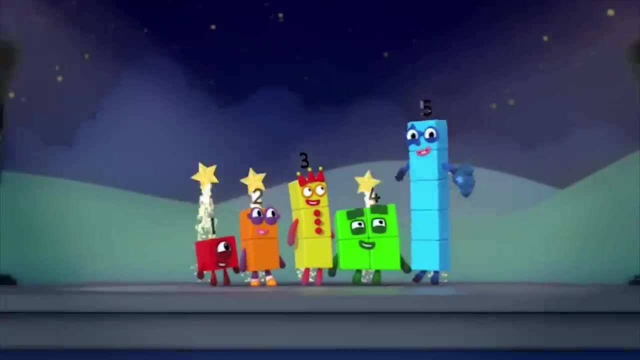 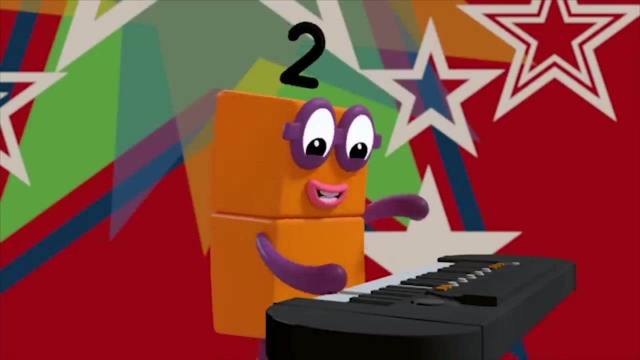 Whenever you need help, I'll be there to lend a hand. Now the band is all together. the rest can join the queue. We'll be five stars forever and there's nothing we can't do. Five questions on our lips: Who, what, when, where, why? 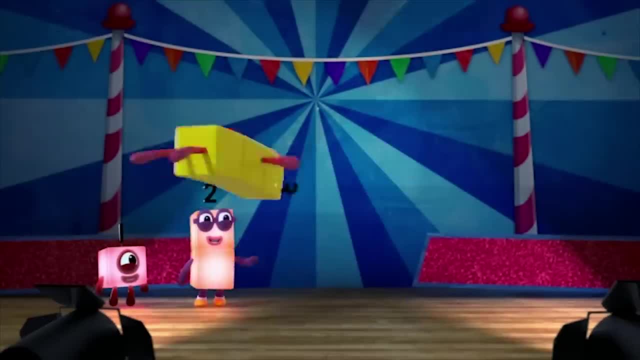 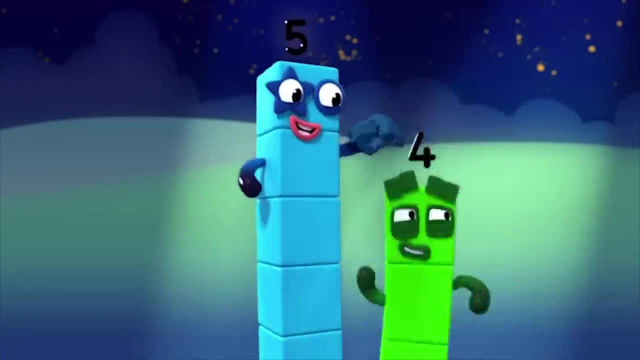 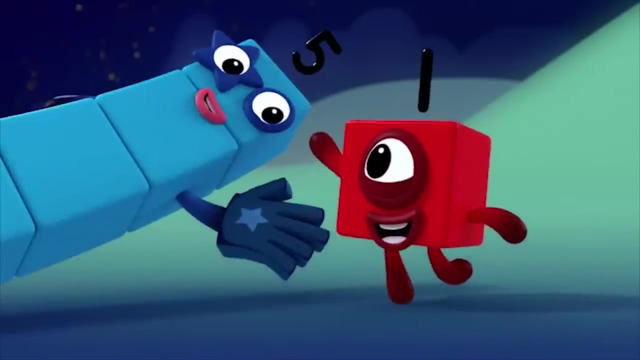 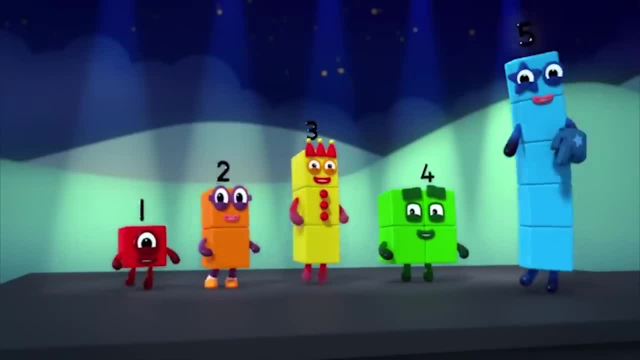 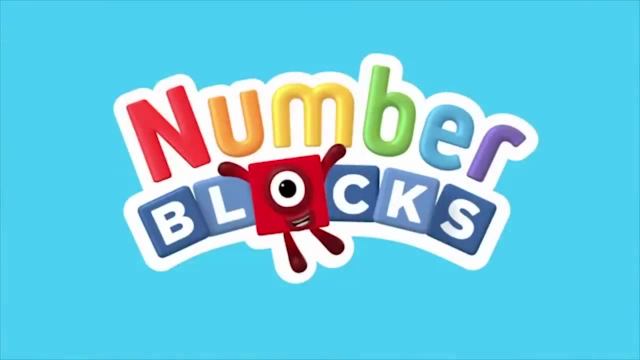 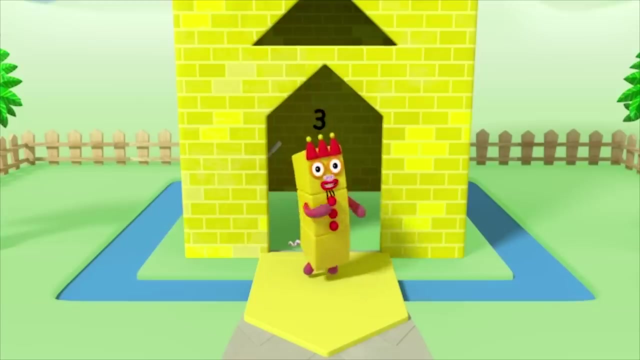 High five. Ooh, I feel so alive. You know that you've arrived. when you're with number five, You can count on us. we're the number five. But where will we live now? Luckily, the third little pig. Oh, that's me. 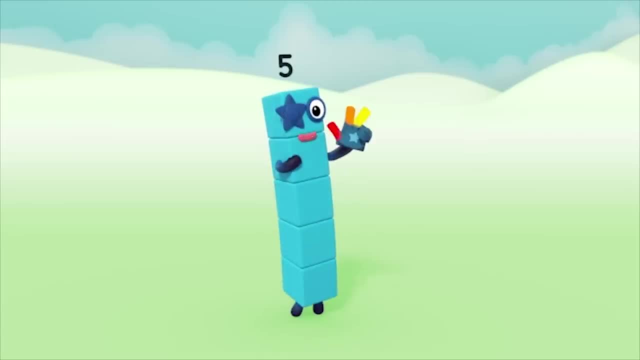 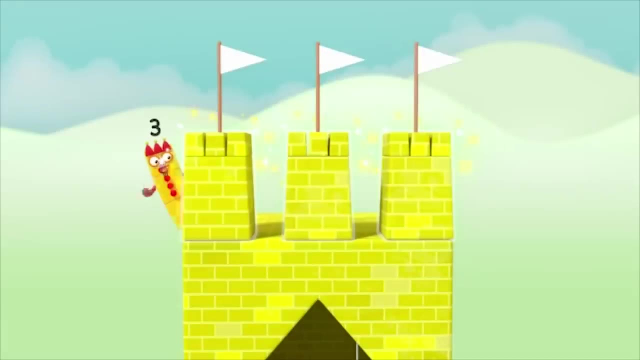 Busy, busy, busy. had a house with three rooms And one, two, three, three windows And one, two, three, three turrets And one, two, three, three flags. And yes, yes, thank you. 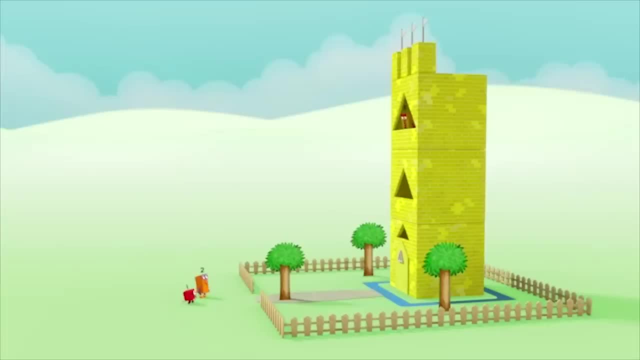 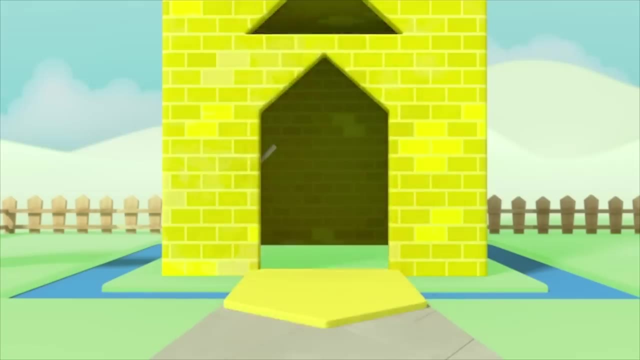 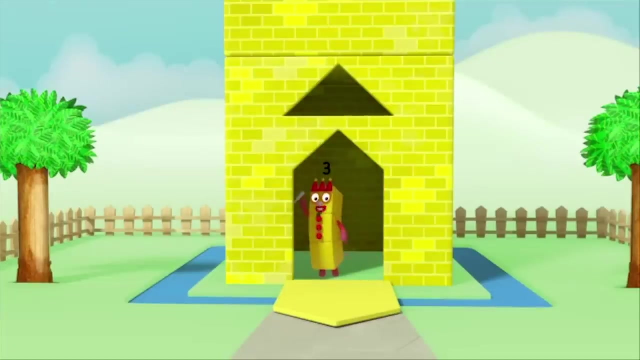 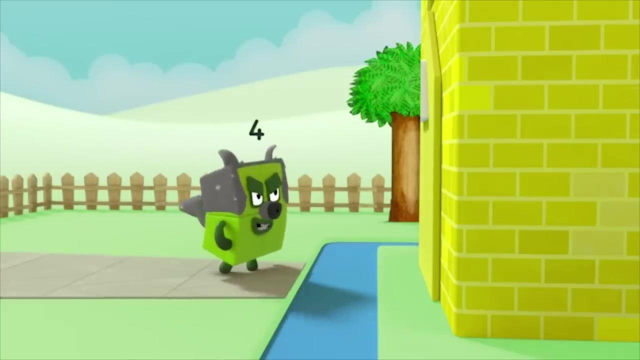 And one, two, three. Room for a couple more. Sure, Two's company and three's a party. Keeping that big bad square out is as easy as one, two, three. Little pig, little pig, Let me in. 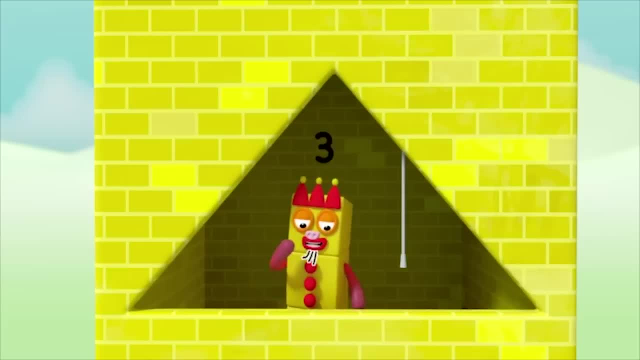 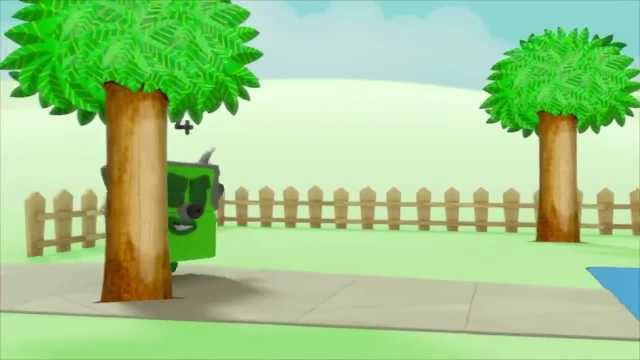 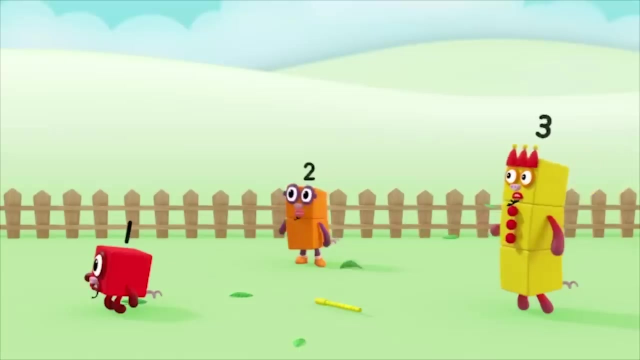 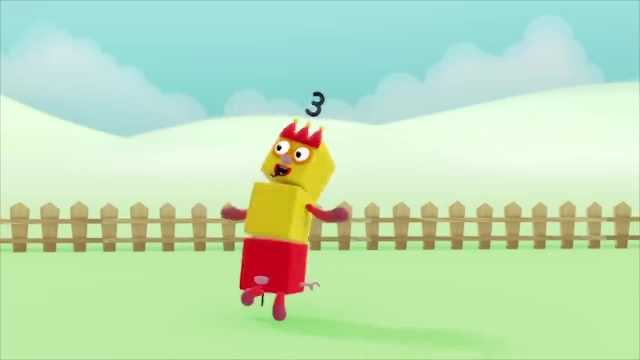 Let me in, Not by the Three hairs on my chinny-chin-chin, Then I'll huff and I'll puff and I'll blow your house in What But how? Just a little huff, Hey. 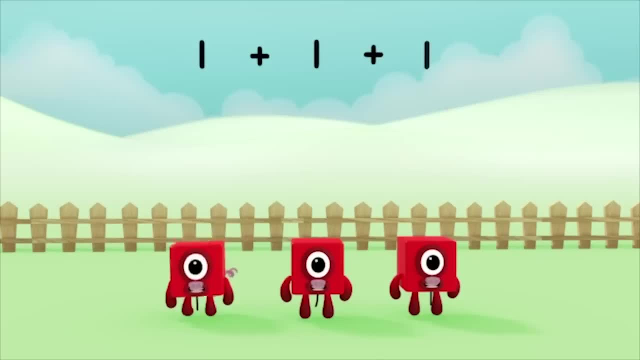 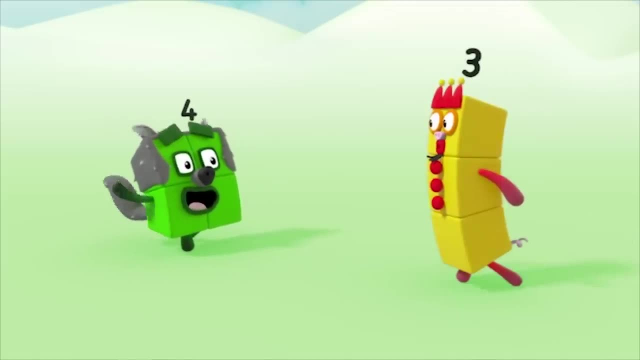 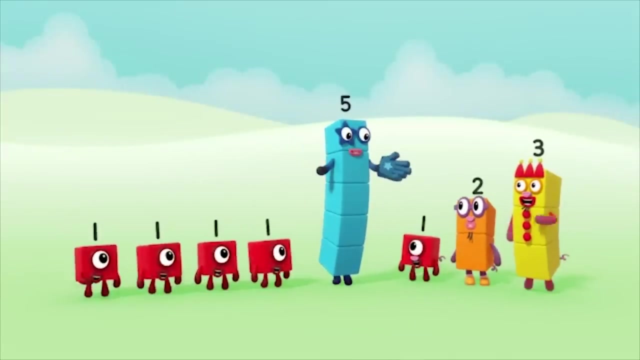 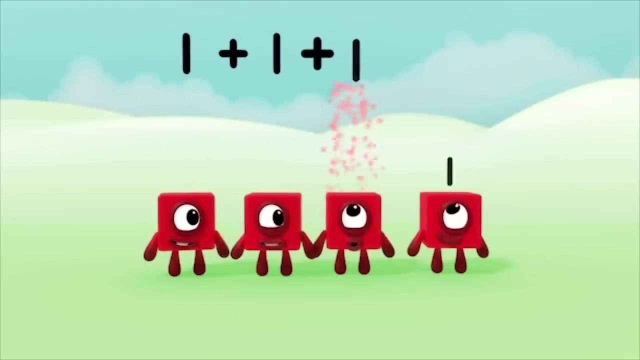 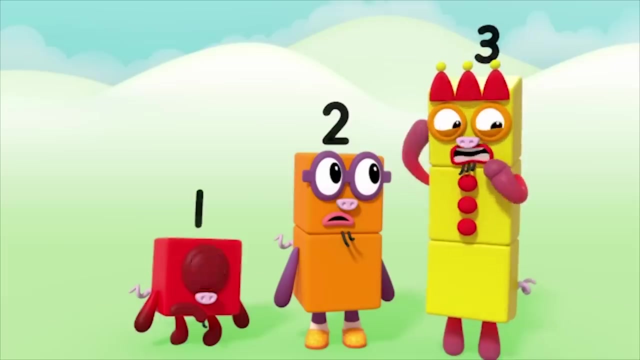 One plus one plus one equals three. See how you like it. Stop. This isn't how the story goes. The third house doesn't get blown down. Oh, One plus one plus one plus one equals four. Where will the three little pigs live now? 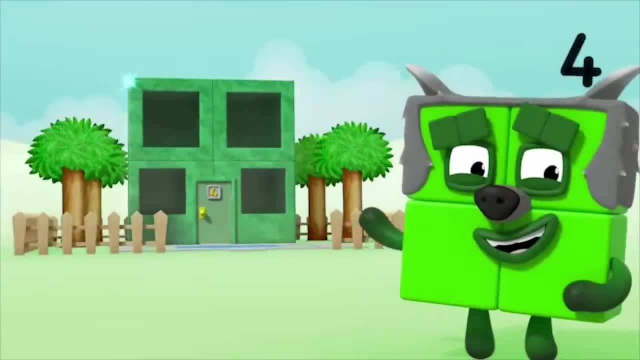 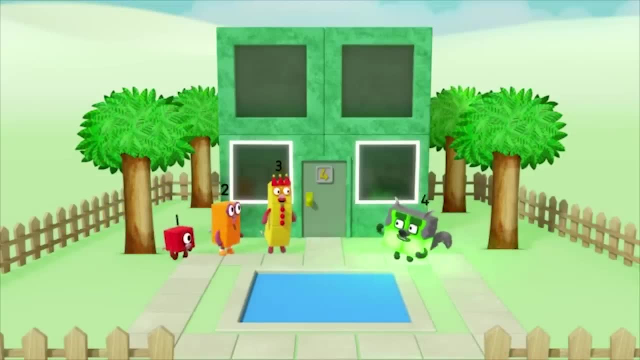 Oh, Where will the three little pigs live now? Where will the three little pigs live now? Oh, Where will the three little pigs live now? There's always my house. It's got four rooms, with one, two, three, four. 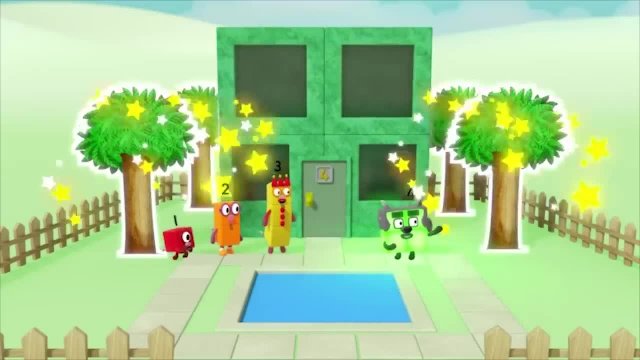 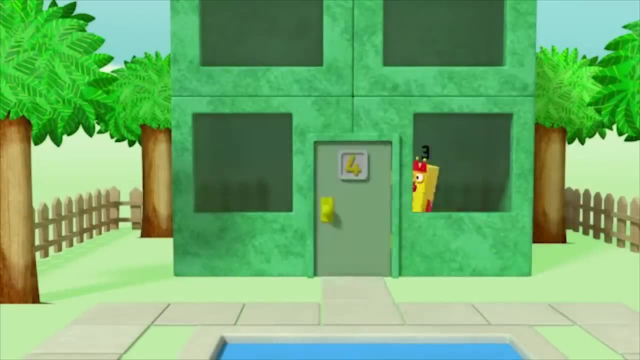 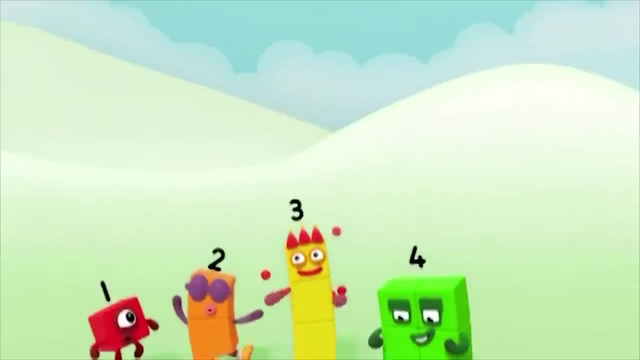 Four windows and one, two, three, four, Four, threes and a number four on the door. One, two, three, four. You can count on us with a number box, Knock, knock, knock. One, two, three, four. one, two. 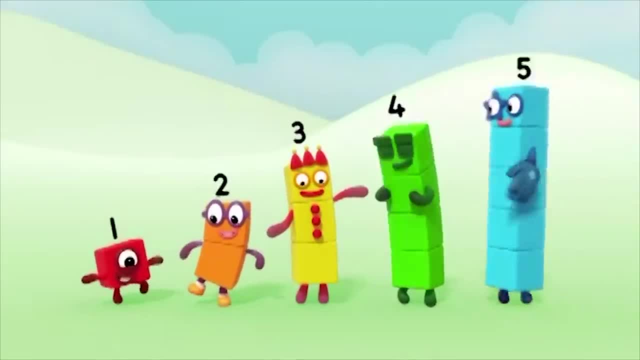 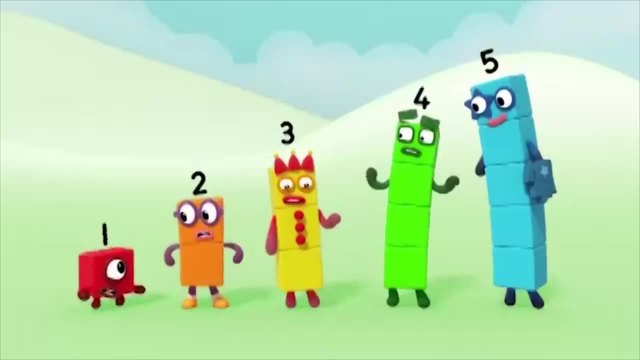 Come back. come back, I got a number. I can do my exercises. What now? Pop, two, three, I can do my exercises. Hi, team, High five. So are we all here? Well, how can we tell? 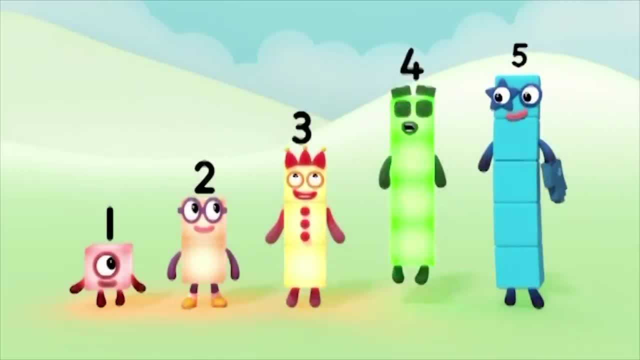 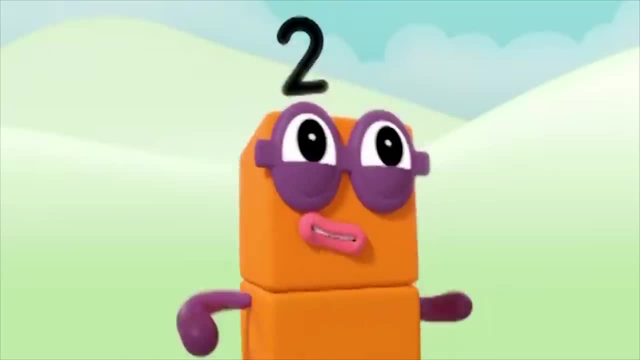 I know just the thing: Ready, steady, sing One, two, three, four, five. That sounds right. That sounds right. What shall we do today? Run through the forest, Climb to the top of a tree, Pretend to be pirates. 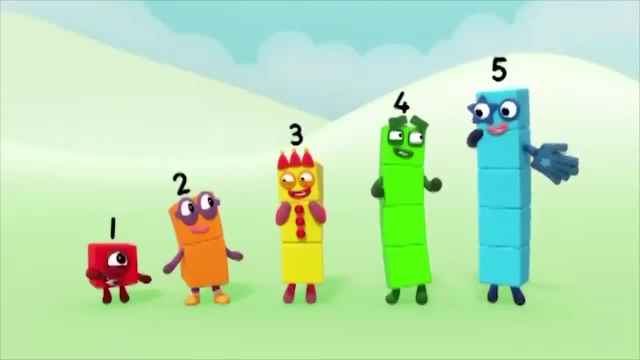 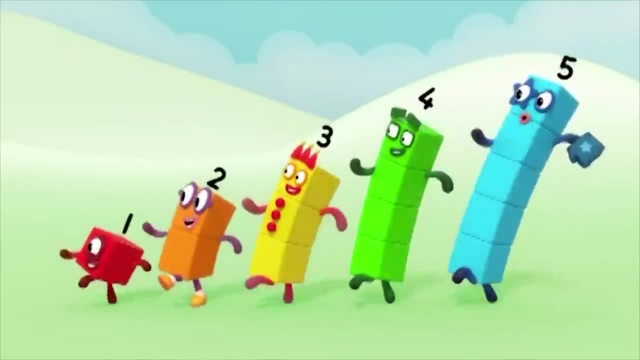 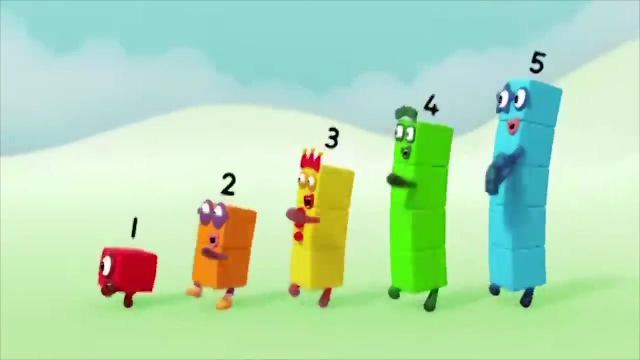 Discover a whole new world. Let's have an adventure. Hooray, Everybody ready, Off we go, Off, we go on a big adventure. We don't know what the day will bring. Off we go on a big adventure. Ready, steady, sing. 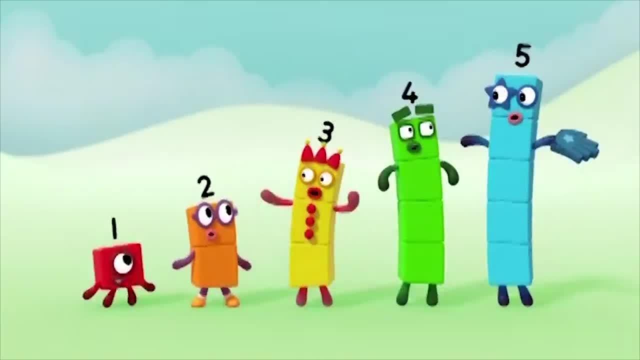 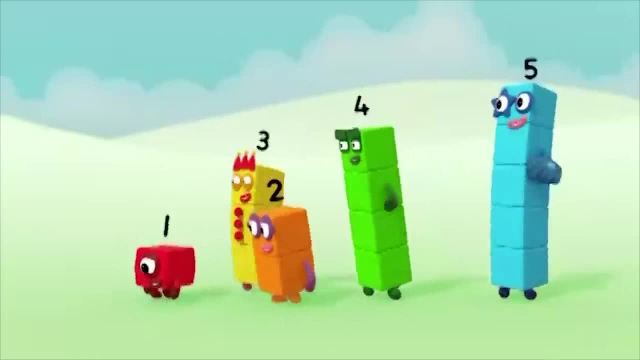 One, two, three, four, five. That sounds right. And off we go again. Off we go on a big adventure, We don't know what the day will bring. Off we go walking in the sunshine, Ready, steady, sing. Wait Too short, Can't see. 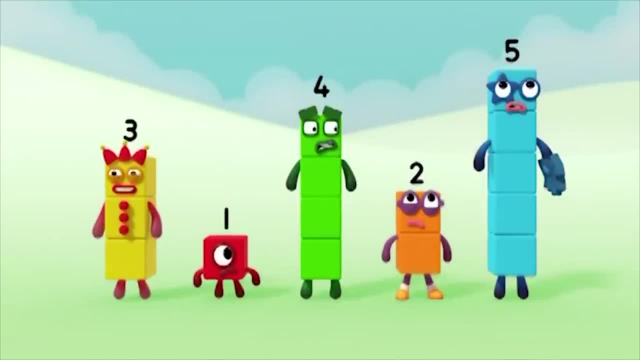 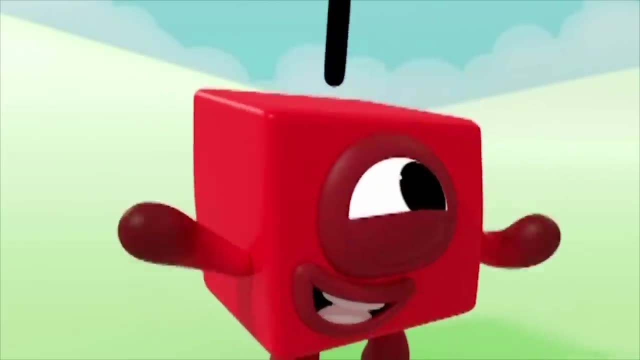 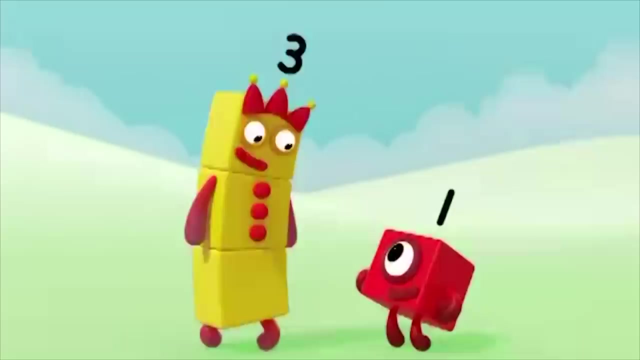 Three, one, four, five. That doesn't sound right. We're in the wrong order. I know what to do. Diddly, diddly do. Smallest that way, Biggest that way, This way Go, I'm bigger than you. 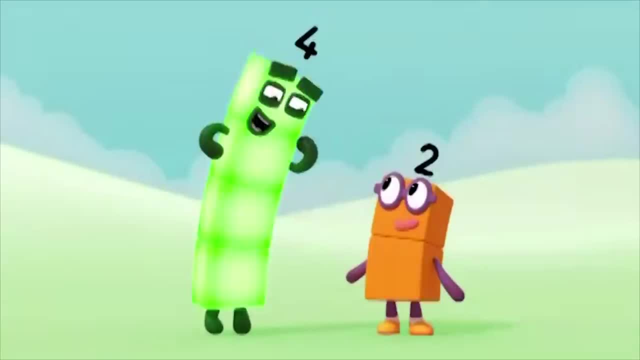 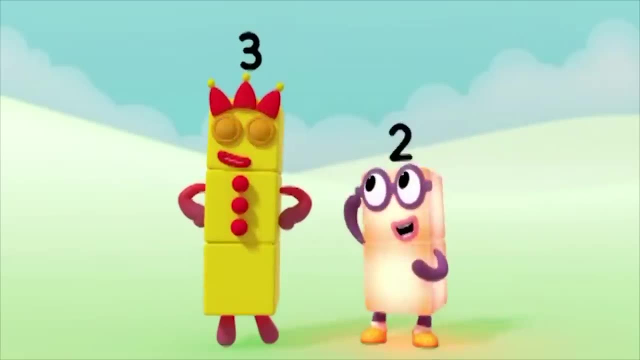 I'm smaller than you Diddly diddly do. I'm bigger than you. I'm smaller than you Diddly diddly do. I'm bigger than you. I'm smaller than you Diddly diddly do. 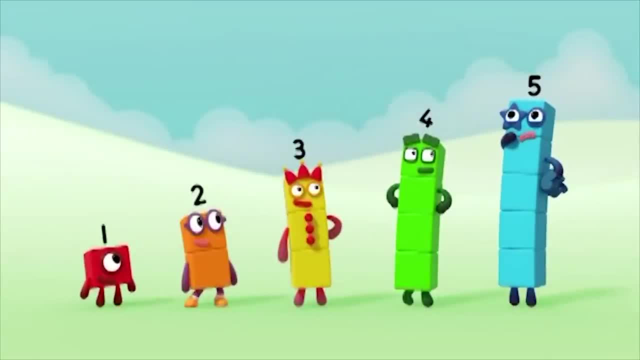 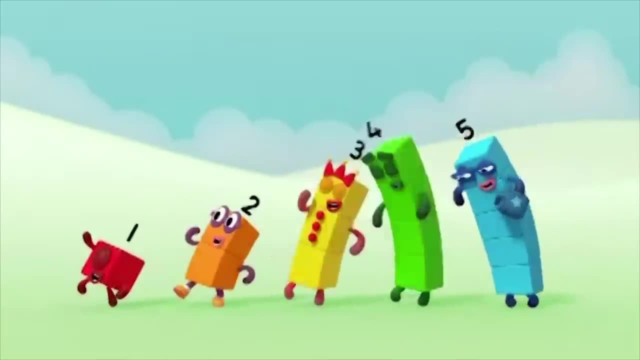 Are we all in order? Did we all do the right thing? Ready, steady, sing One, two, three, four, five. That sounds right. And off we go again, Off we go on a big adventure. We don't know what the day will bring. 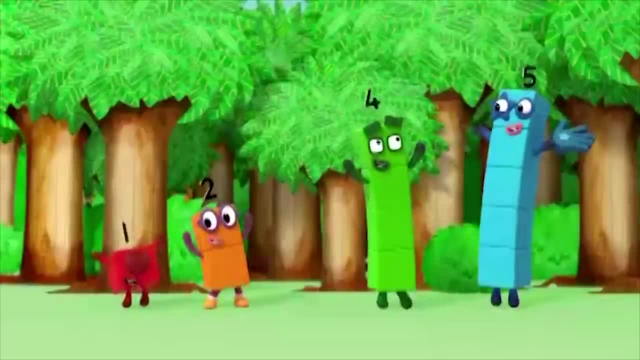 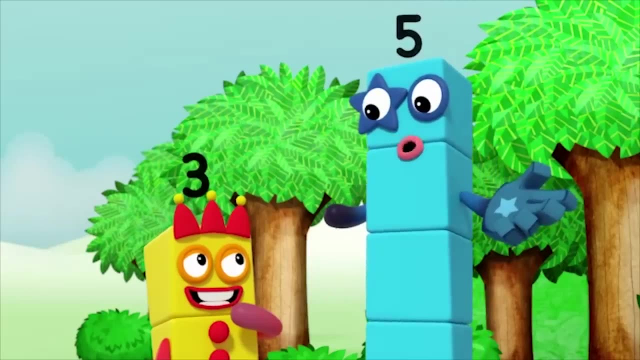 Off we go, running through the forest, Ready, steady, sing. You can count on us with an autobox Three. do you know how to count? Yes, of course. Look at a bunch of things, say some numbers and then say three. 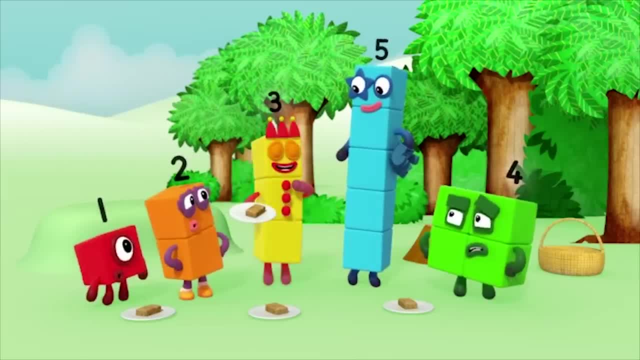 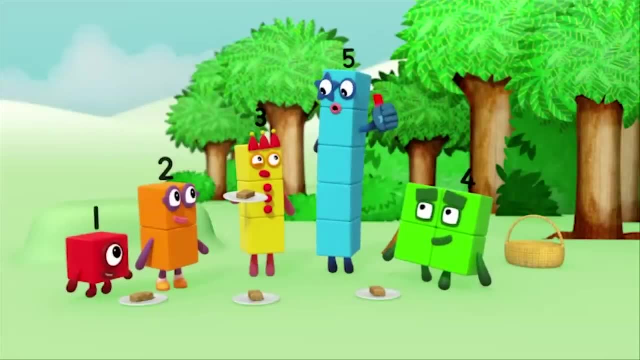 Because three's the best number. There's a little more to it than that three. There are some rules you have to follow. Rule one: count everything once. Try counting those flapjacks. It can help to put them in a line. 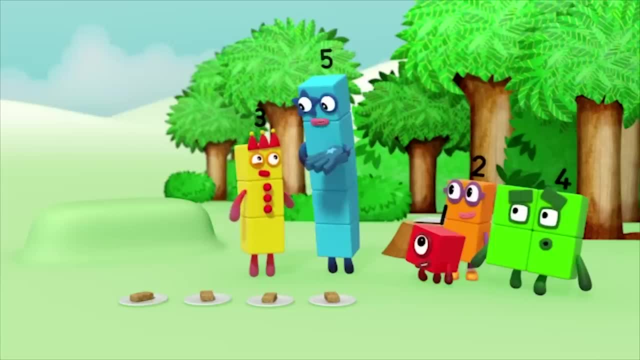 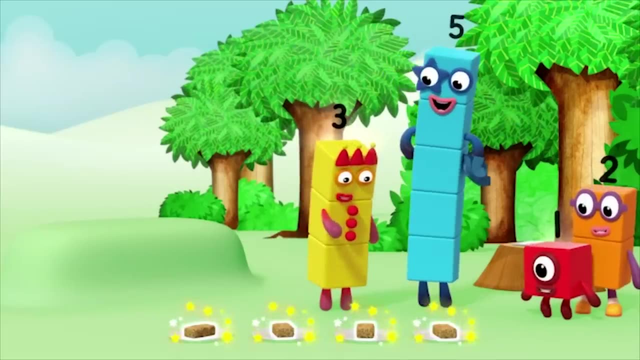 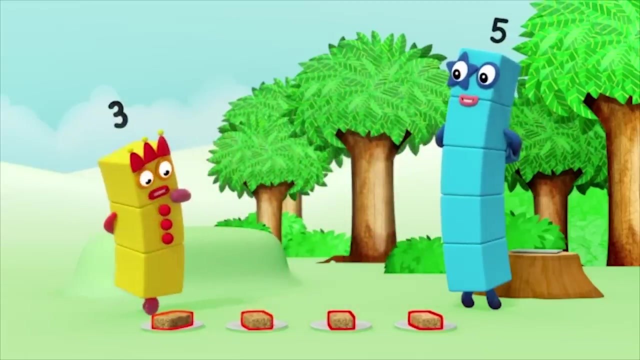 and to point at them one at a time, to make sure you don't miss any Or count the same one twice. One, two, three, four. Very good, Four, three, two, one, Wait one. That's not right. 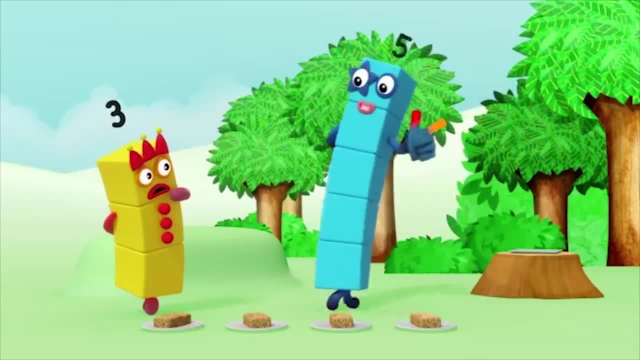 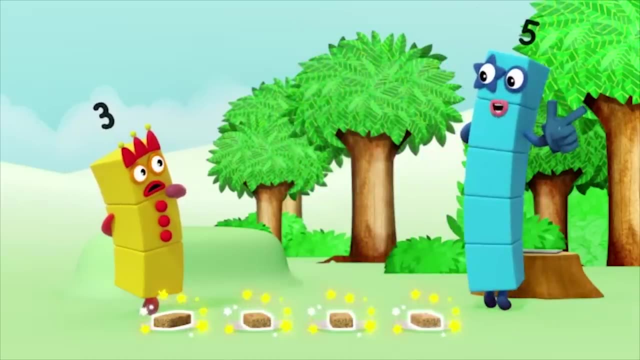 Rule two: Say the number again, The number's in the right order. If you don't say them in the right order- one, two, three, four- you won't know how many there are. Oh, One, two, three, four. 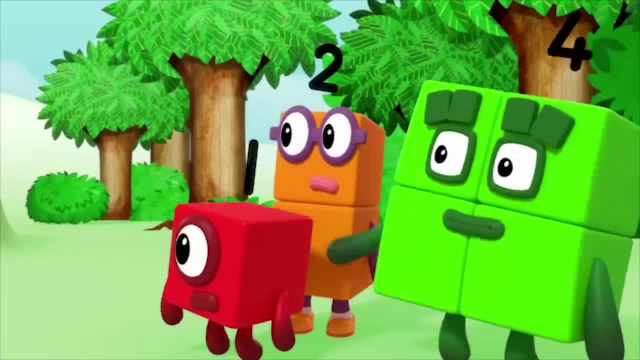 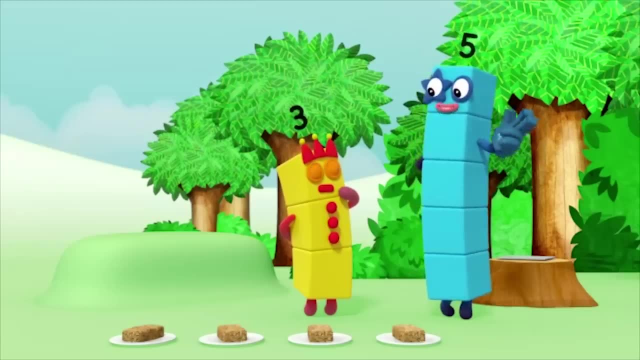 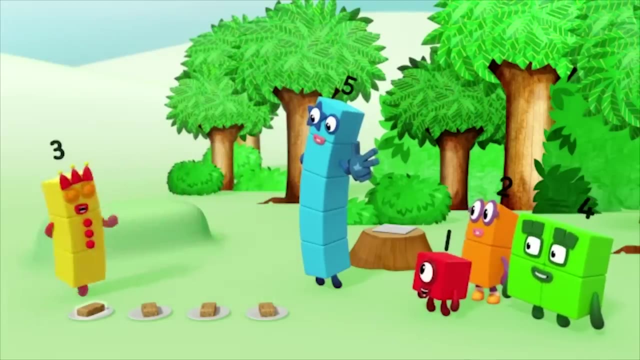 Three flapjacks. Oh, we've been here before. Rule three: The last number is how many. When you reach the last thing to count, the last number you say tells you how many there are. Try, You can do this, Go on. 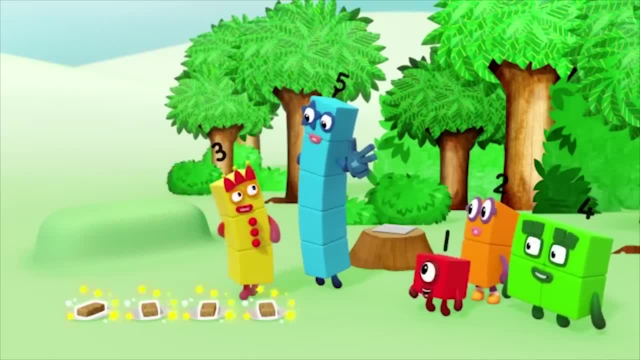 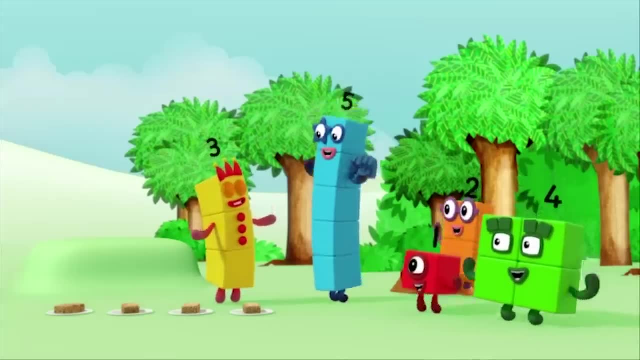 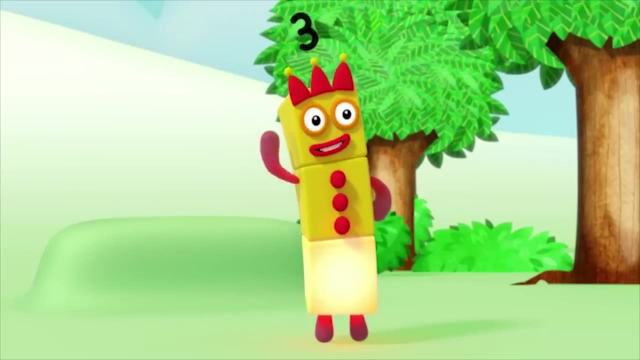 One, two, three, four. That's the last flapjack. So four flapjacks, That's right. Yeah, I did it. I know how to count. One count everything once. Two say the numbers in the right order. 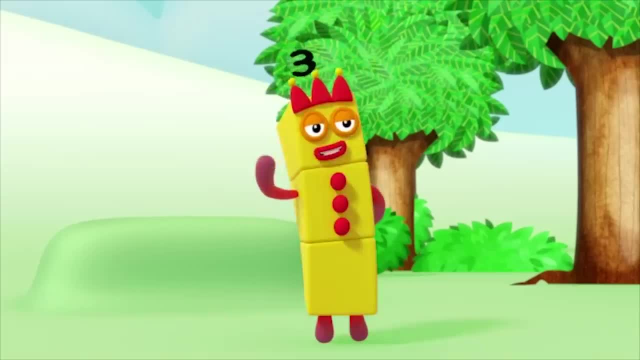 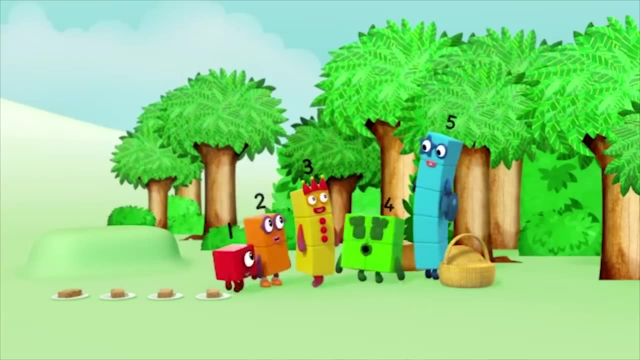 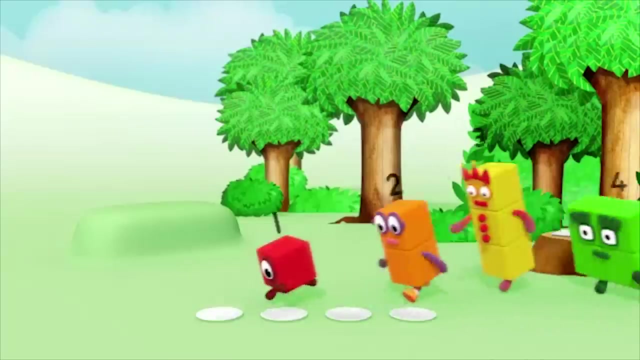 Three. the last number is how many? Three rules of counting. All right, Let's celebrate with flapjacks. I've packed an extra one for you: five. Hang on, It's gone. Oh, Oh, Oh, Oh Oh. 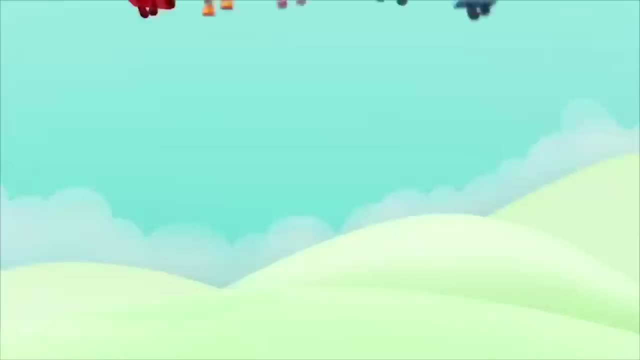 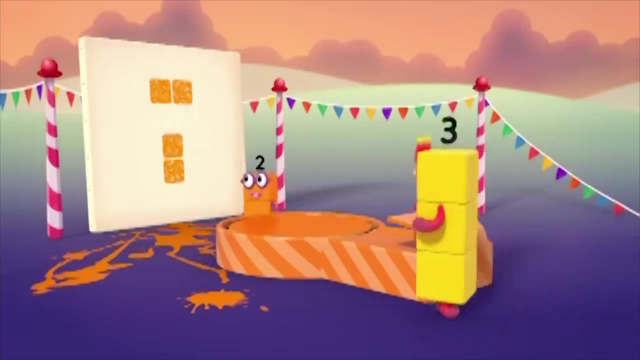 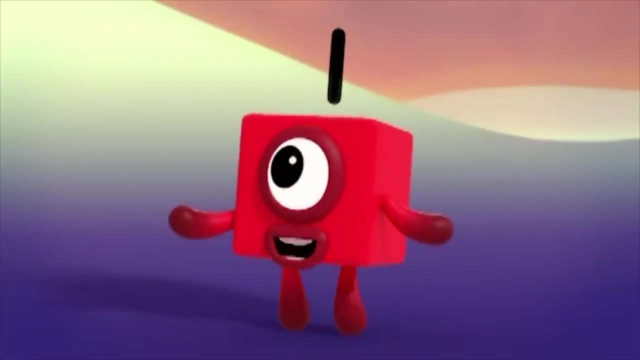 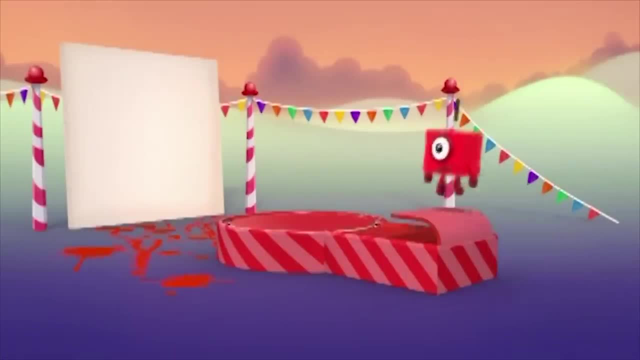 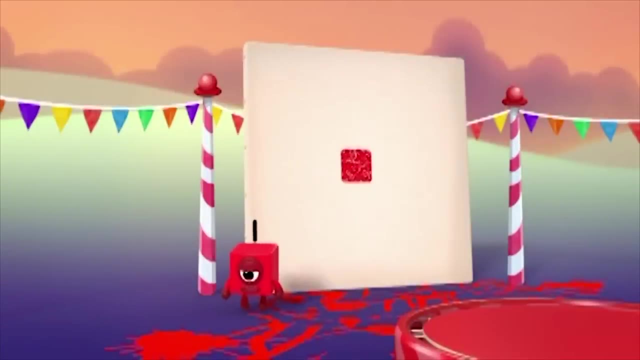 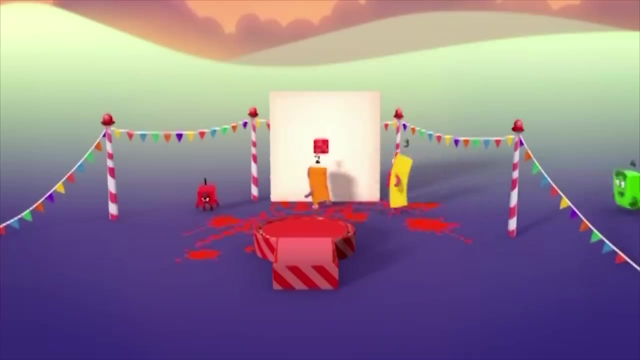 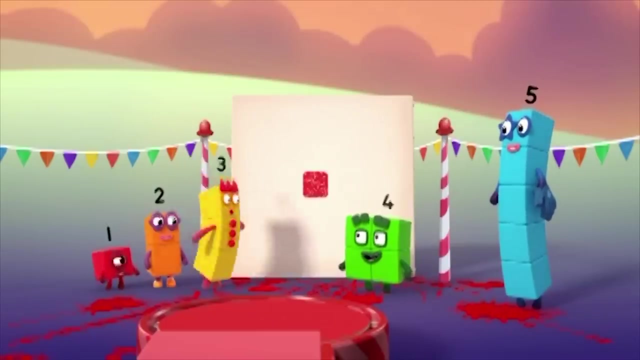 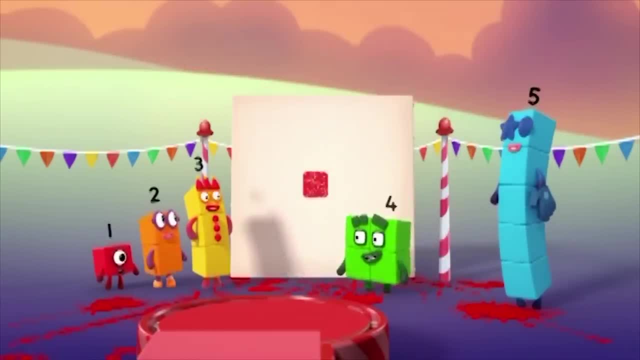 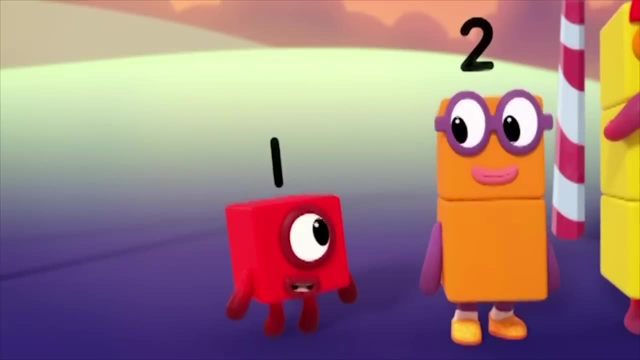 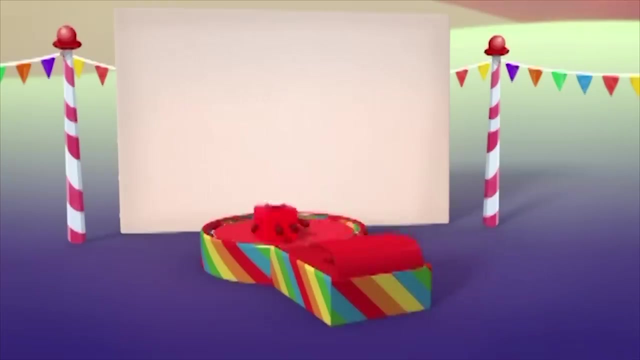 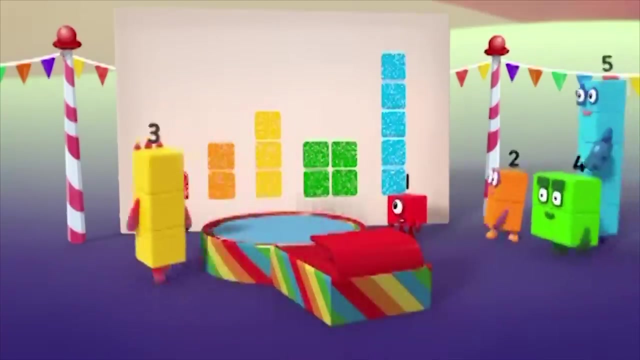 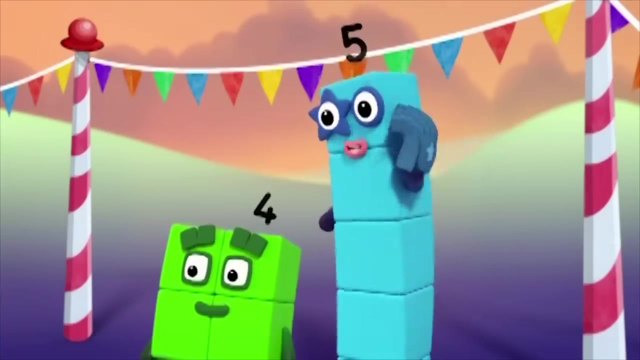 equals four. Every big shape is made up of lots of little ones, So lots of little ones can make every big shape. Look what I can do. Whee, You made all of us All right. Well done, And just in time for the grand finale. 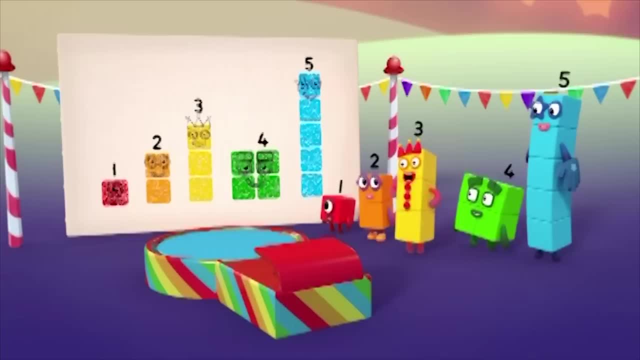 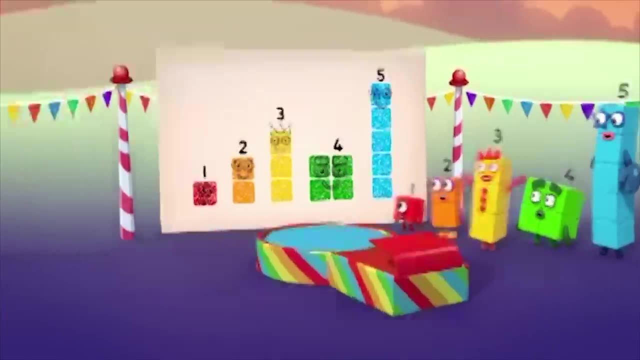 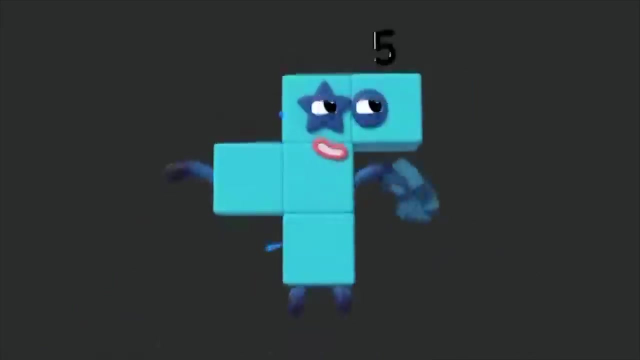 What better way to celebrate opening my new park than with fireworks. Ooh, May I present the Sky At Night. Whee, Yay, Woo-hoo, Yeah, Wahoo, Woo-hoo, Yay, Yeah, Woo-hoo. 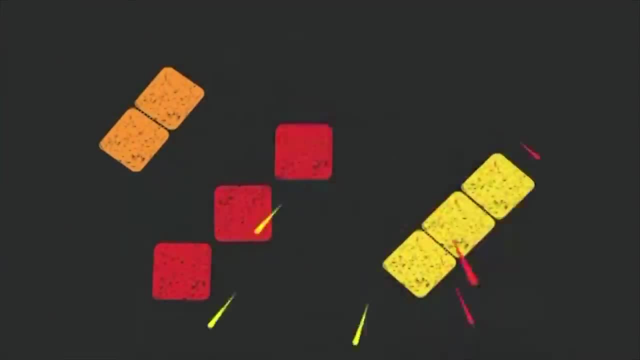 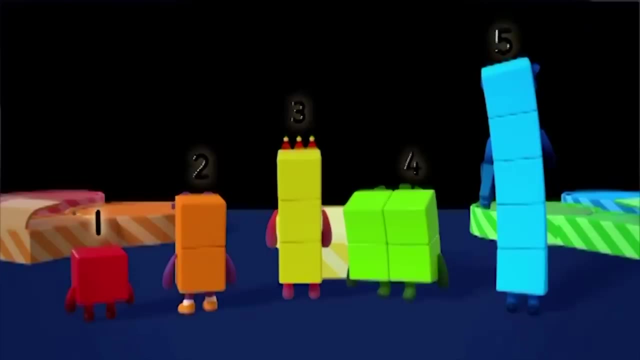 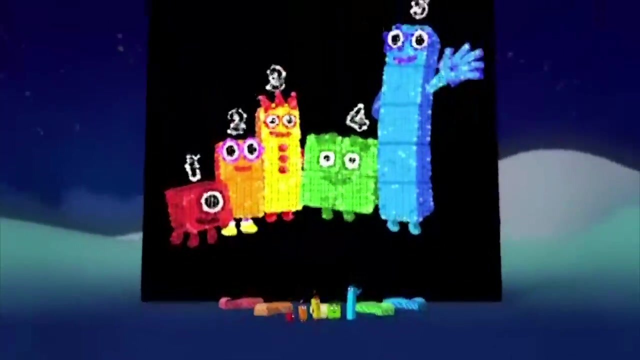 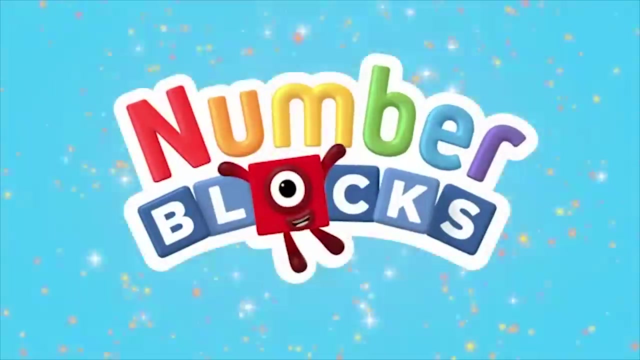 Wahoo, Wahoo, Wahoo, Yeah, Wahoo, Wahoo, Yeah, Wahoo. You see one, when we all work together, the sky's the limit. Yeah, Yeah, Wahoo. You can count on us with a number box. 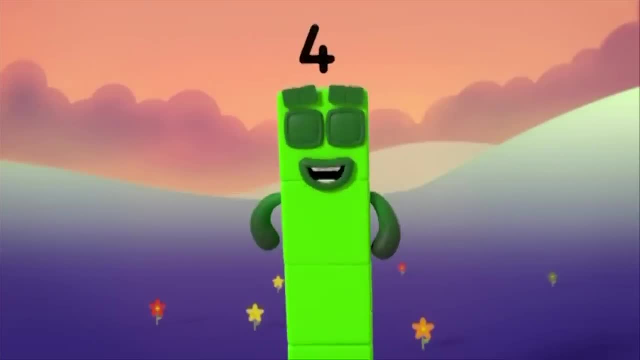 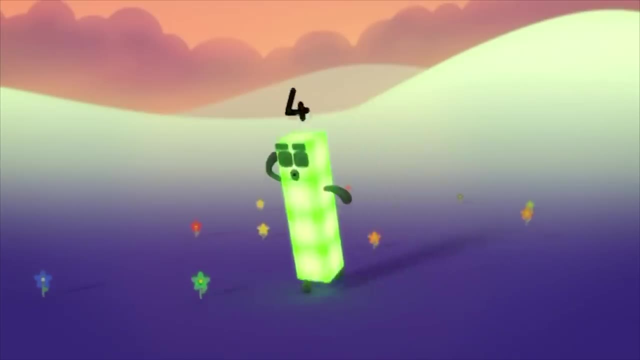 I'm number four And I am sure that I've got four blocks to play with and the whole of me is four: One, two, three, four. One is a part of me And three is a part of me, And the whole of me is four. 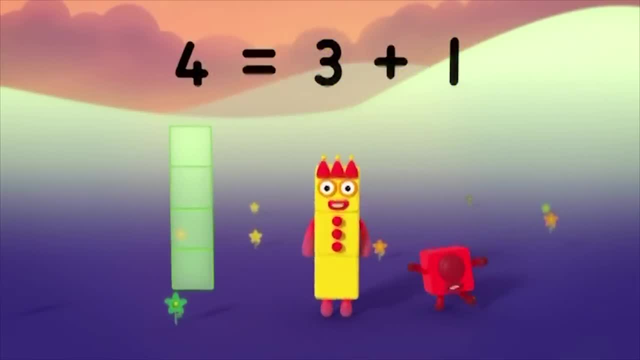 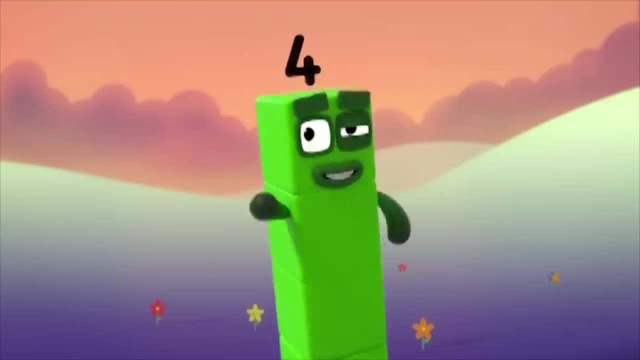 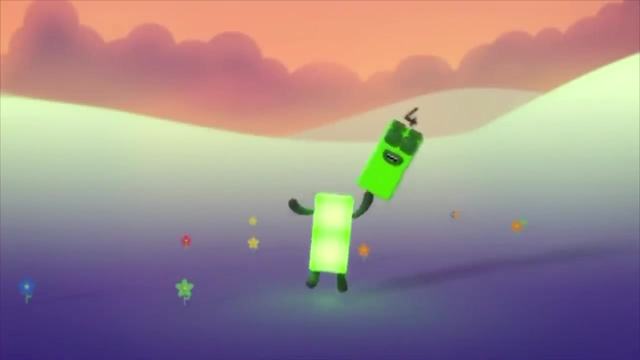 Watch, And three And I'm a part, I'm one And I'm a part, And the whole of me is four. Now here is something more that's different from before. Two is a part of me, And two is a part of me. 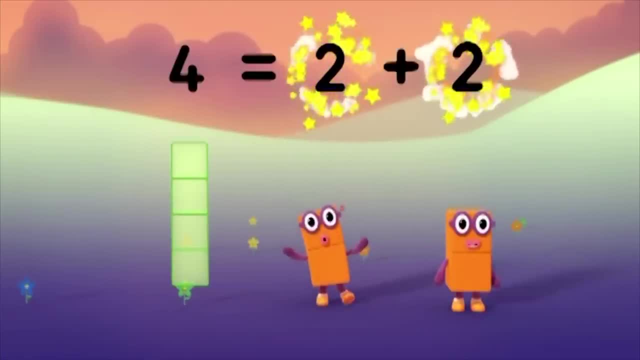 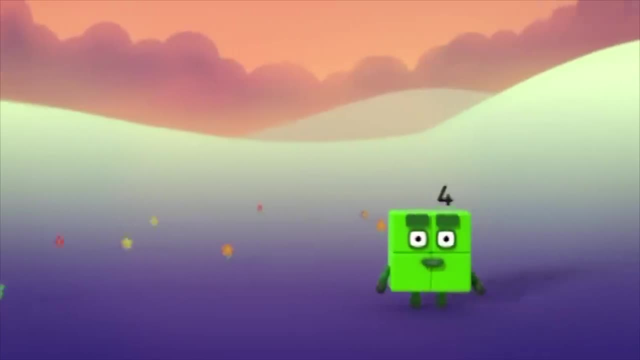 And the whole of me is four. Watch, I'm two and I'm a part. I'm two and I'm a part, And the whole of me is four. I'm a square. look Four sides, four corners. I'm number five. 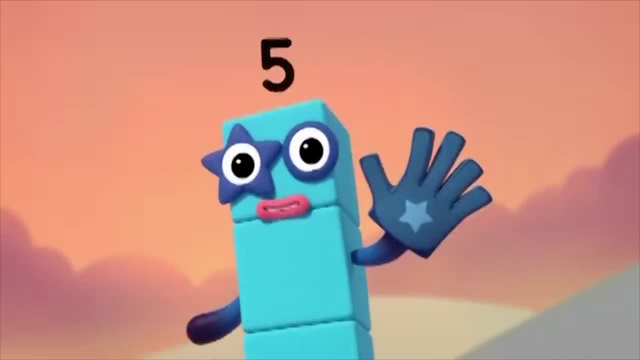 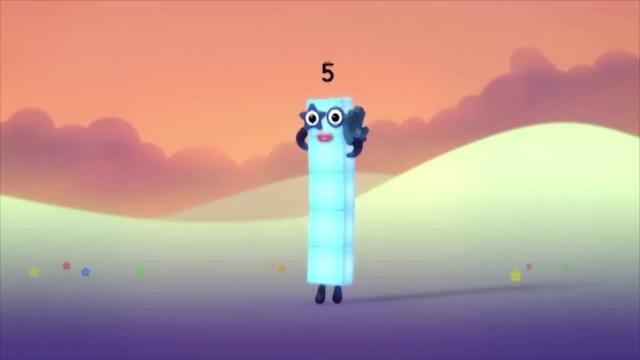 I am alive. I've got five blocks to play with and the whole of me is five. One, two, three, four, five. One is a part of me And four is a part of me, And the whole of me is five. 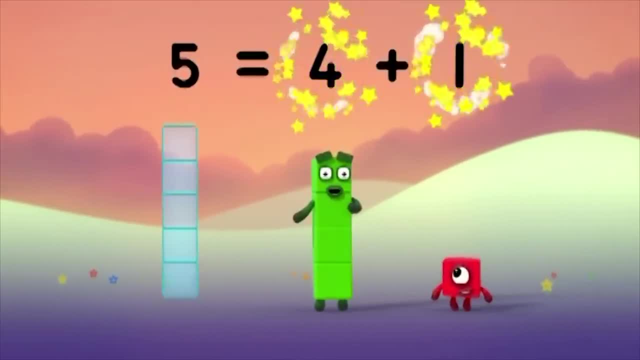 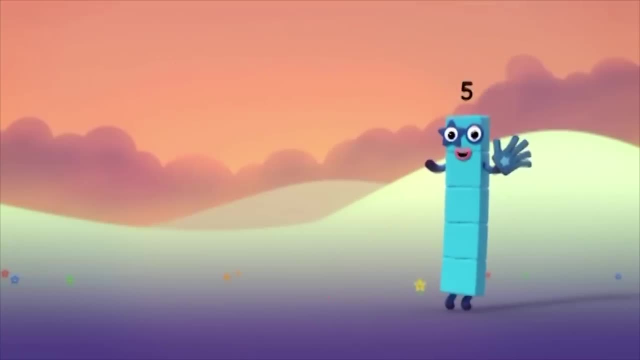 Watch. I'm four and I'm a part, I'm one and I'm a part, And the whole of me is five. But now I feel alive going into overdrive. Two is a part of me And three is a part of me. 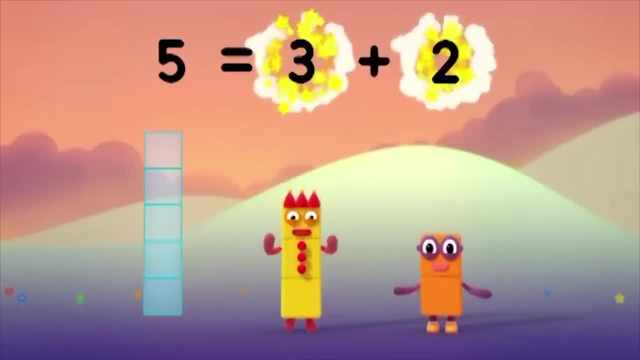 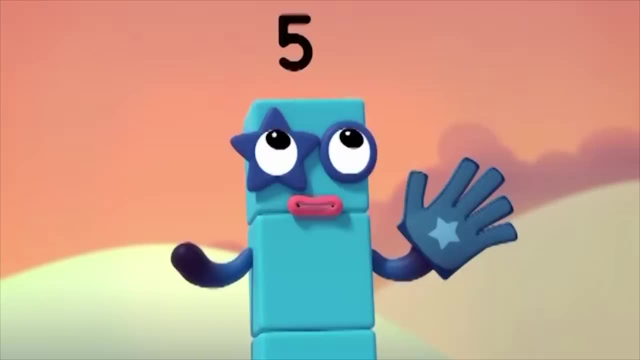 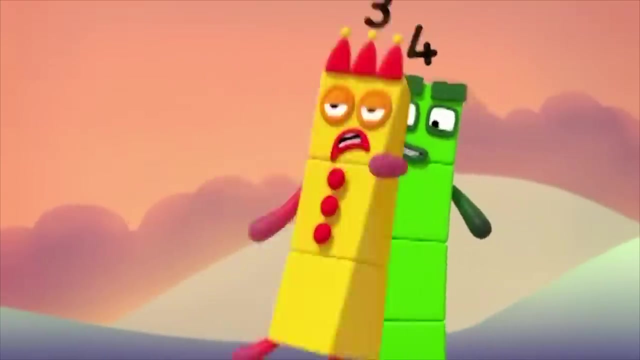 And the whole of me is five. Watch, I'm three and I'm a part, I'm two and I'm a part, And the whole of me is five High five. Making friends is easy when you can come apart. Splitting up is not so hard. it won't break your heart. 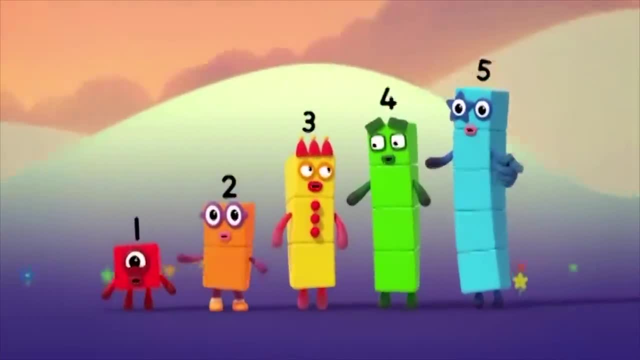 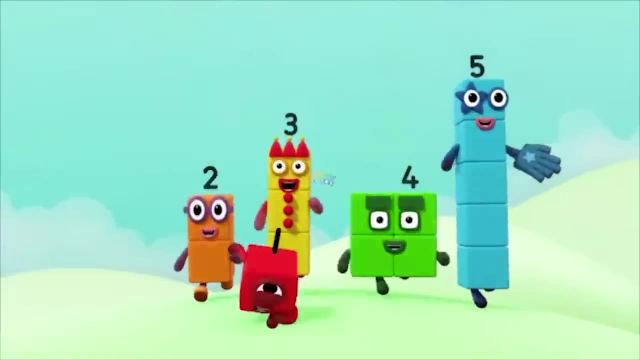 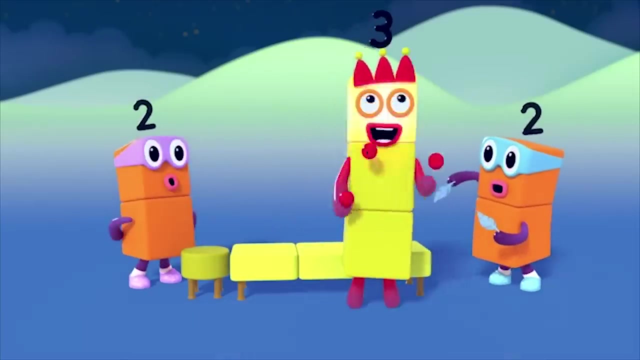 So when we fall to pieces, we have lost control. A hole is made of all its parts and the parts they make are whole. You can count on us. we're the number blocks One, two, three. Looks like fun. let's try it too. 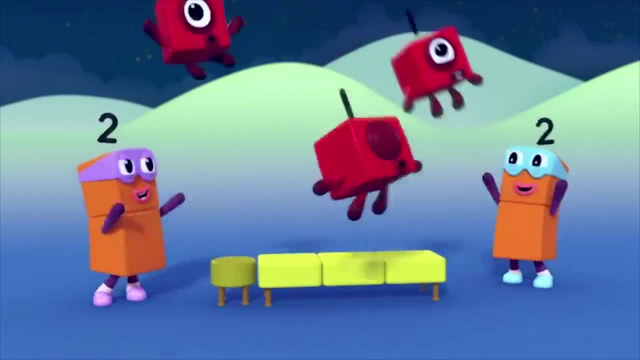 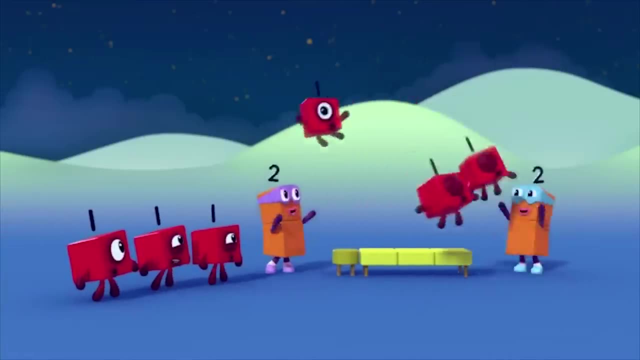 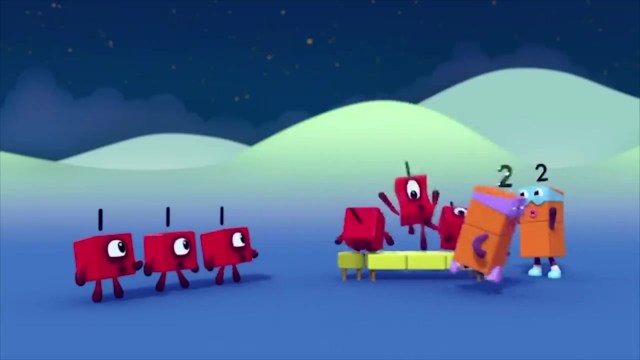 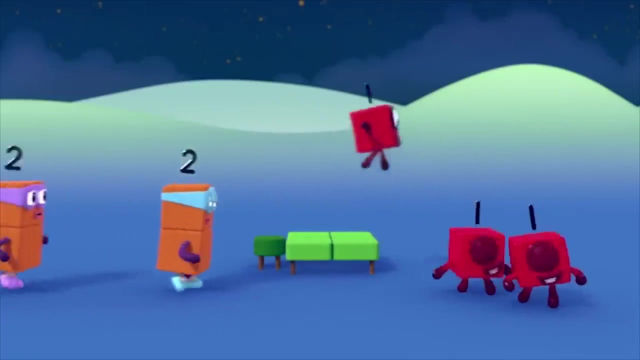 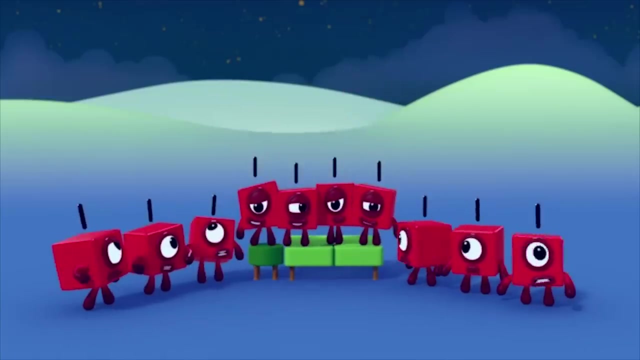 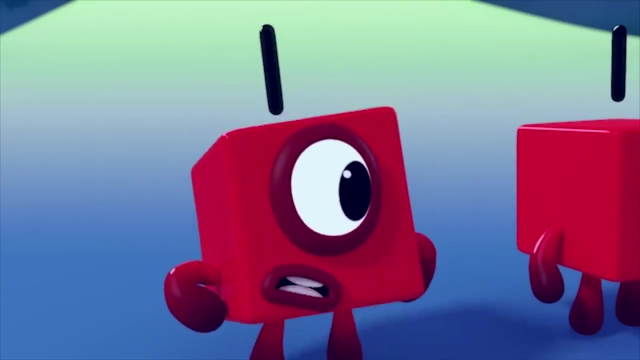 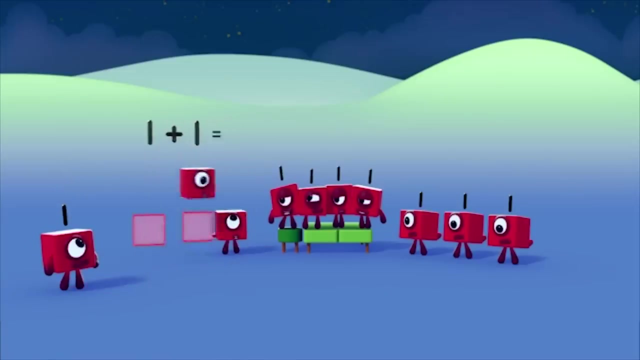 Just as soon as we both say BOOM, You can't stop A terrible two say toodaloo, We've only one thing to say: BOOM, Everyone, pull yourselves together. One one block. One plus one equals two. 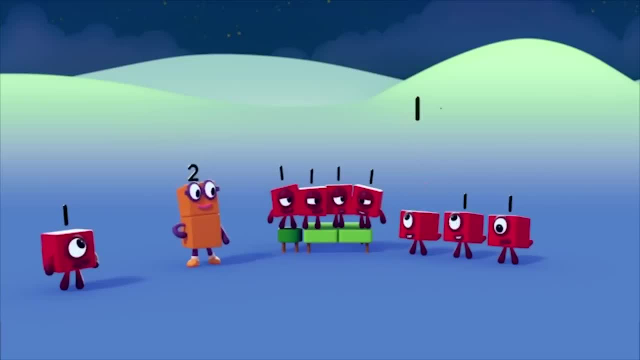 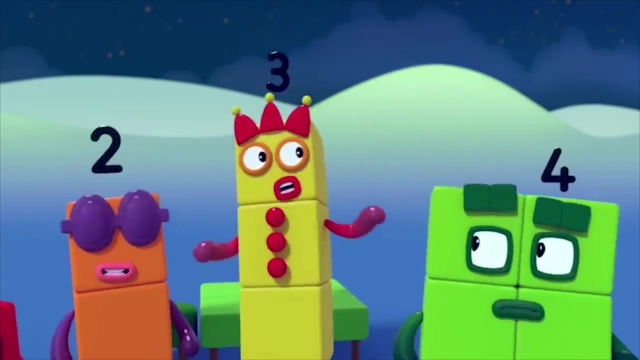 Two is two ones. One plus one plus one equals three. Three is three ones, Three is three ones. Four is four ones. Where are they? Where did those terrible twos go? Don't look at me. What all of the noise. 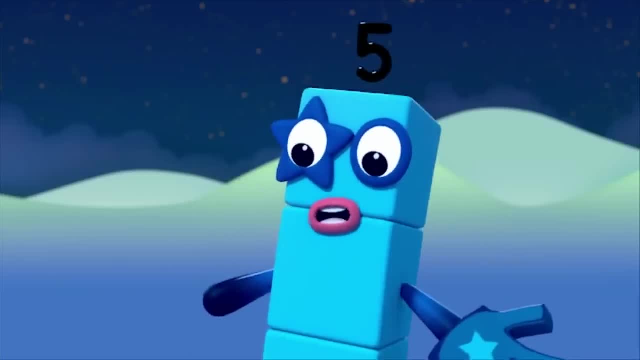 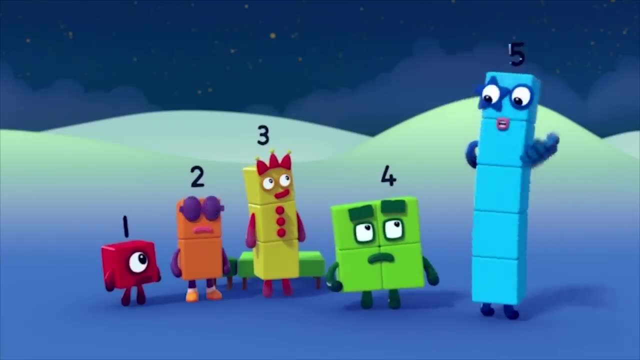 The terrible twos are playing tricks on us. Where are they now? I have to be square with you. they made me. What did they make you? You can tell us four. No, they made me. Well, I made them. 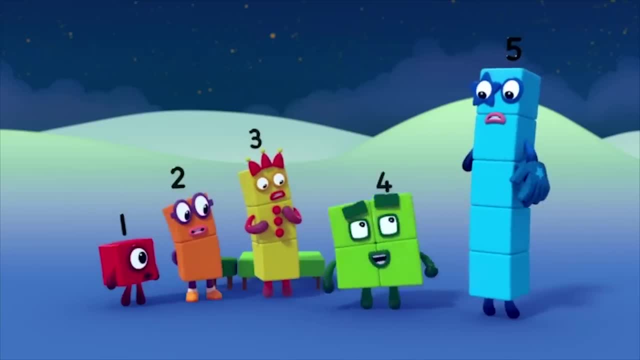 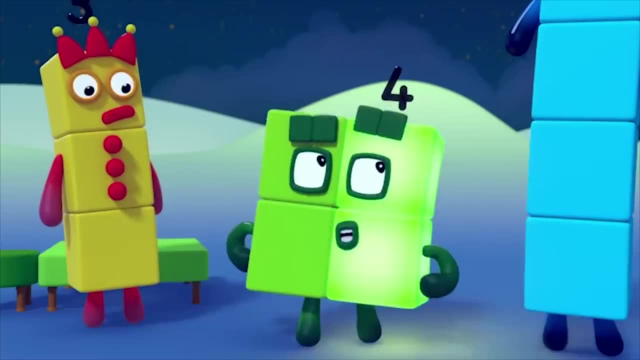 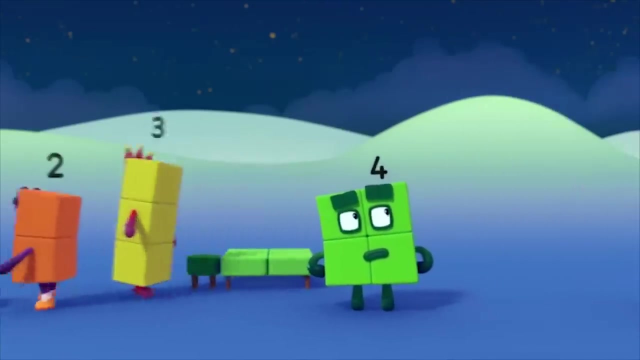 Then they made me: Huh, I'm the terrible twos, I'm four lots of one, but I'm also two lots of two. You're funny, Don't be silly. That's a very funny joke. Four equals two plus two. 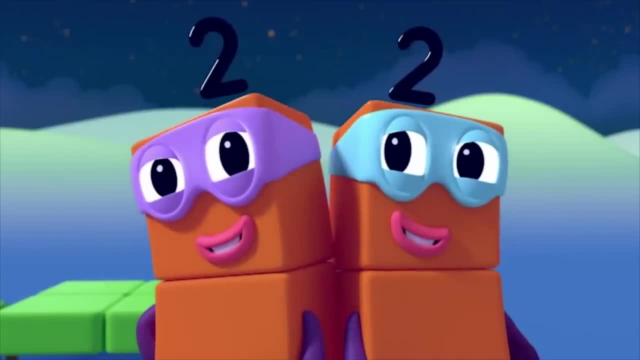 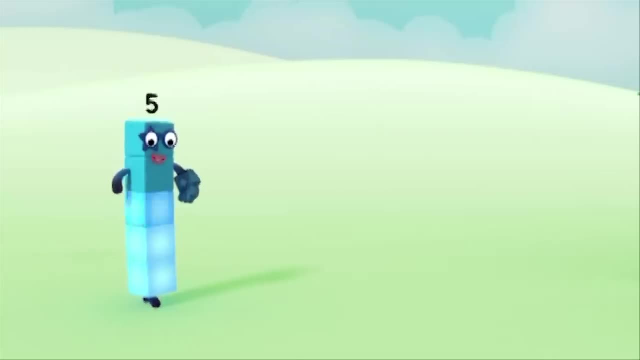 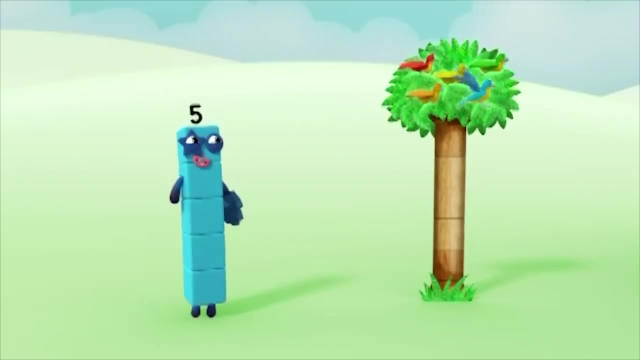 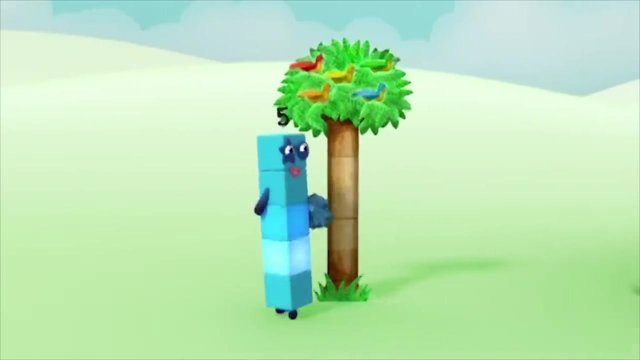 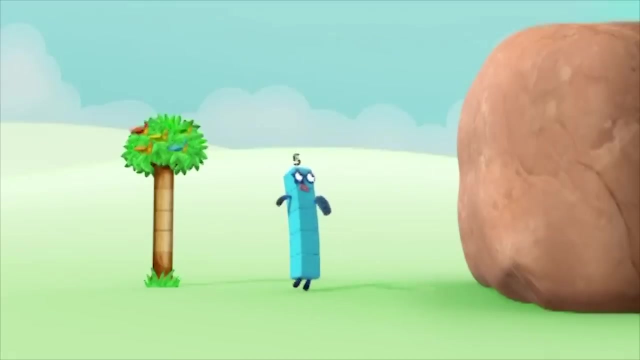 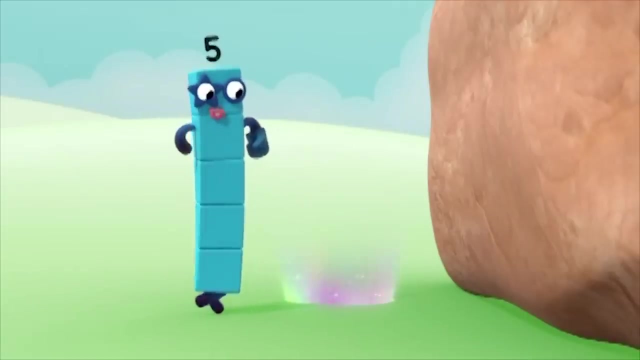 The terrible twos. Shh, I'm where I need to be. What is that silly sucking sound? Oh, look a hole so big and round. Why is it there? I do not know. I wonder what is down below. 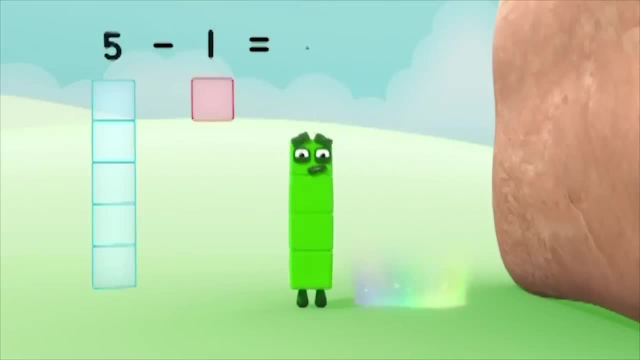 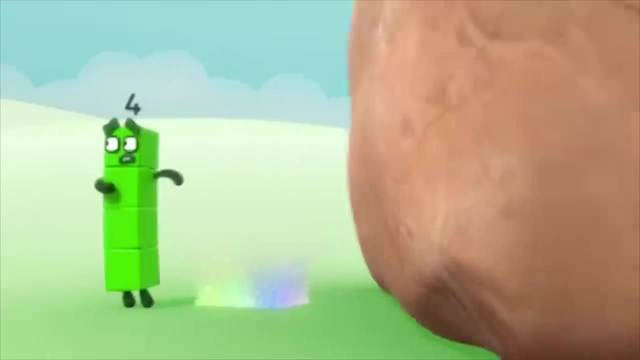 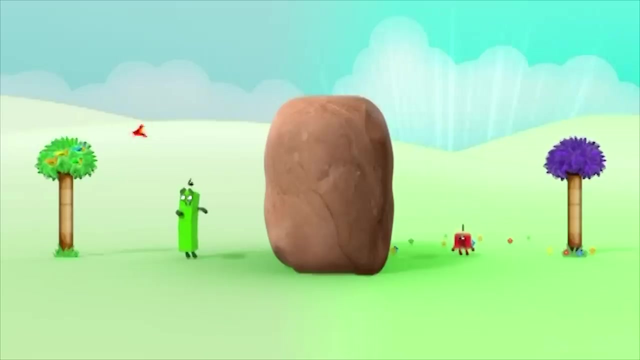 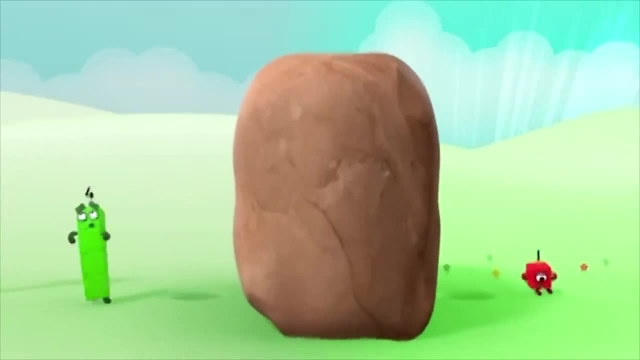 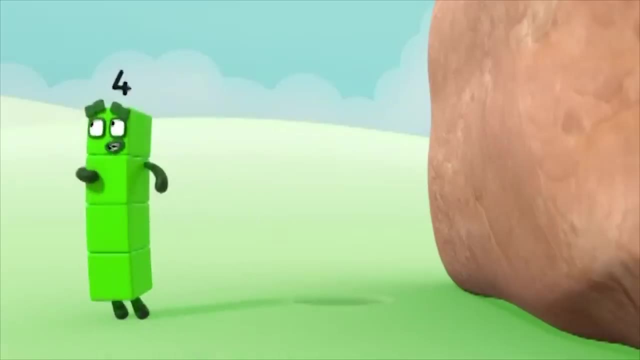 Here I am. What a wonderful day to be alive. Where, where, where is five? Five is gone. Where did she go? Is she all right? I do not know. Is she here, Is she there? I must keep looking everywhere. 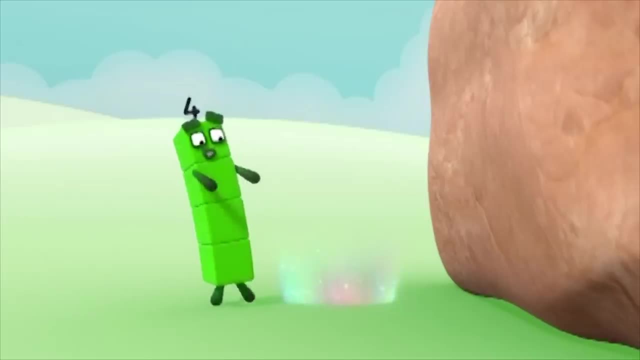 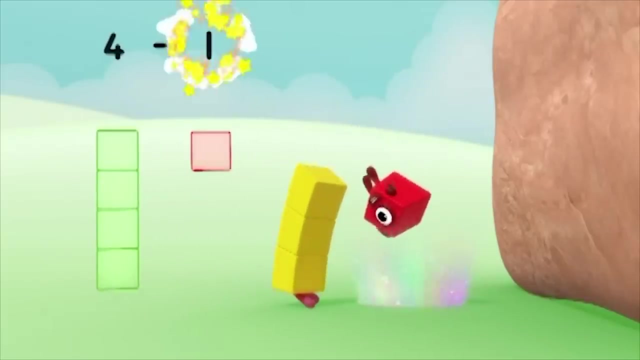 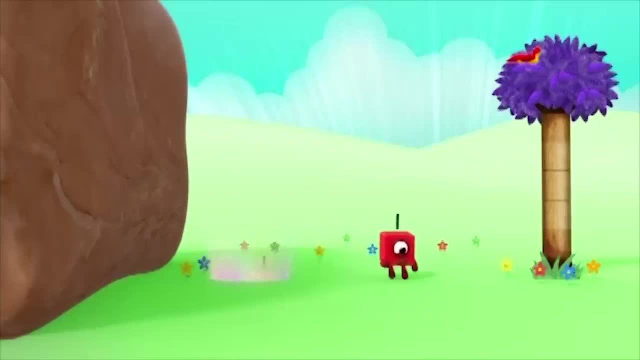 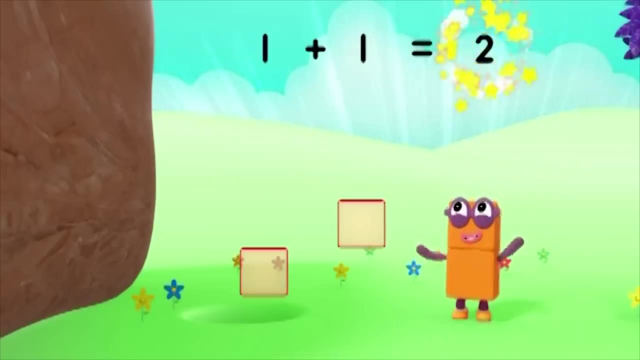 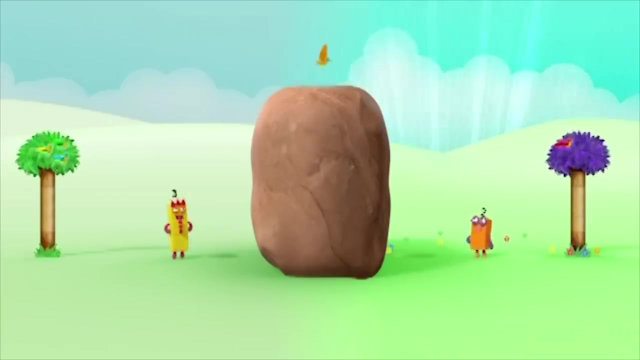 My head fell off. Where did it go? I am one. That was fun. One plus one equals Two. What is happening to me? I just got bigger, Did you see? Now I am three, and here I am. Now I am two, and here I am. 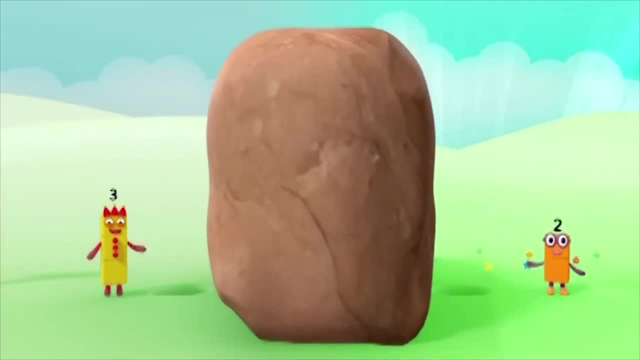 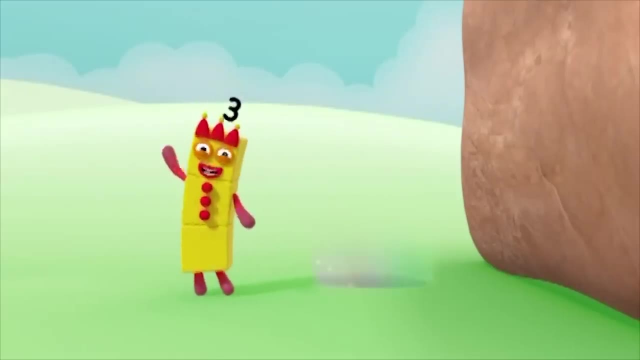 What a wonderful day to be alive. Where, where, where is five? I was five, then four, then three. Someone has played a trick on me. I do not mind at all. you see, Three is who I want to be. 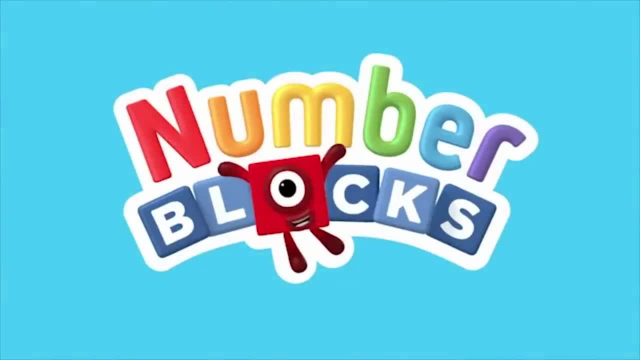 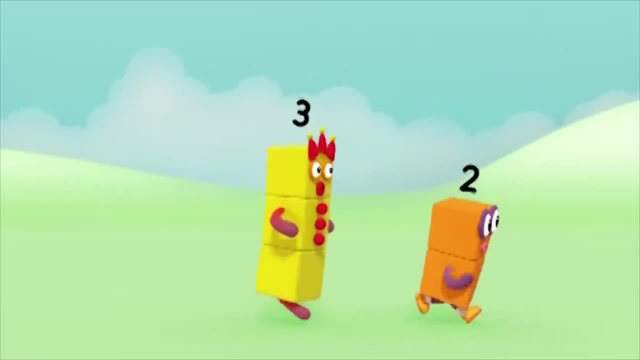 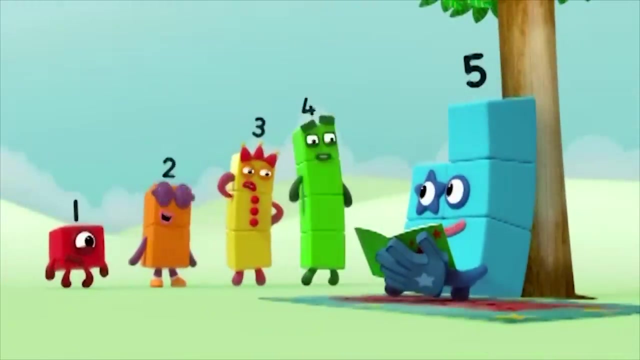 You can count on us with an autobox. Five minus three Equals two. A pair of pointing prints. Five found us, But but how? There? There Five, You are here. How did you Told you I was good? 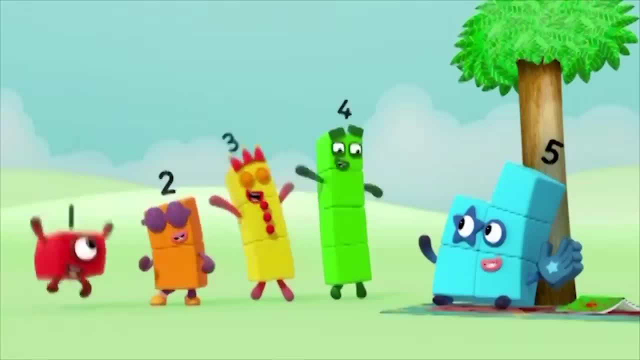 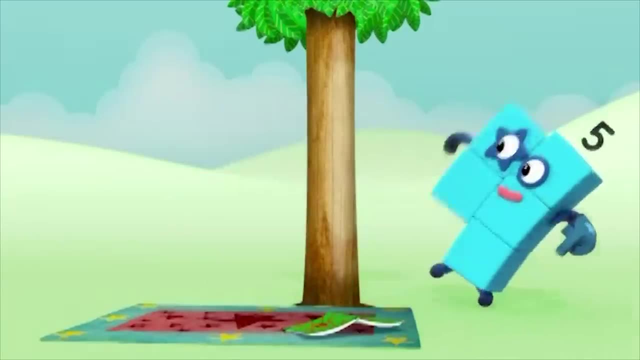 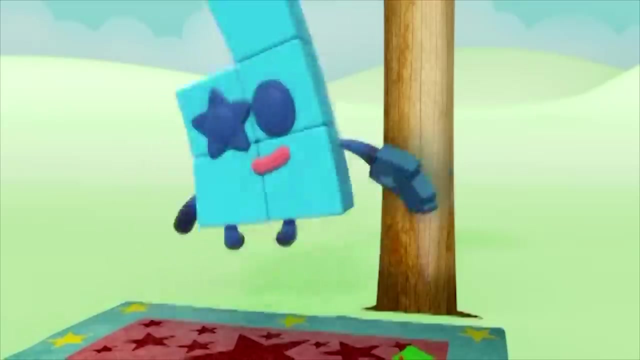 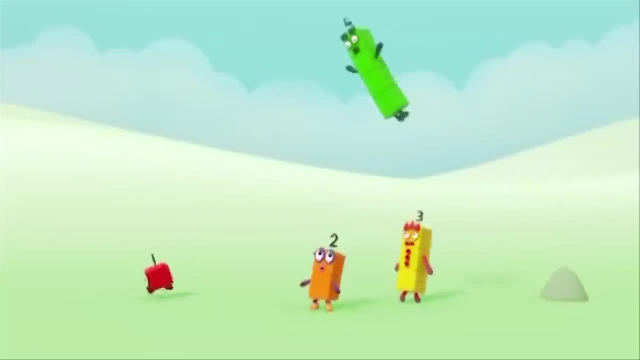 Oh, Rock Hack Hack. One Plus four Equals Equals five. Found you Amazing. Can you find me again? Five Minus four Equals one. Quit moving, I'm aòg отделing my desk. 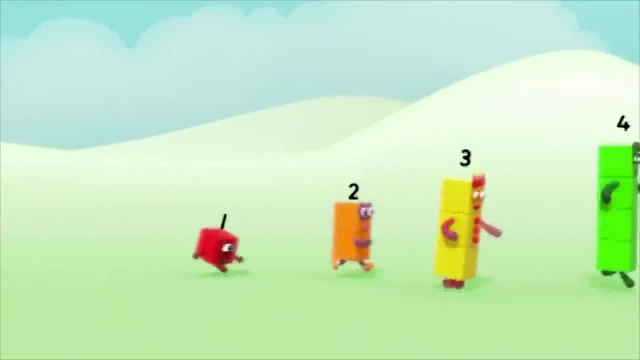 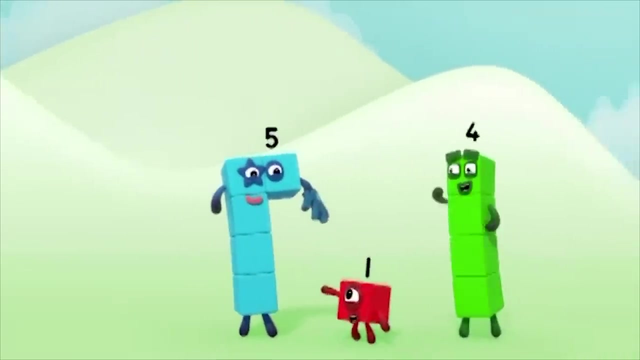 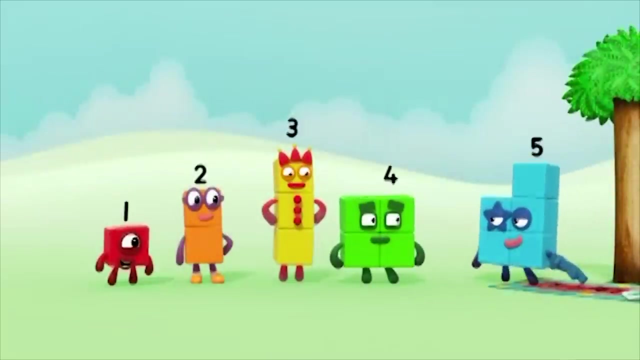 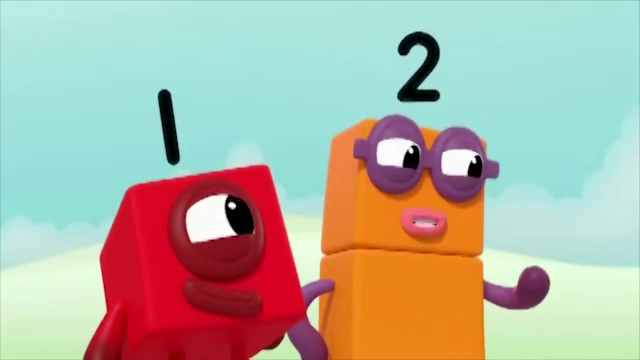 There, there Come on. Three plus two equals five- Found you. Fantastic, Can you find me again? Five minus two equals three. Found you, Found you, Found you. You stars, You all found me. Can you teach us to be as good at hide and seek as you? 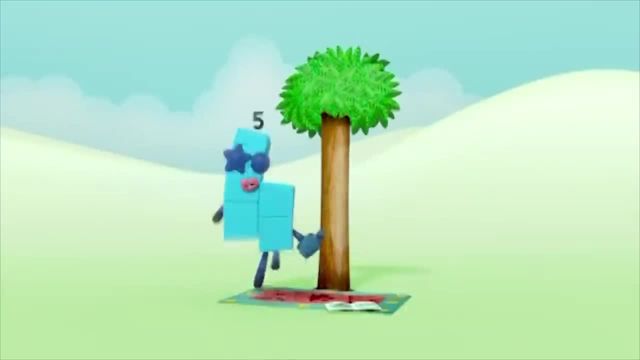 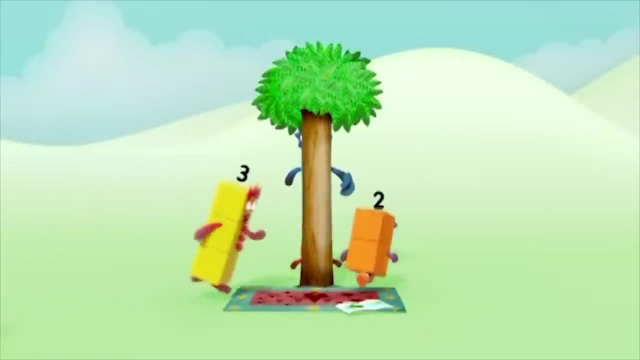 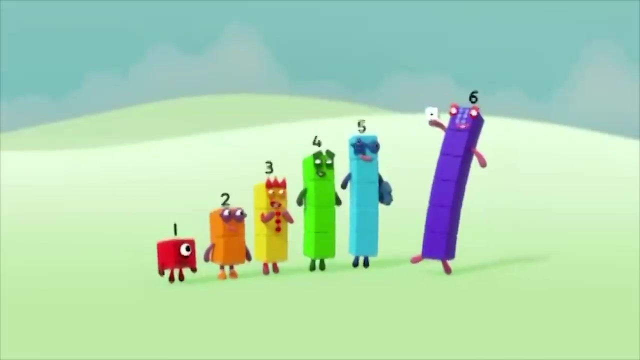 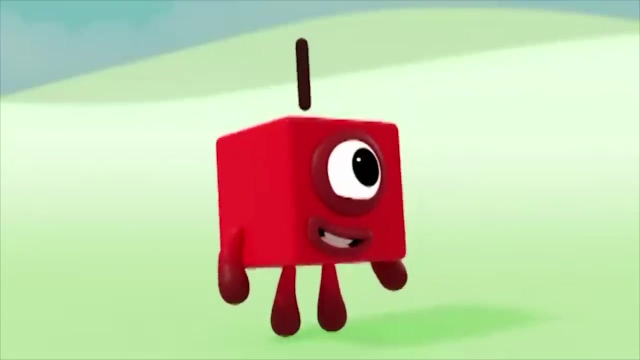 Sure, I can Try this. Four Oops. You can count on us. we're the number blocks. And this game goes like this: When you see a number, make the shape. One, One spot on the dice: Make the shape. 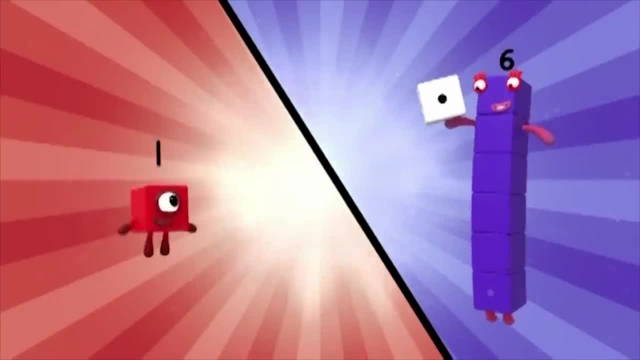 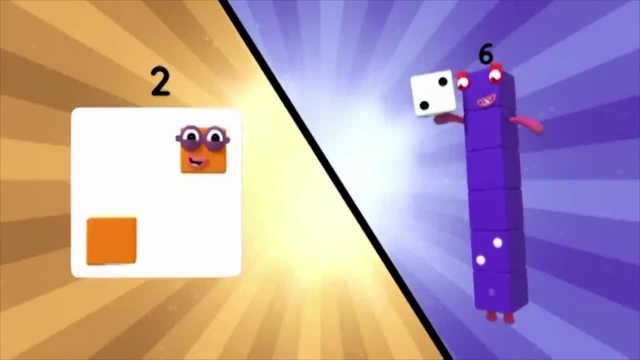 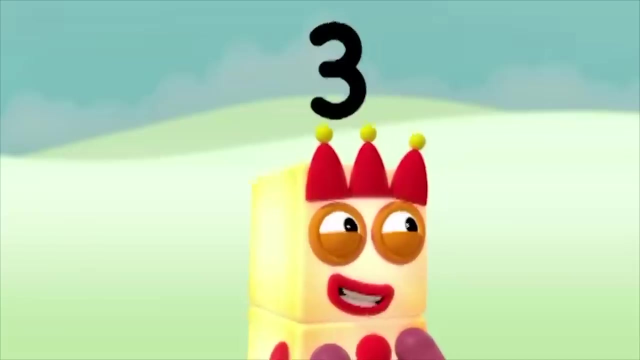 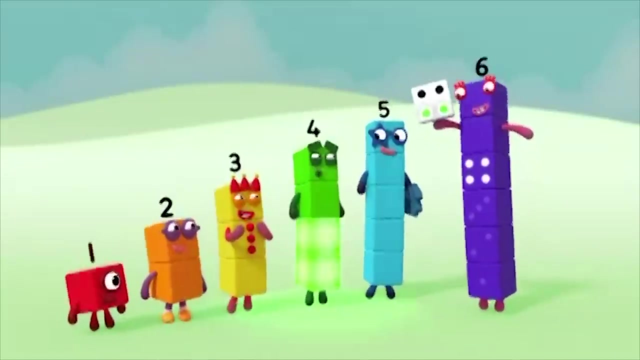 One, One, two, two spots on the dice: Make the shape Two. Make the shape Two. Make the shape Three. One, two, three, Three spots on the dice: Make the shape Three. One, two, three, four. 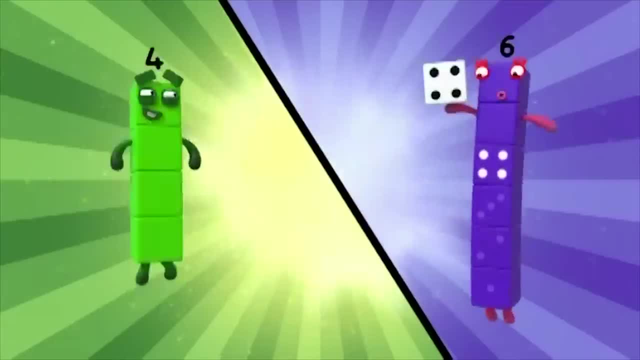 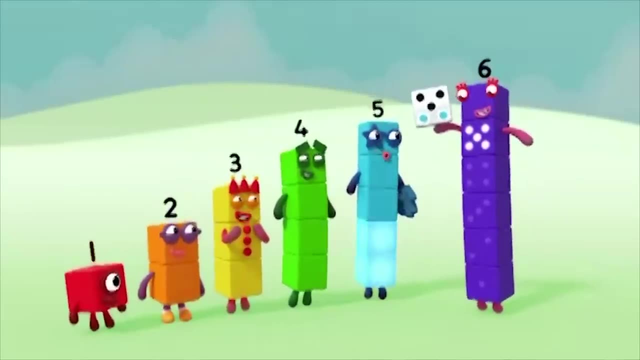 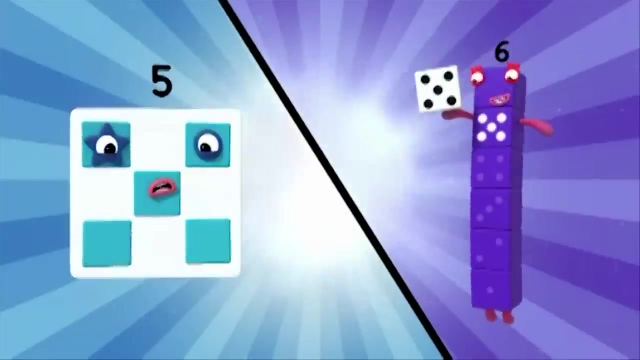 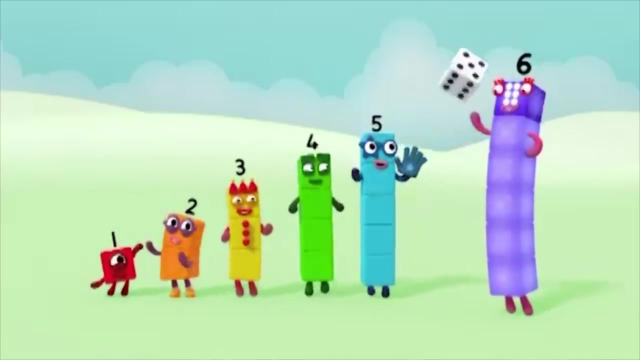 Four spots on the dice. Make the shape Four. It's a square One, two, three, four, five, Five. sports on the dice. Make the shape five: One, two, three, four, five, six, Six. sports on the dice. 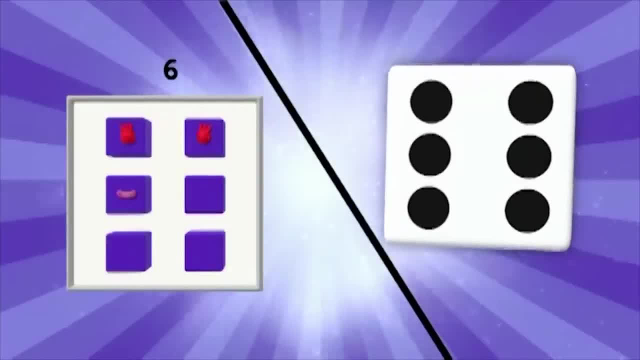 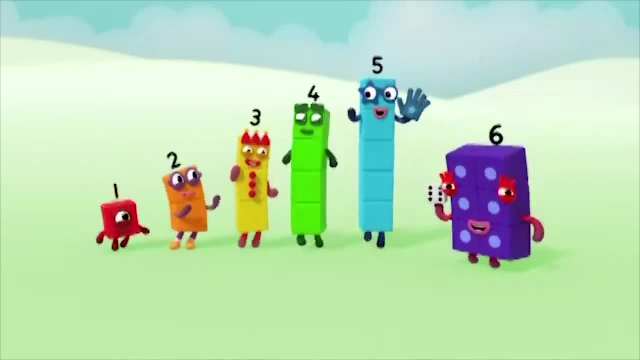 Make the shape six. I'm number six and I've got game. When you hear my name, you'll be glad you came. So take a chance, take my advice: Do a little dance and throw the dice. I'm number six. I'm in the mix. 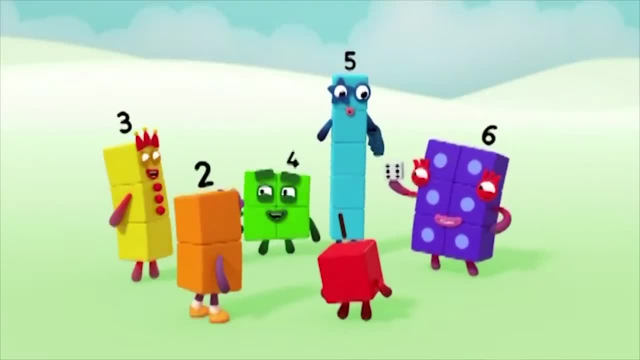 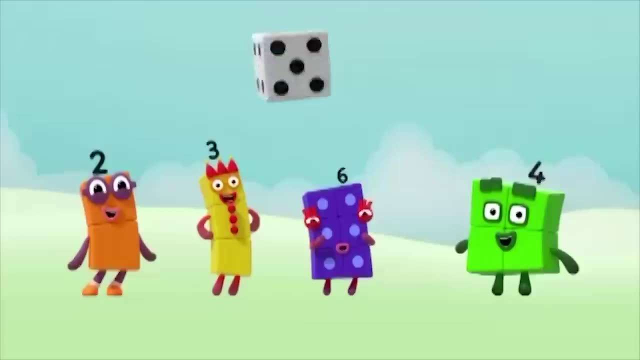 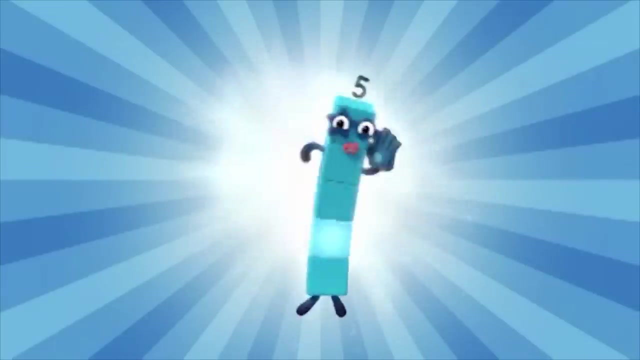 Good times are my go. that's how I roll New game. If you see your number, it's your turn to dance. Let's roll Five hand jive: One, two, three, four, five. One, two, three, four, five. 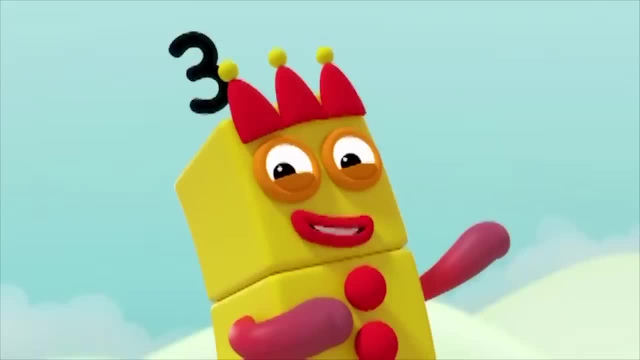 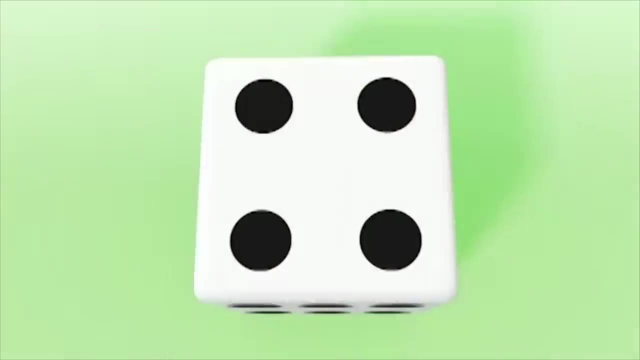 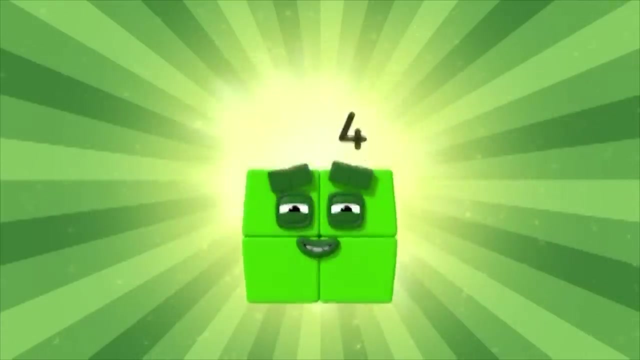 Three. look at me. One, two, three. One two, three, Four, Not sure, Oh, square dance. One, two, three, four. Two Time to use my dancing shoes: One two, one, two, one, two, One. This is fun. 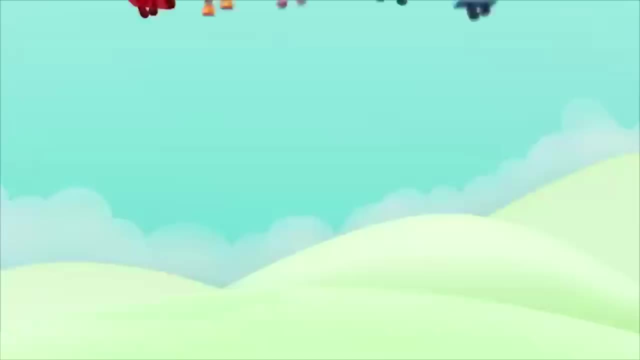 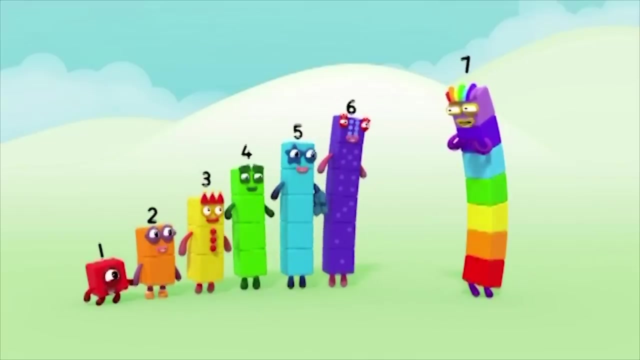 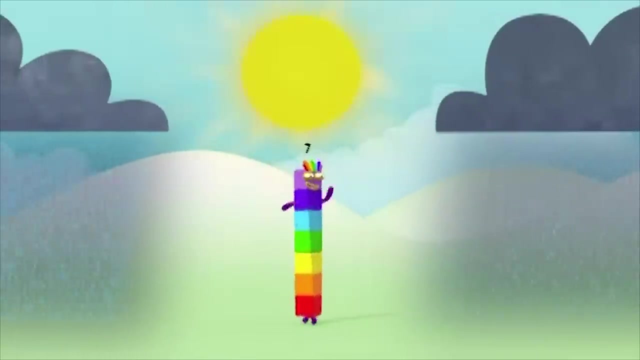 One, one, one one. You can count on us. we're the number box. Luckily, I know just what to do now. Seven minus one equals six. All you lovely blocks are my friends. I'm the luckiest number block in the world. I'm lucky number seven. I'm in a happy place. 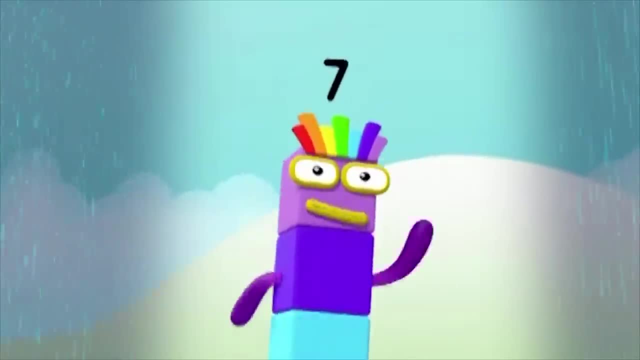 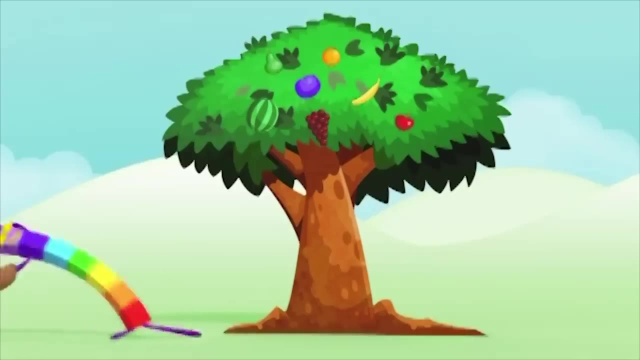 The sun is always shining and there's always. The sun is always shining and there's always. The sun is always shining and there's always A smile upon my face. I see a penny and I pick it up, And all day long I have good luck. I'm lucky number seven. 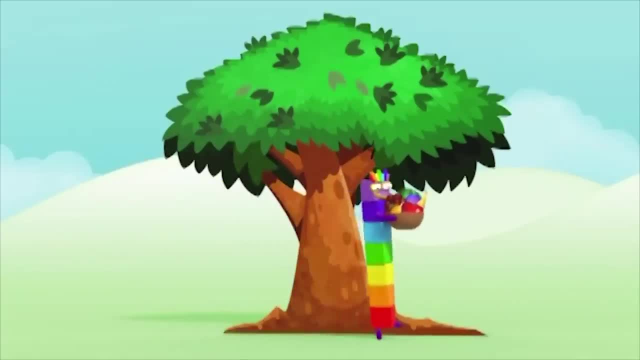 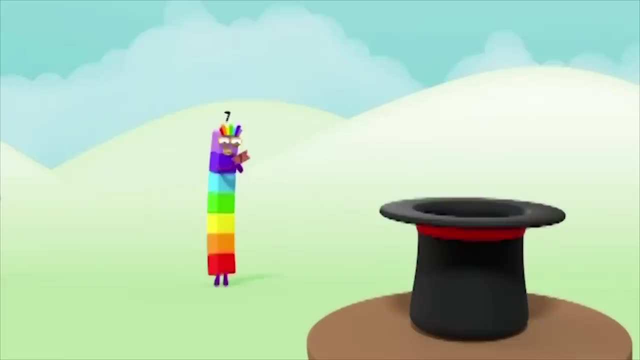 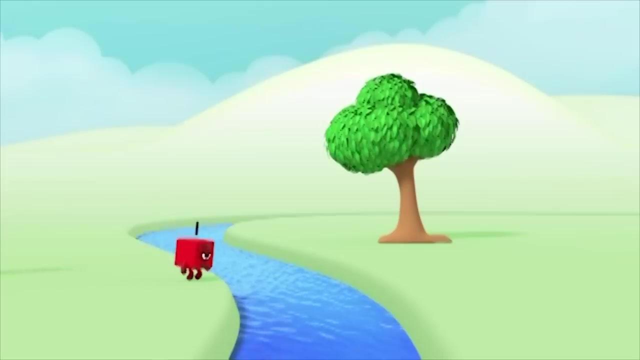 And everything is falling into place. I'm lucky number seven And, as you might have guessed, I always win the raffle With seven on your side. you're seven less In a pickle, you're in luck. I help you out when you get stuck, And if you stick with me, you're in luck. 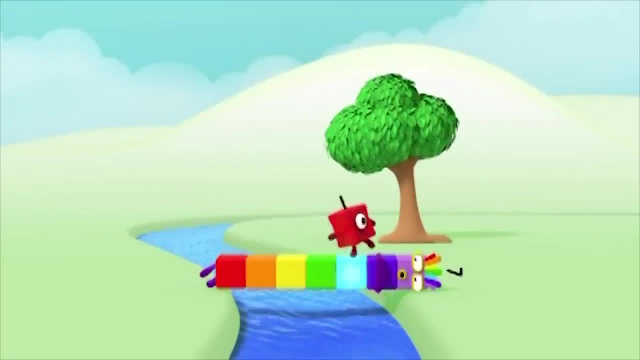 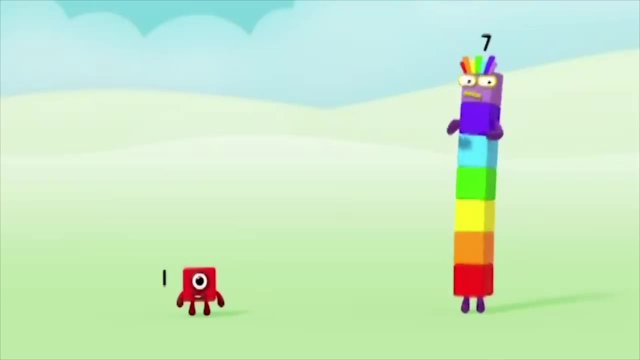 And if you stick with seven, Everything will work out for the best. Yay, Rainbow time- Red: My first block is the same as you. Orange. My second block is the same as two. Yellow: My third block is, just like number three, Green. 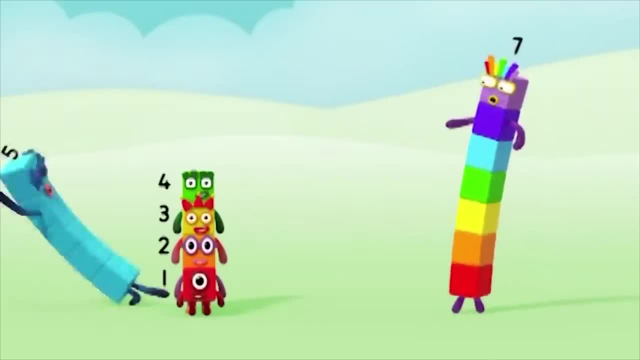 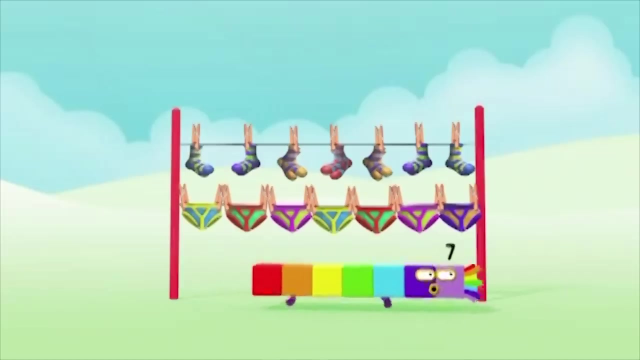 My fourth is green, as you can see. Blue for five, Indigo for six, Violet is for seven. Oh, That's me. I've got seven rainbow-colored locks. That makes me unique. I've got seven pairs of pants and socks, One for each day of the week. 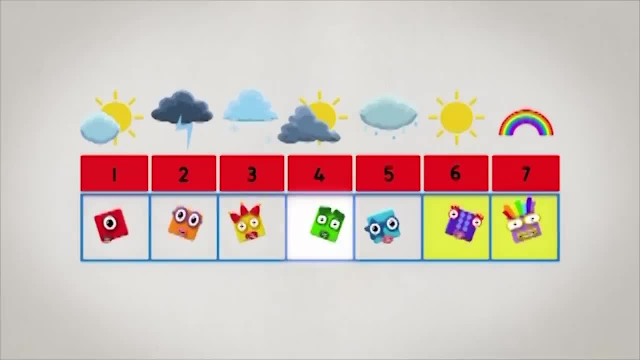 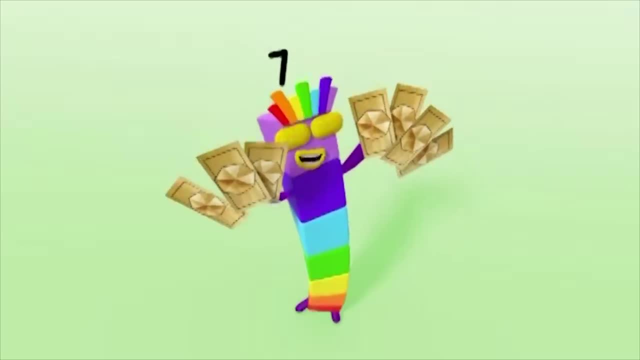 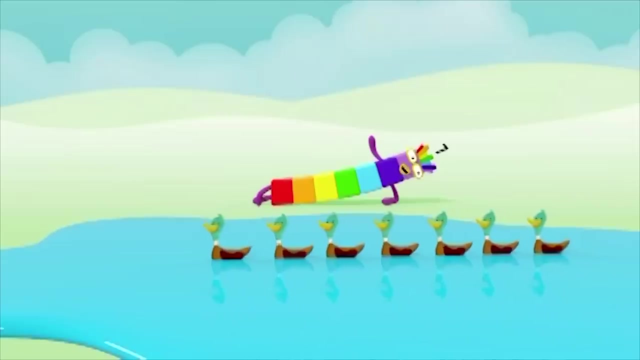 Monday, Tuesday, Wednesday, Thursday, Friday, Saturday, Sunday, One, two, three, four, five, six, seven. I've got seven golden tickets: One, two, three, four, five, six, seven. All my ducks are in a row. 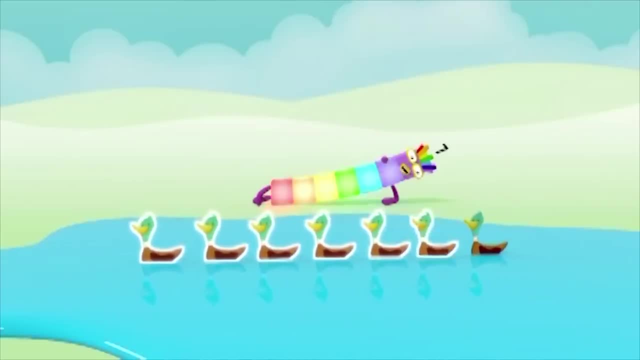 One, two, three, four, five, six, seven. All my ducks are in a row: 1,, 2,, 3,, 4,, 5,, 6, 7. Nothing's going to stop me. all my traffic lights are on go. 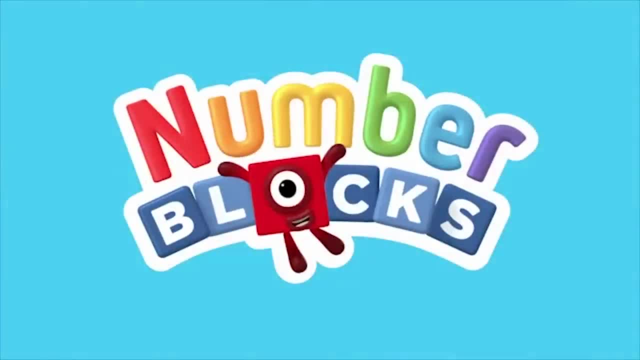 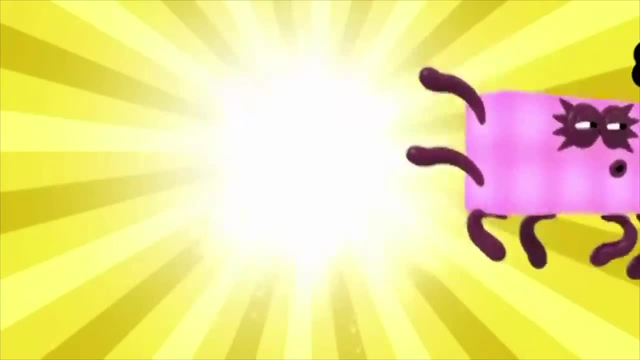 You can count on us. we're the number blocks: Octoblock crawl 1,, 2,, 3,, 4,, 5,, 6,, 7,, 8, crawl. He can run really fast In a blur. 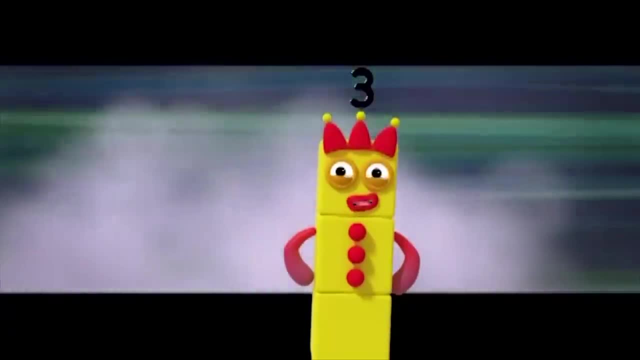 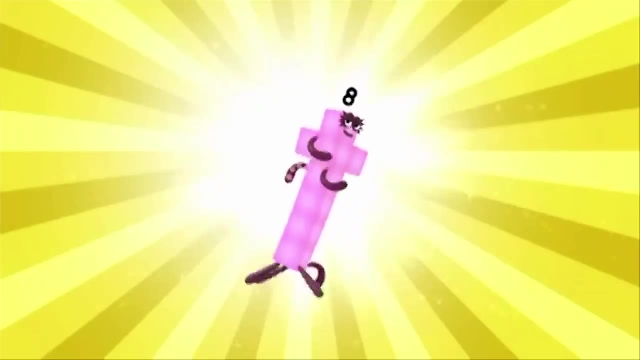 Speeding past. He is Octoblock, Octoblock, Octoblock. run 1,, 2,, 3,, 4,, 5,, 6,, 7,, 8, run. He's an eight-legged hero. He's strong and he's stocky. 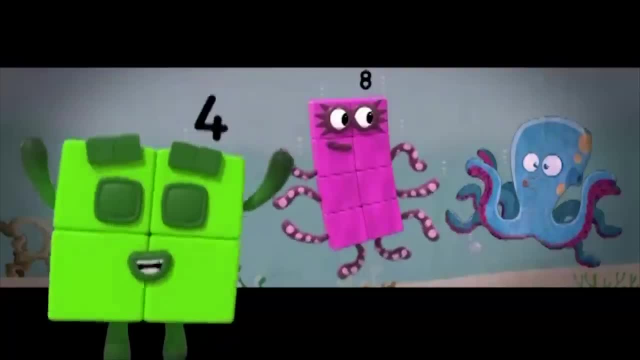 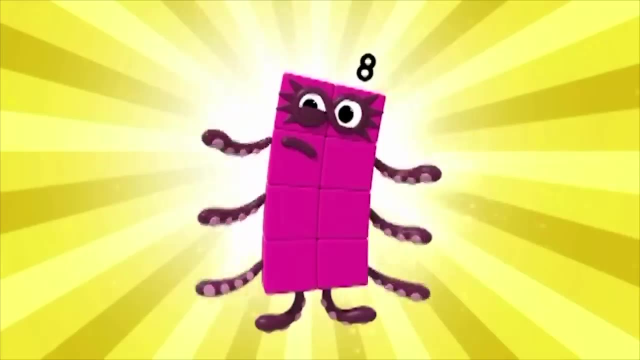 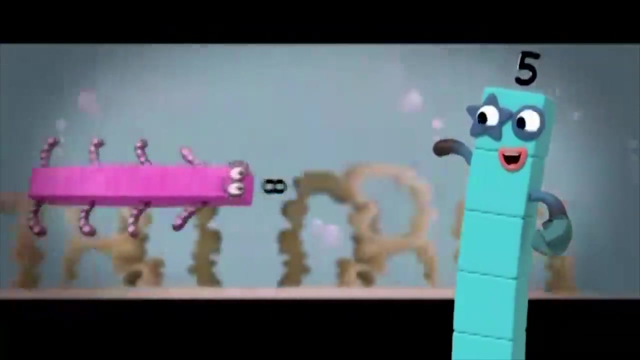 Sort of an octopus, only more blocky. He is Octoblock, Octoblock, Octoblock. Uh, what do octopuses do? He can swim. Add great seed Like a weird millipede. He is Octoblock, Octoblock. 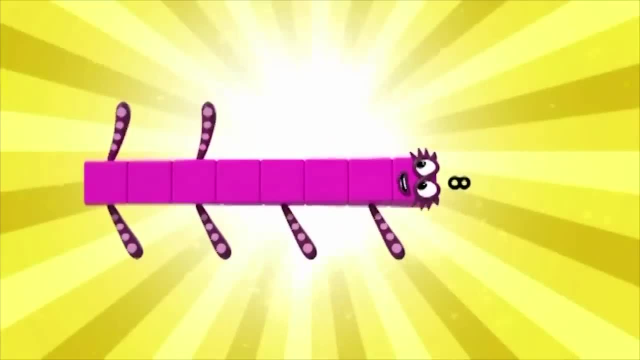 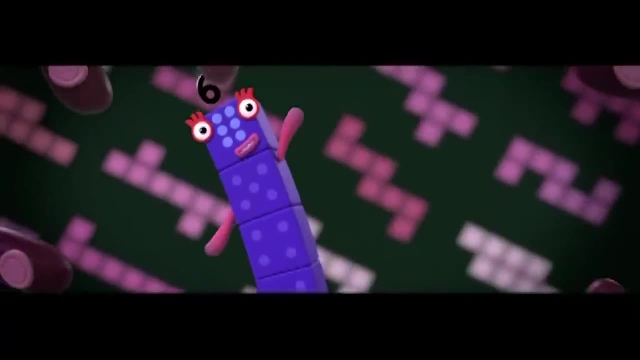 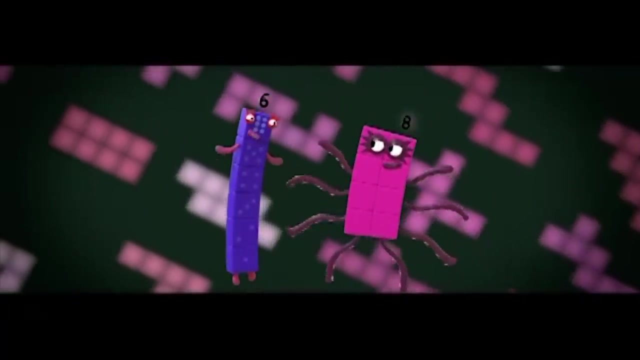 Octoblock. swim 1,, 2,, 3,, 4,, 5,, 6,, 7,, 8, swim: He's got eight legs, Or maybe they're arms. When he gives you eight hugs at once, you'll fall for his charms. 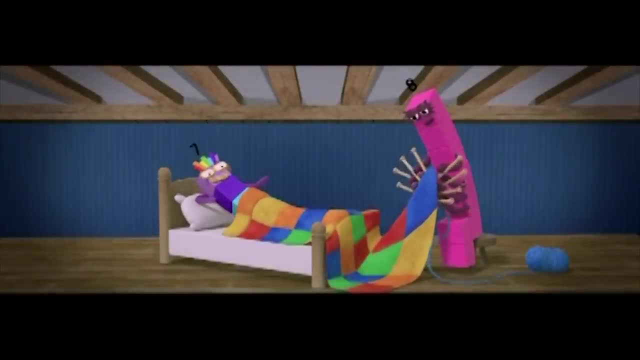 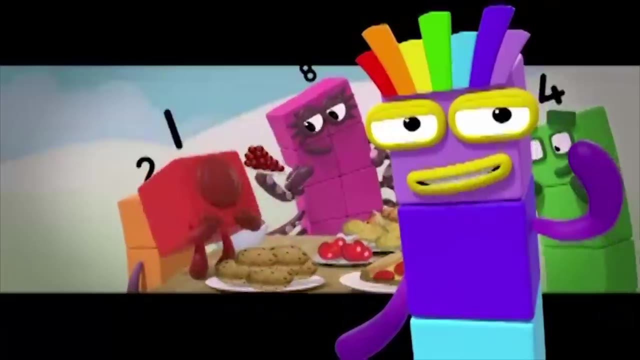 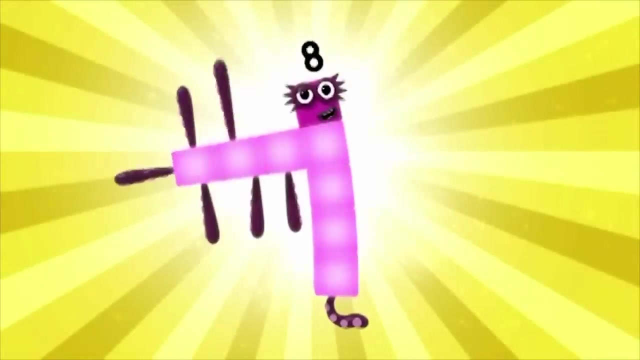 He can knit you a great woolly blanket. He can cook you an eight-course banquet. But don't get too close, Don't be too keen. He's the tickliest tickler the world's ever seen. Octoblock tickle 1,, 2,, 3,, 4,, 5,, 6,, 7,, 8, tickle. 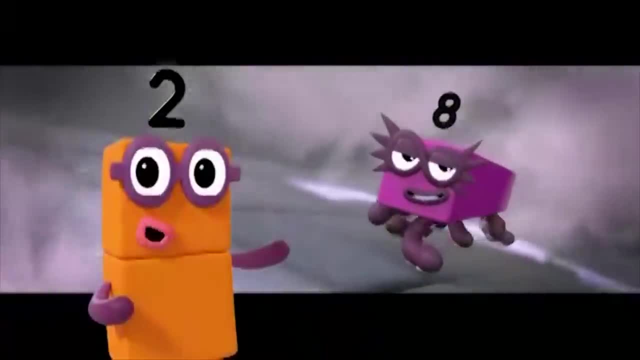 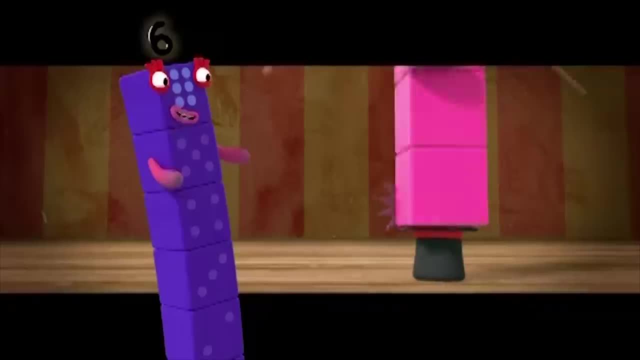 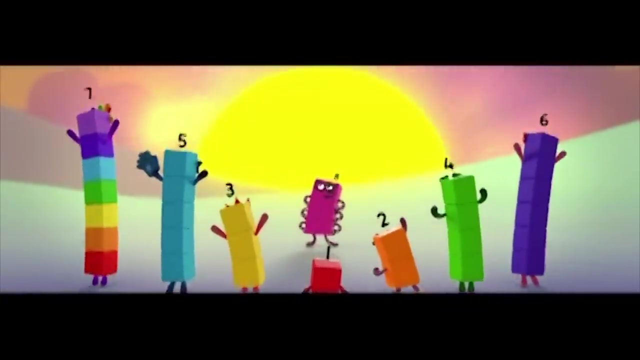 He can stand really tall, He can climb up the walls, He can juggle eight balls at a time, He can skate like a dream. He's his own rowing team And his dancing is something sublime. He's Octoblock, Octoblock, Octoblock. 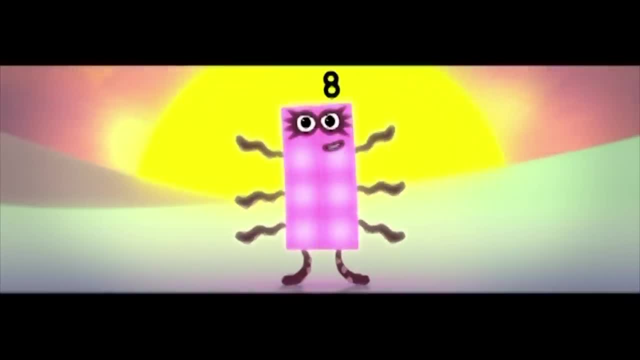 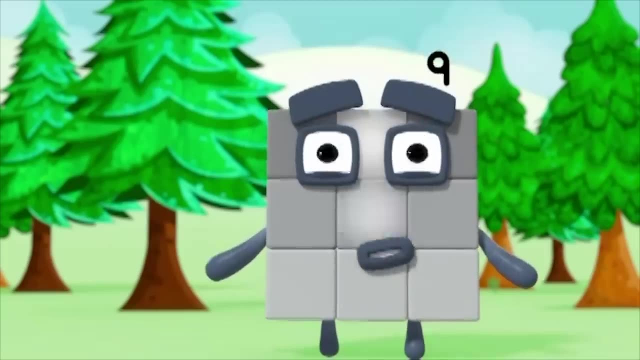 Octoblock 1,, 2,, 3,, 4,, 5,, 6,, 7,, 8!. You can count on us. we're the Octoblocks 1,, 2,, 3,, 3 blocks top to bottom. 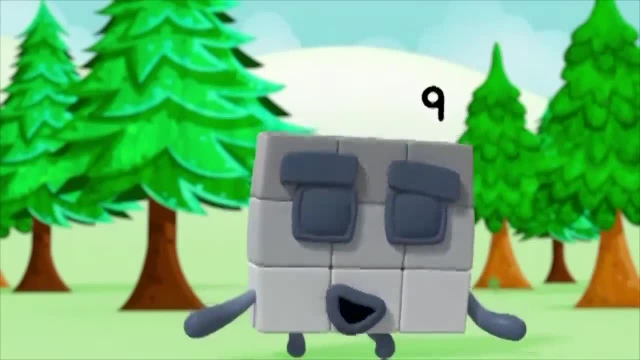 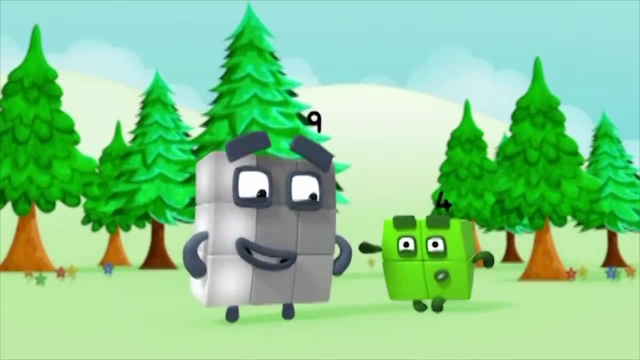 1, 2, 3, 3 blocks. if you've got them, 3 lots of 3, 3 in a line, As you can see, 3 lots of 3 make 9. That's right: 1, 2, 3, 4, 5, 6, 7, 8, 9!. 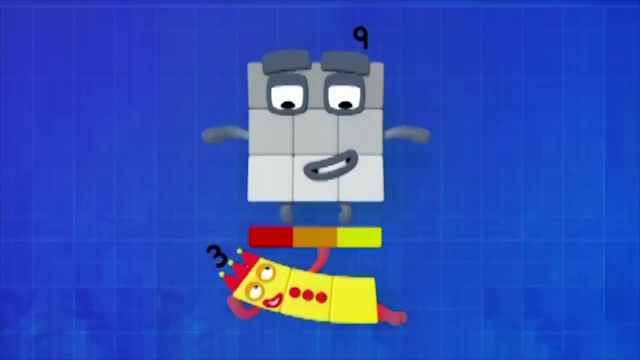 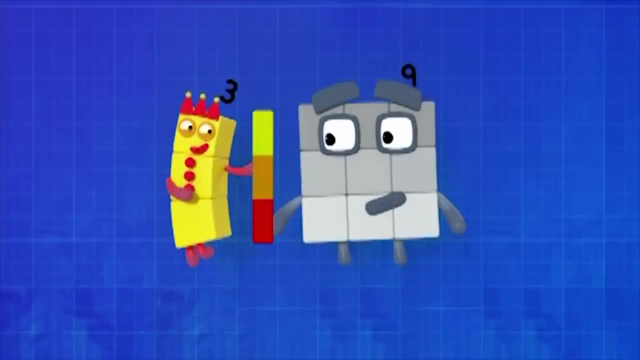 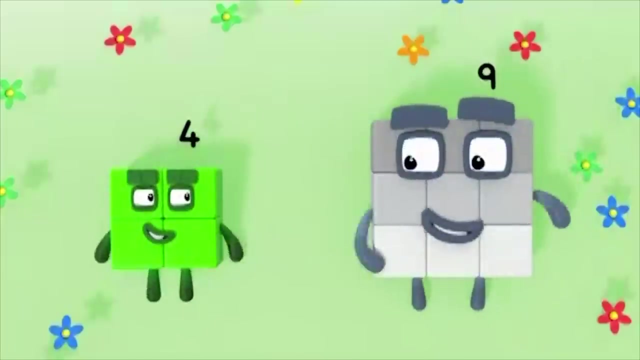 I'm 3 blocks up and down And 3 from side to side. I'm the same in both directions. I'm as tall as I am wide. That's why I'm square like you. I'm 3 by 3, you're 2 by 2. 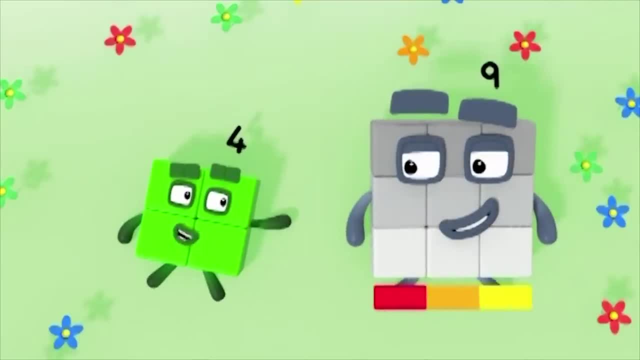 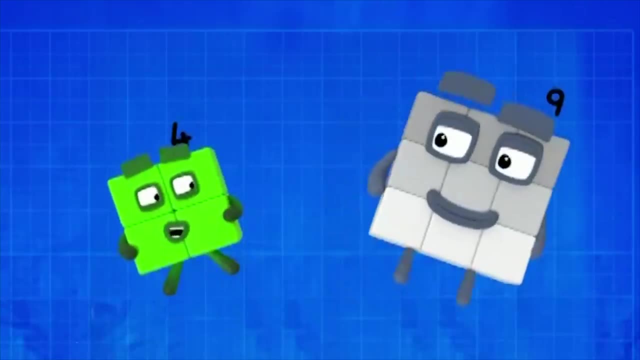 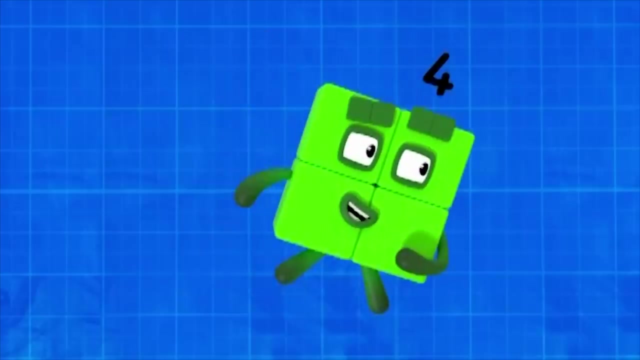 I'm 2 by 2, you're 3 by 3. That's why you're square, like me. We seem a very unlikely pair, But now you've explained it. I see The squareness we share. I'm 2 blocks up and down. 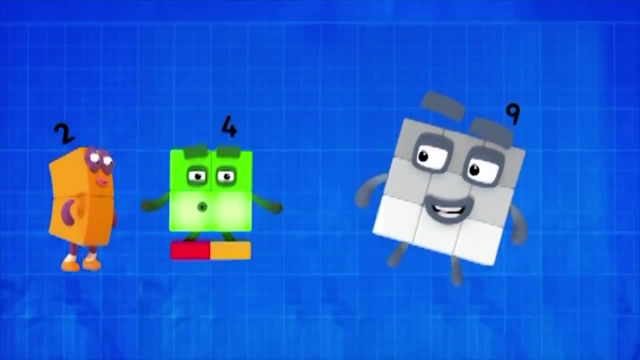 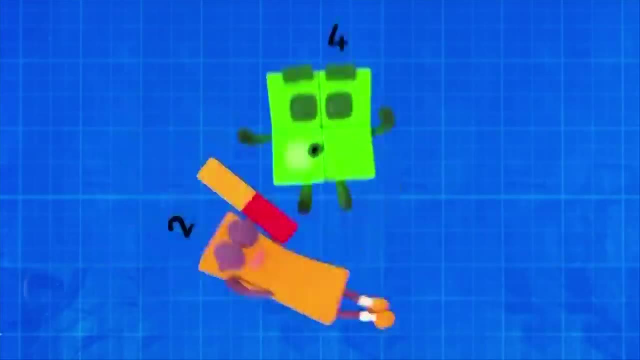 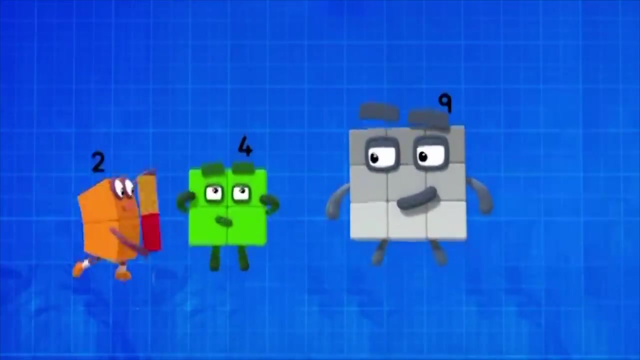 And 2 from side to side. I'm the same in both directions. I'm as tall as I am wide. That's why I'm square. like you, I'm 3 by 3, I'm 2 by 2. That's why I'm square. 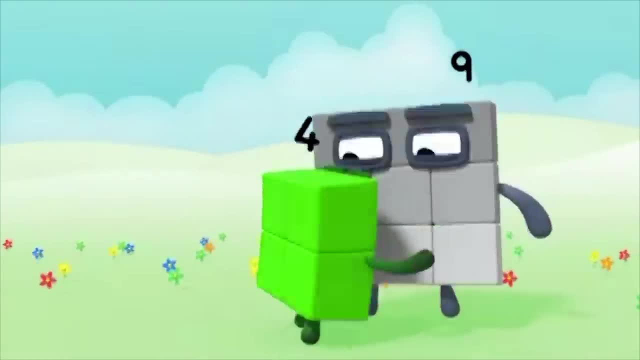 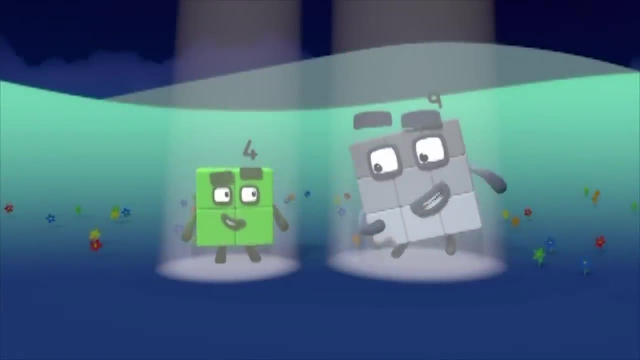 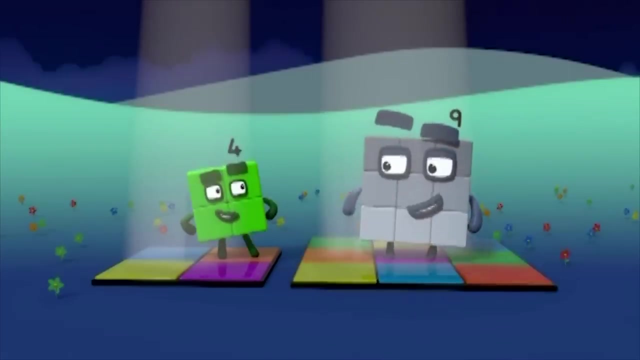 Achoo, Yes, I am square like you. I'm 3 by 3, you're 2 by 2. I'm 2 by 2, you're 3 by 3. That's why you're square. That's why you're square. 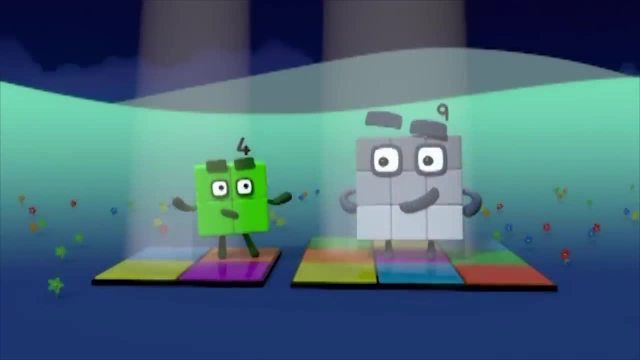 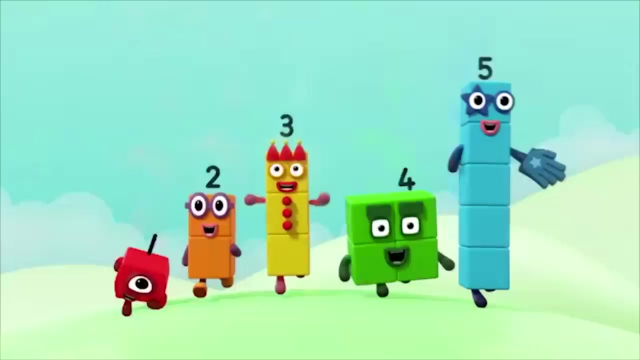 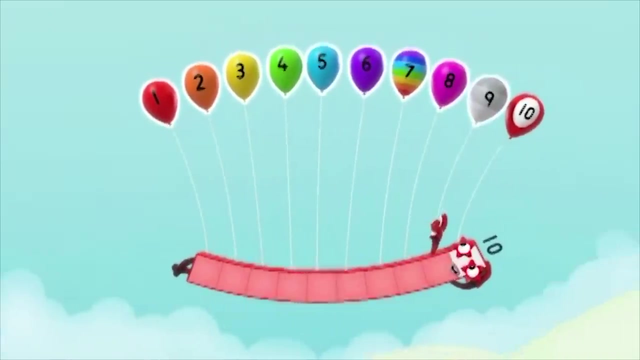 That's why you're square Like me. 1, 2,, 3, 4. 1, 2,, 3, 4, 5, 6,, 7,, 8, 9!. Squares 1, 2,, 3,, 4,, 5, 6, 7,, 8,, 9,, 10!. 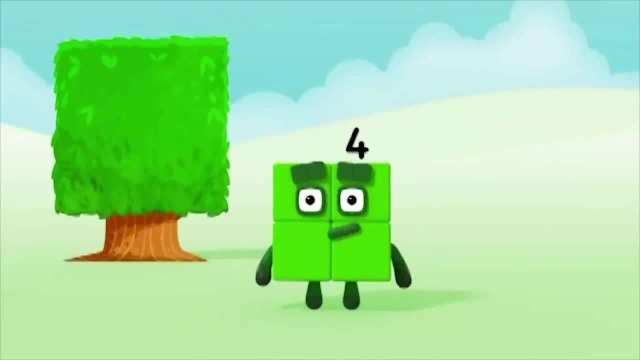 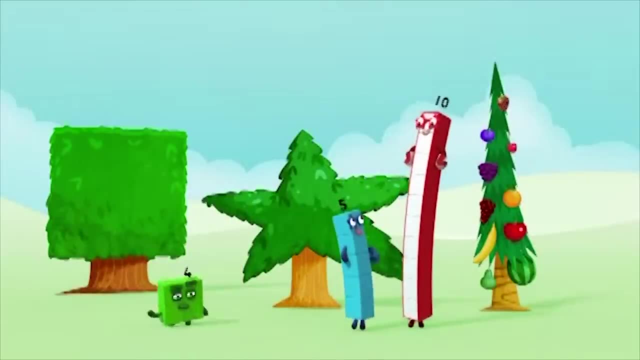 4 is made of 4 blocks. I love to be a square. 5 is made of 5 blocks. High five There. I'm there. I'm 4 ones And I'm 5 ones And I'm 10 ones, which means 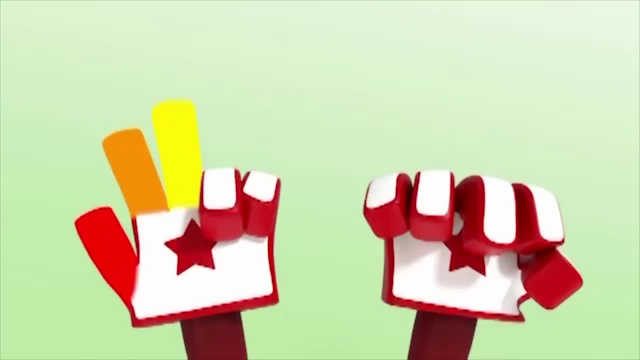 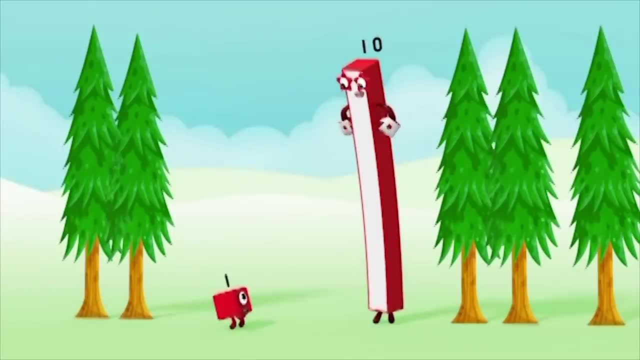 I'm 1 ten: 1,, 2,, 3,, 4,, 5,, 6,, 7,, 8,, 9,, 10!. Oh, why have you got that round thing next to your 1?? 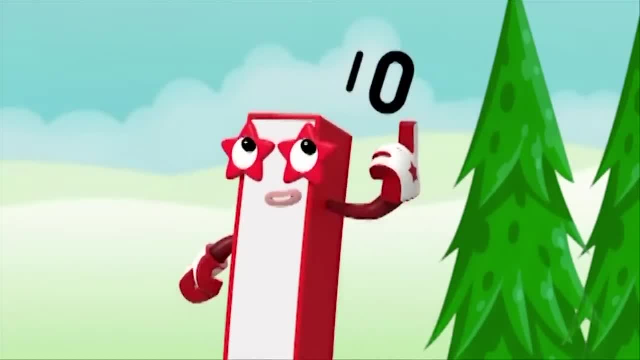 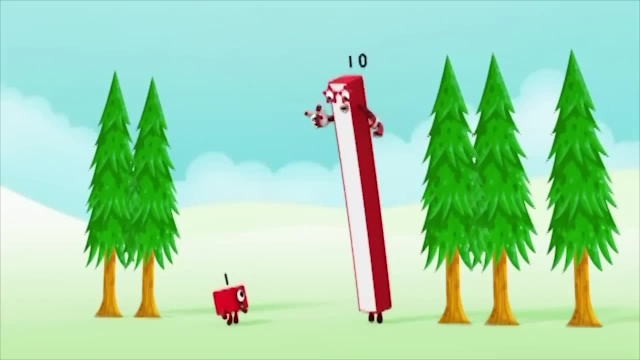 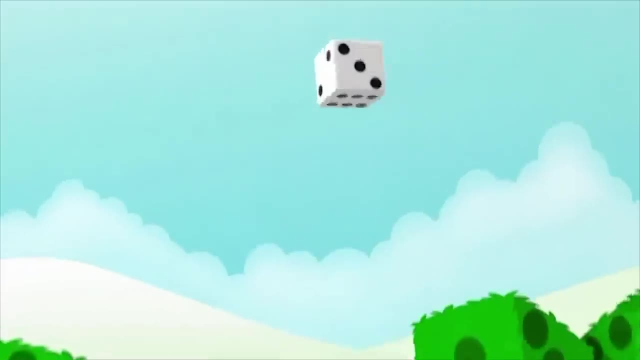 It's a zero. I need my zero hovering in space. It's there to keep my 1 in place And if you're wondering what it's for, It shows you I'm not 1, I'm 1 ten and nothing more. 6 is made of 6 blocks. 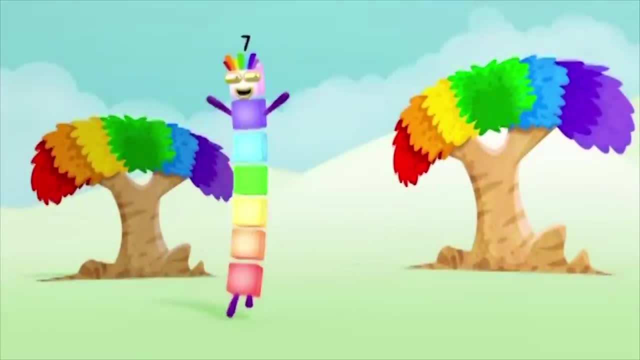 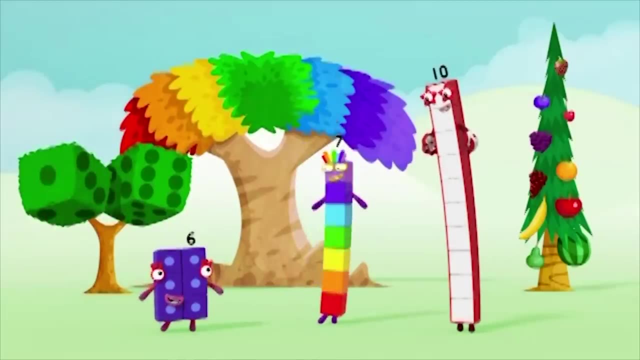 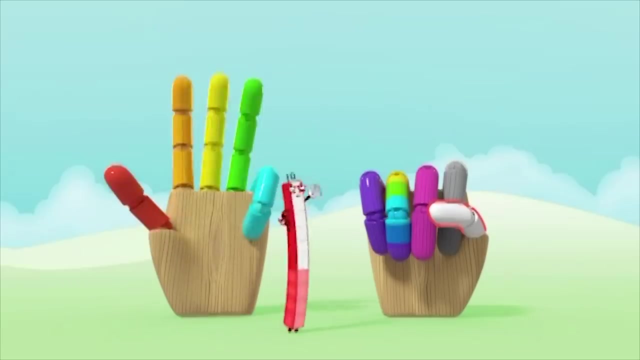 I like to roll the dice 7's made of 7 In a rainbow. That looks nice. I'm 6 ones, I'm 7 ones And I'm 10 ones, which means I'm 1, ten, 1, 2,, 3,, 4,, 5,, 6,, 7,, 8,, 9,, 10!. 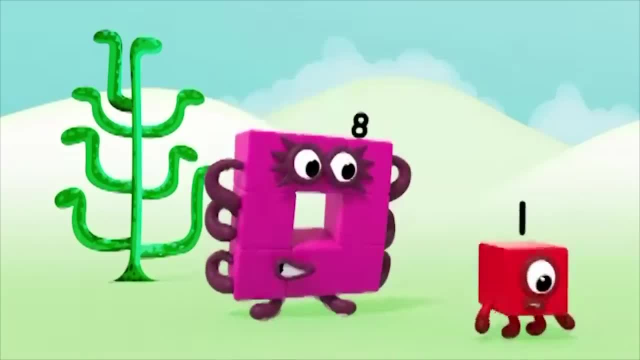 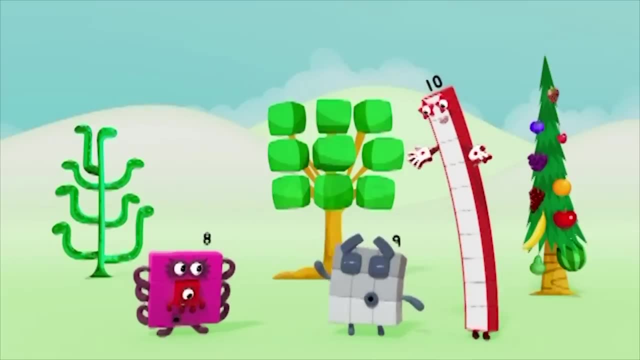 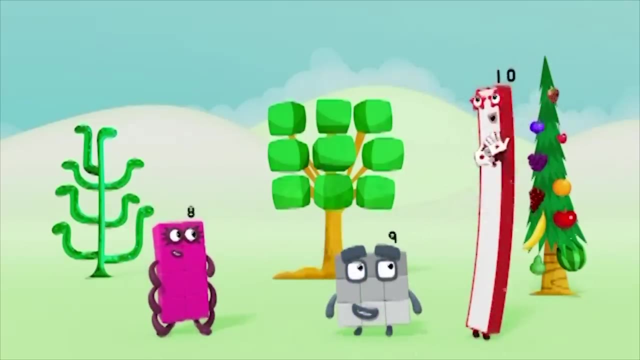 8 is made of octoblocks And if you add one more, 9 is made of 9 blocks. I'm a bigger square than 4, I'm 8 ones And I'm 9 ones And I'm 10 ones, which means I'm 1 ten. 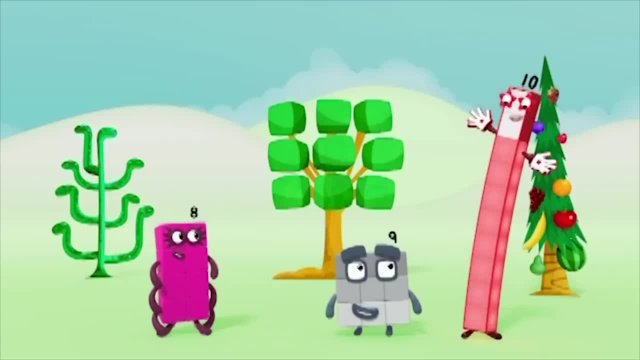 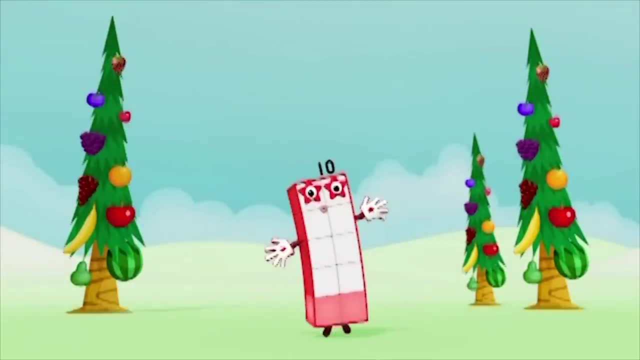 1, 2,, 3,, 4,, 5,, 6,, 7,, 8,, 9,, 10!. I can be 2 lots of 5, Or 5 lots of 2, In other words 5 pairs. 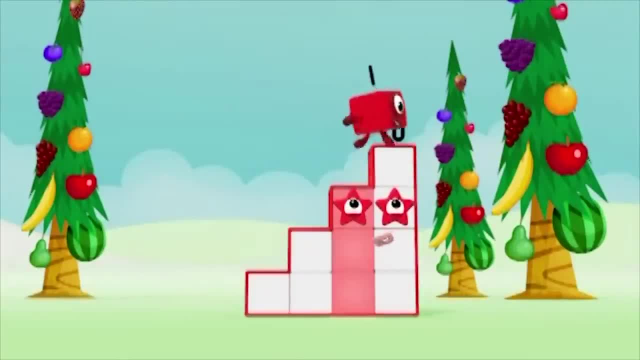 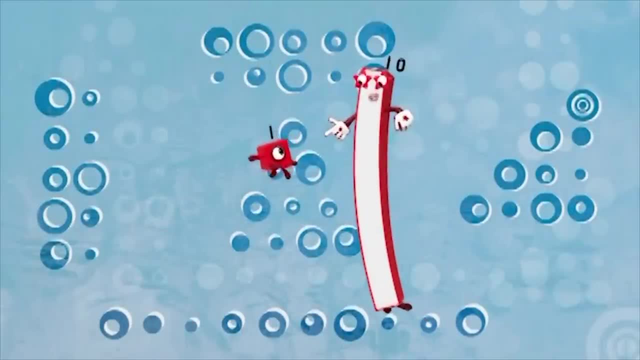 I can be 1 and 2 and 3 and 4 When you need to go upstairs. I'm a 10 block. I'm a 10 block. You might think we're different. Think again. They're all just made of counting blocks. You're 1 one. 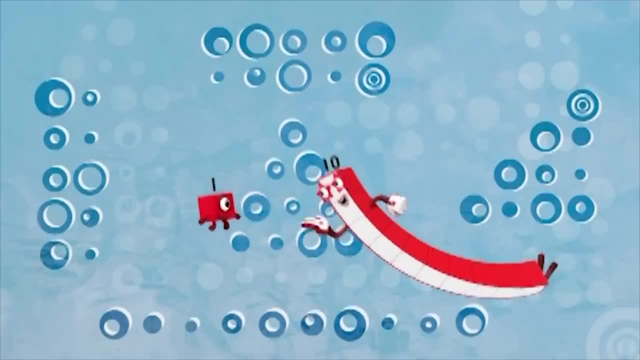 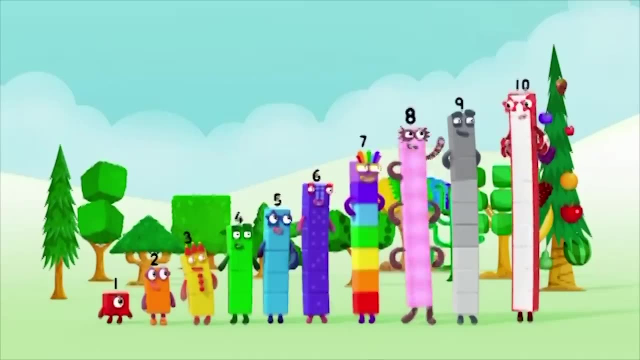 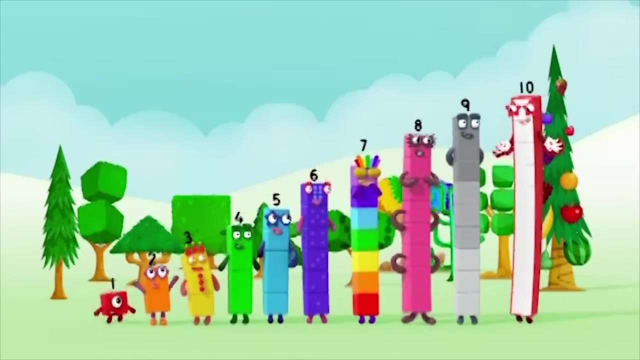 And you're 10 ones, Which means I'm 1 ten, 1,, 2,, 3,, 4,, 5,, 6,, 7,, 8,, 9,, 10!. You can count on us with another box. 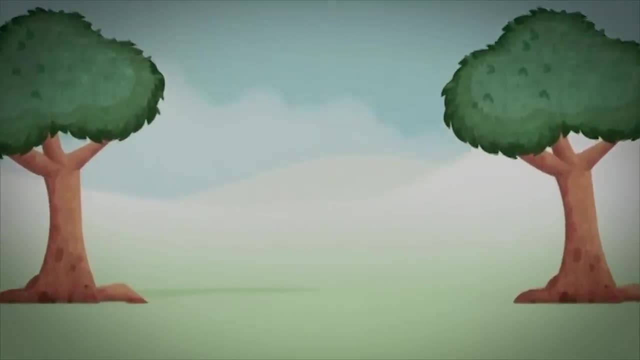 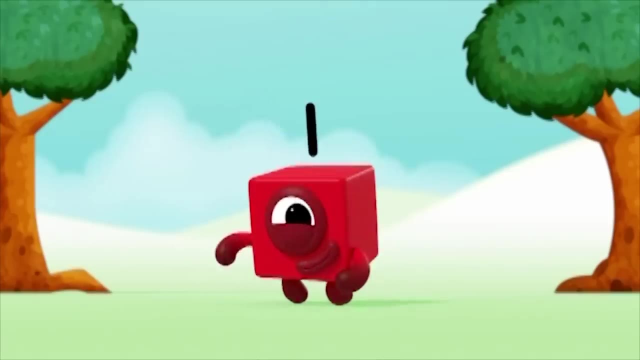 If there's nothing going on, No one's there and it's no fun. You can get the party started With a bang by adding 1!. I am 1 And I'm playing in the sun. Being 1 is my idea of fun. 1!. 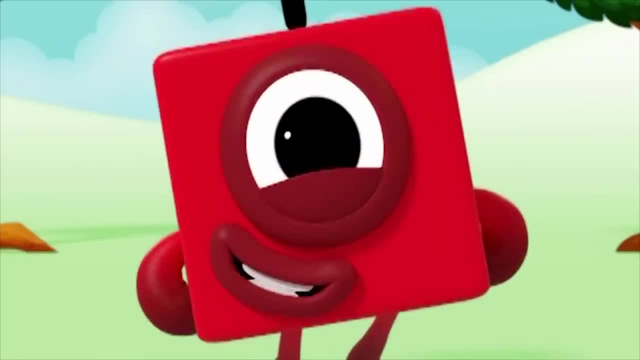 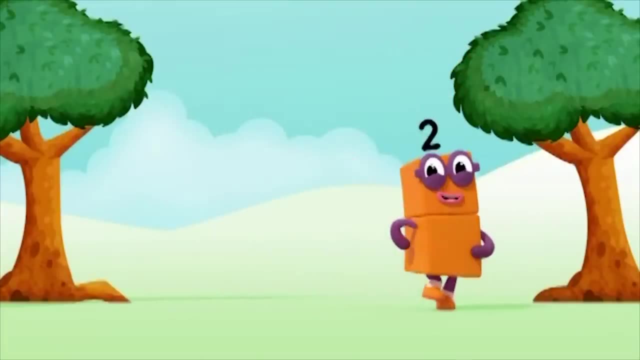 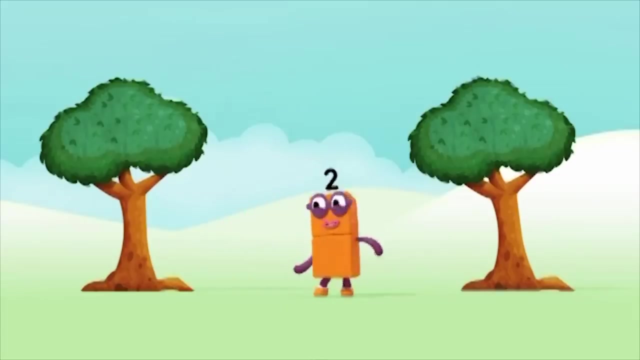 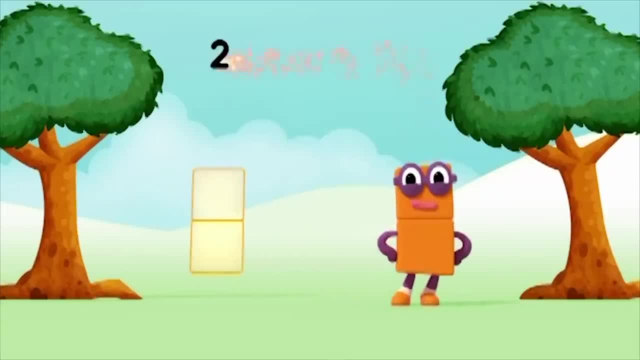 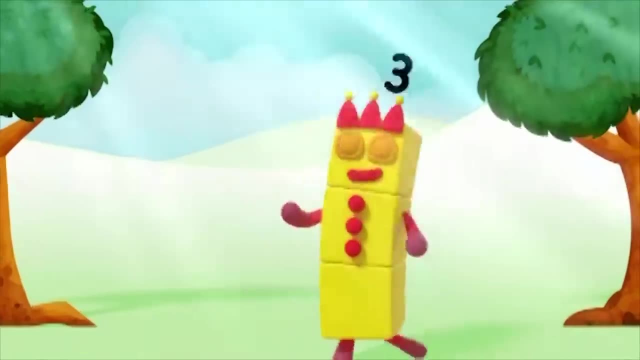 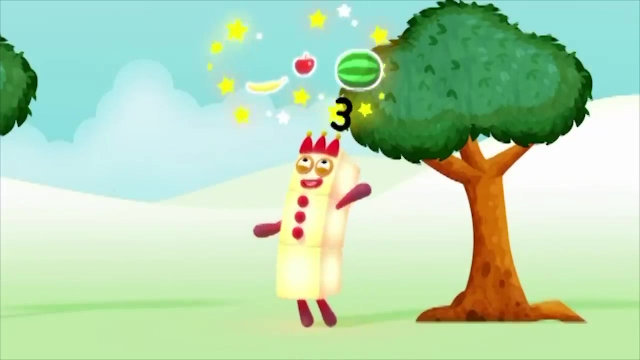 Now let's add another 1. 2 plus 1 equals 3!. I am 3 And I'm playing in the sun. Juggling things Is my idea of fun. 1, 2, 3! 3 things. Look at me. 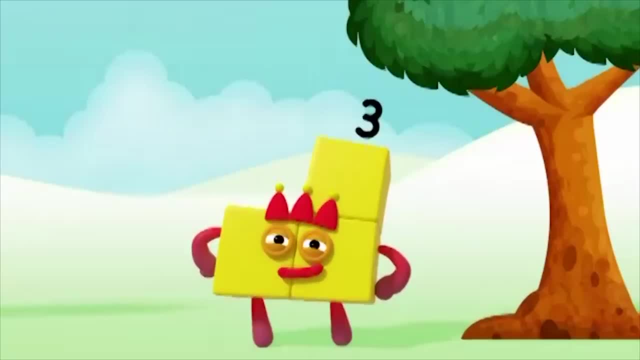 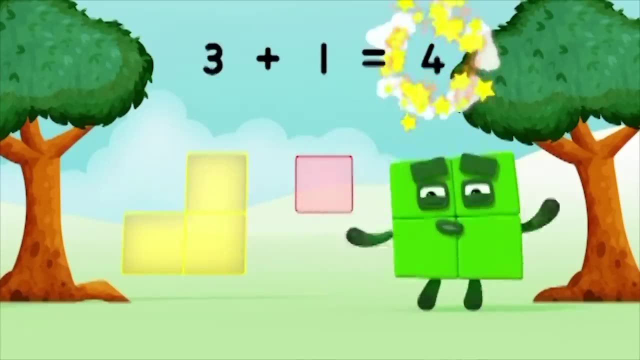 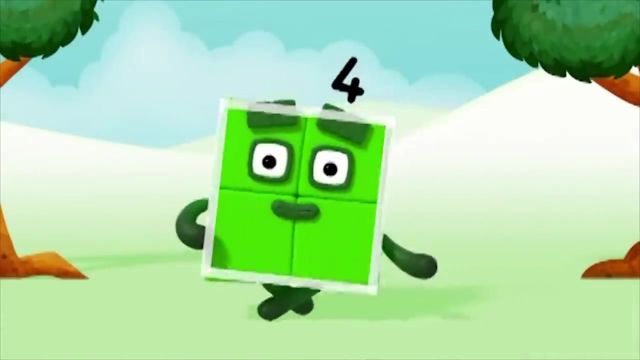 1,, 2,, 3!. Now let's add another 1!. 3 plus 1 equals 4!. I am 4 And I'm playing in the sun. Being square Is my idea of fun. 1,, 2,, 3,, 4!. 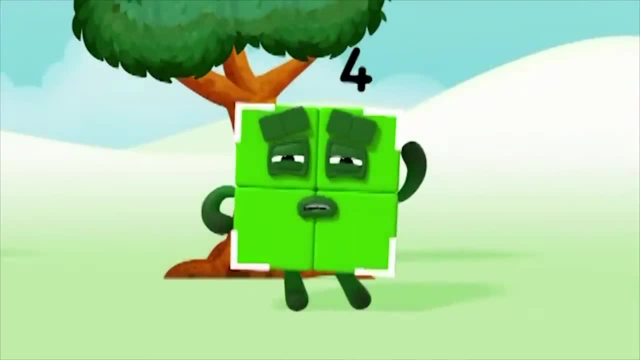 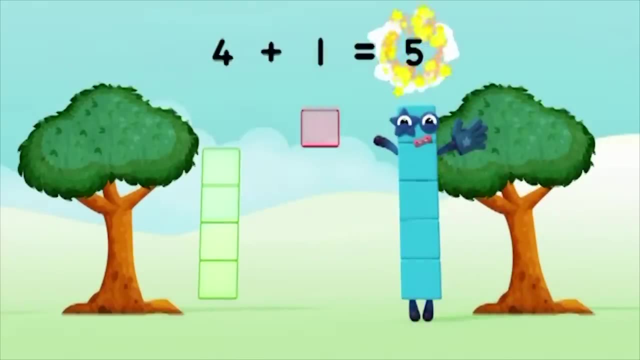 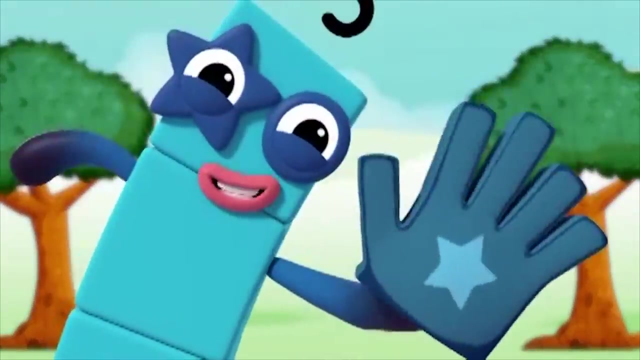 4 sides. Out, Out, Out, Out. 4 corners. Now let's add another 1!. 4 plus 1 equals 5!. I am 5 And I'm playing in the sun. High-fives Are my idea of fun. 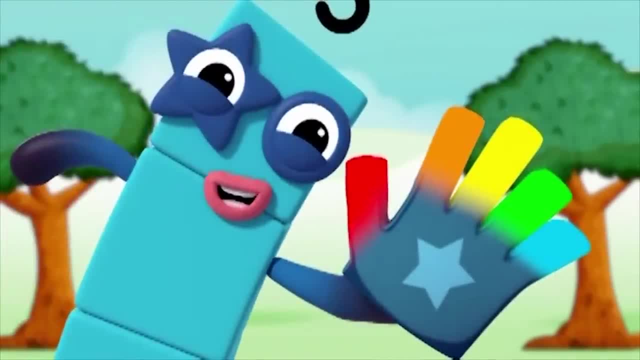 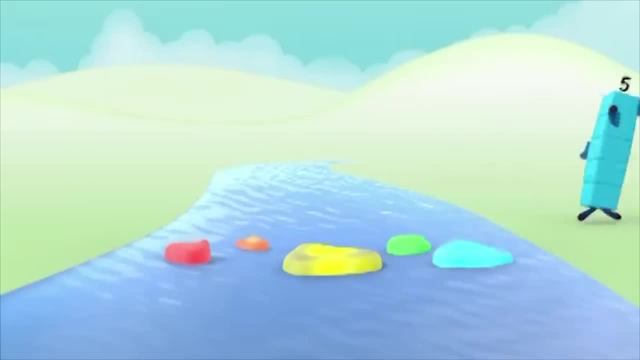 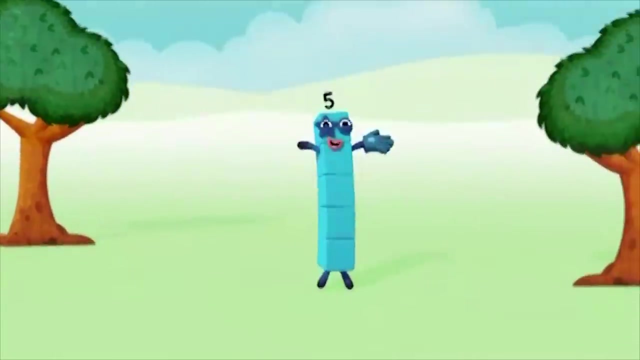 1,, 2,, 3,, 4, 5! 5 fingers. If you add another 1, The number gets one bigger, And if you keep on adding 1 You can get to any bigger. You can count on us with an Octobox. 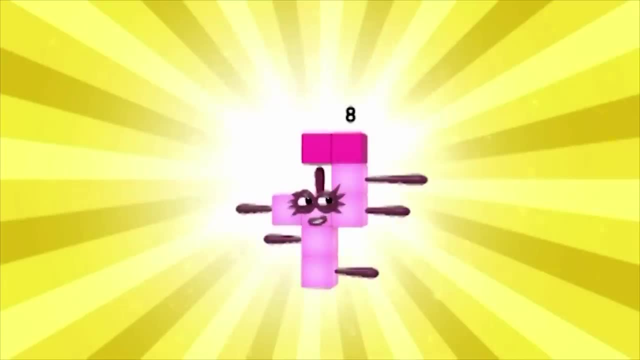 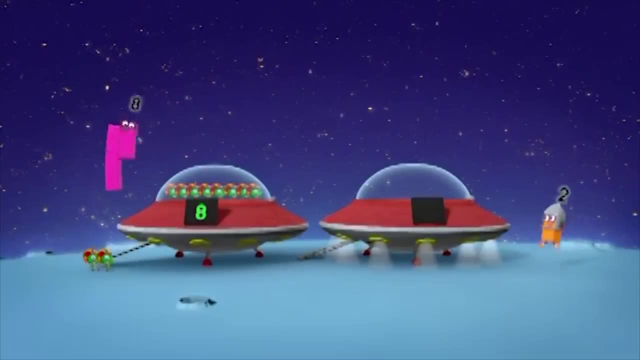 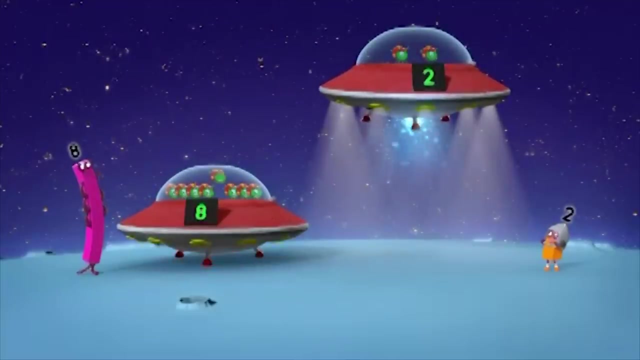 Octoblock- build 1,, 2,, 3,, 4,, 5,, 6,, 7,, 8. Build 2: flying saucers. Good work, I can't lay my hands to theeln anyway. I don't believe in ants any more. 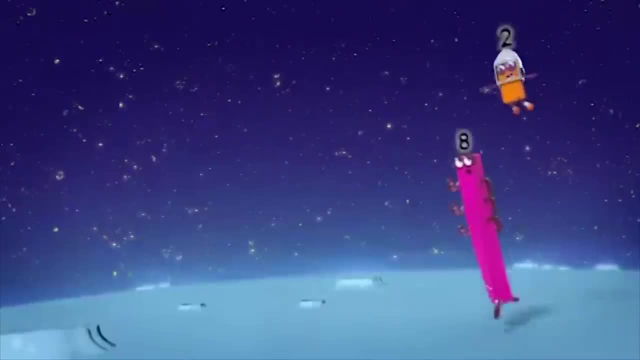 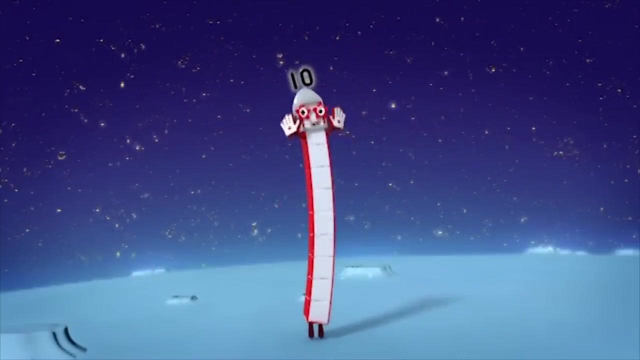 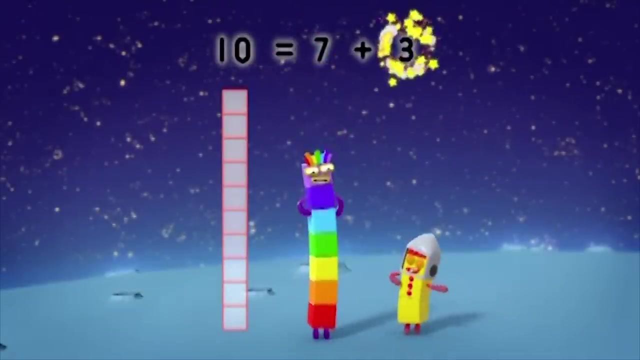 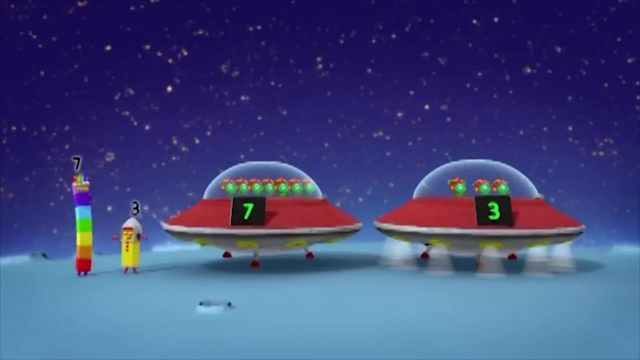 10!, It's 7! 10涉. 10涉 is a camera. Let's roll. 母亲, Who says that на Come back, It's not starting. Oh, We're so lucky. Look at me, Woohoo. 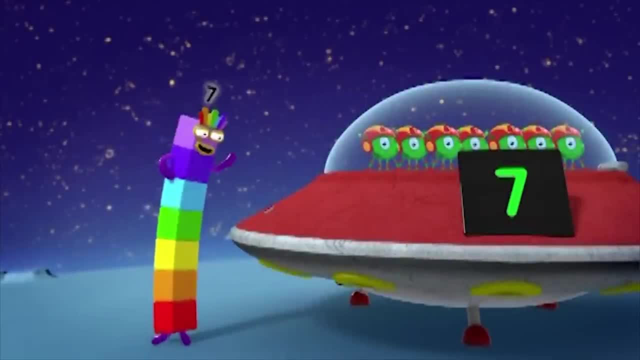 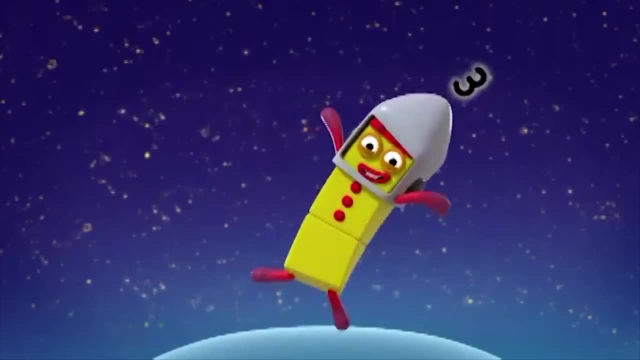 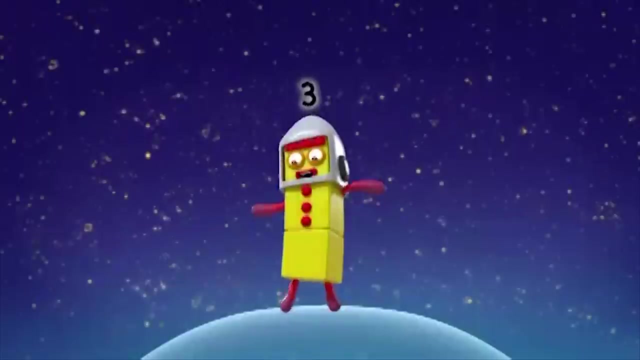 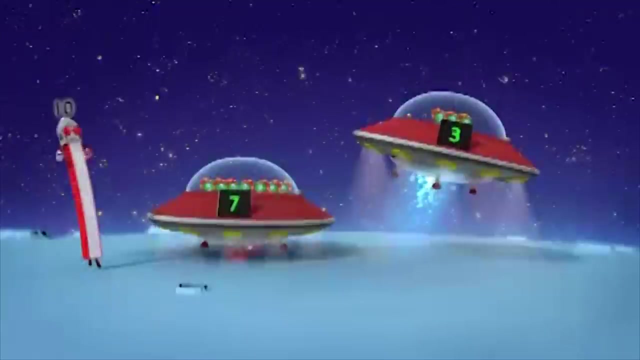 Look at that. There's the on button. That was lucky, Ready, steady, Blast off, It's too heavy. Seven plus three equals ten. It's ten again. Wait and see who my next two friends will be Ten equals. 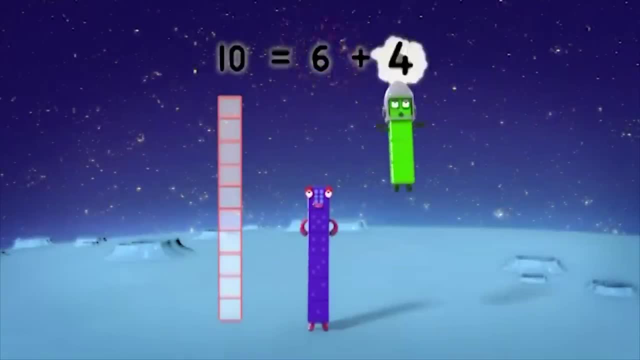 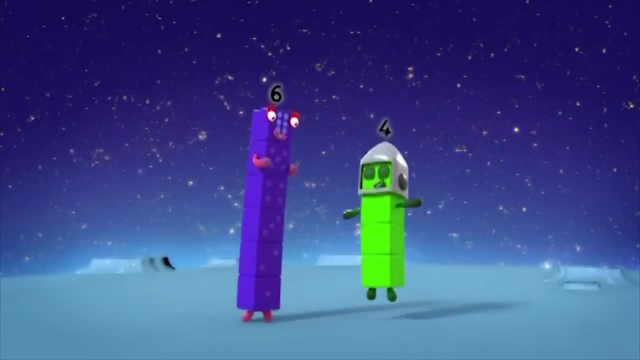 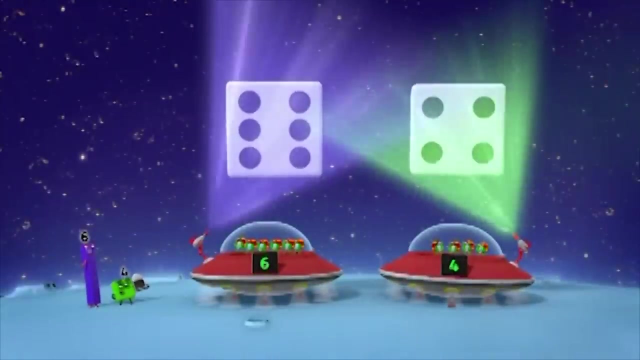 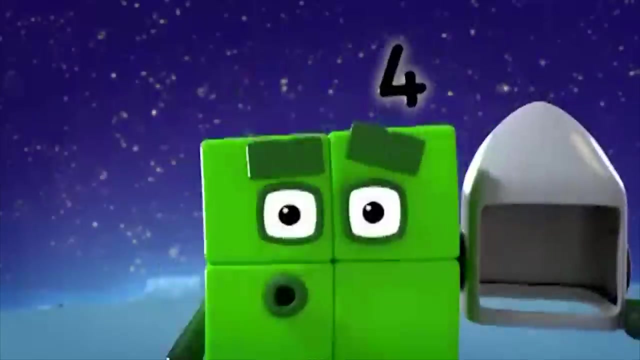 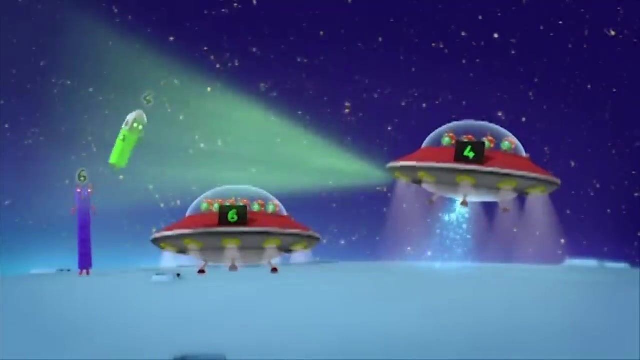 Six plus four, We're on the moon. Six and four. We really couldn't ask for more. Let's play a game, Roll the dice and Woohoo. Oh, Oh, That was so cool, Still too heavy Six. 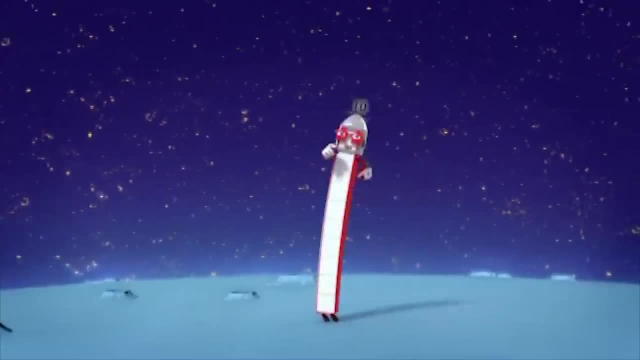 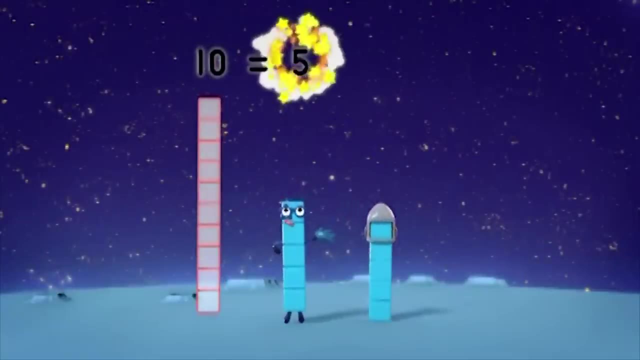 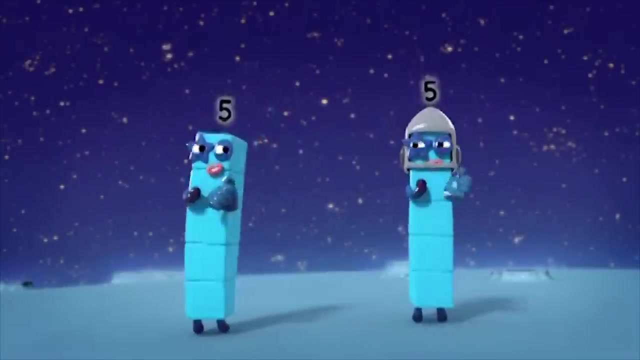 Plus four equals ten. Quick, before our visit ends, We've just got time for two more friends. Ten equals Five plus five. We're on the moon. Five and five. It sure feels great To be alive, to be alive. 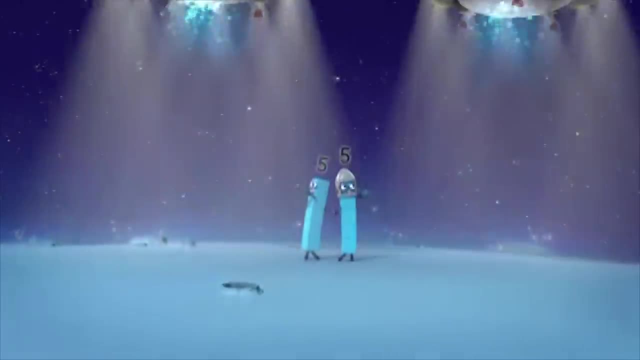 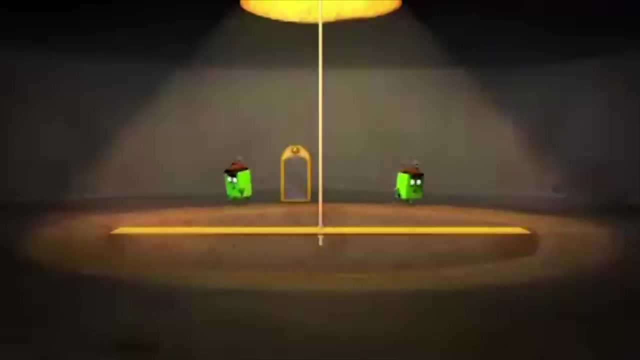 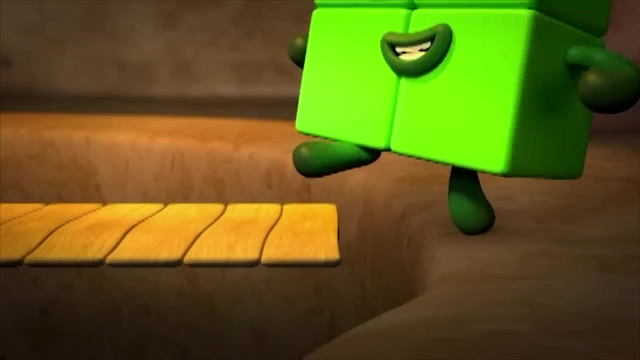 Let's give them a hand. High five. You can count on us With an OtterBox. You can count on us With an OtterBox. With an OtterBox. One, Two, Three, Four, Now One. 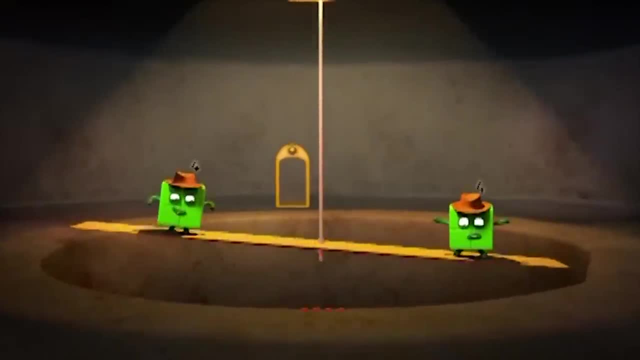 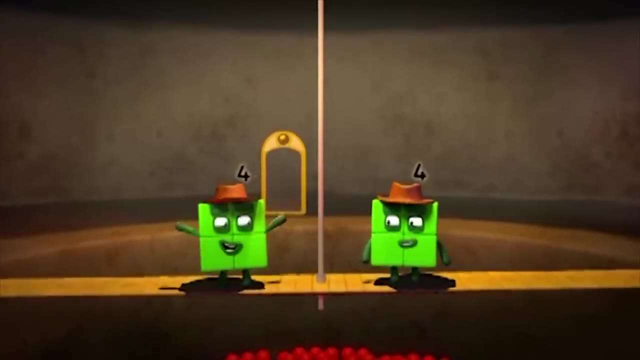 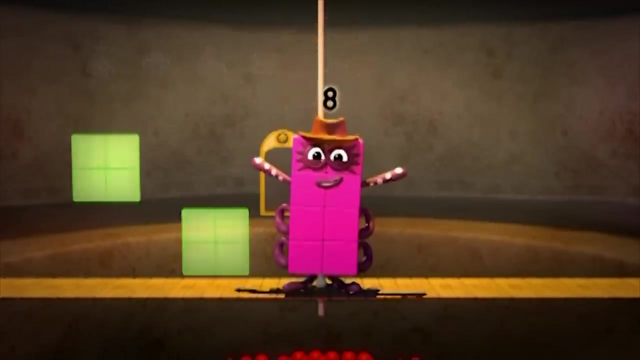 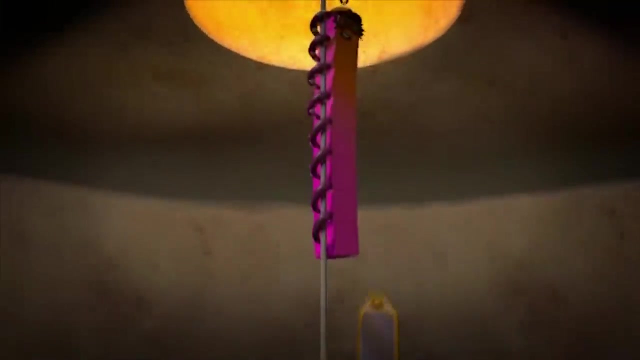 Two, Three, Four. Now Keep going, Keep going And double up. Four plus four equals eight. Octoblock climb One, two, three, four, five, six, seven, eight. Climb The Golden Delicious. 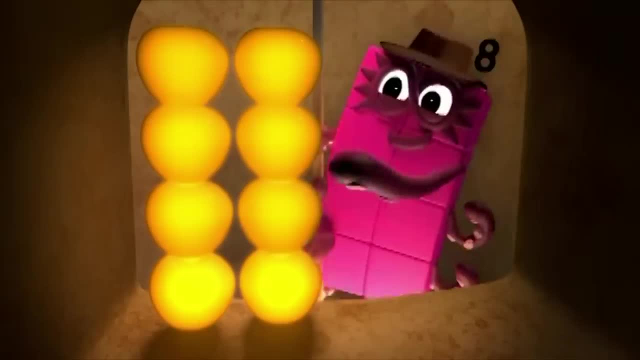 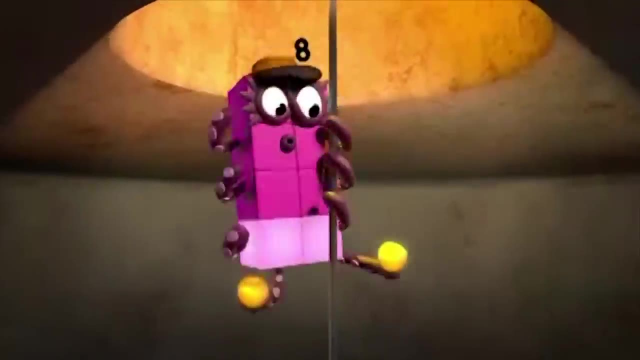 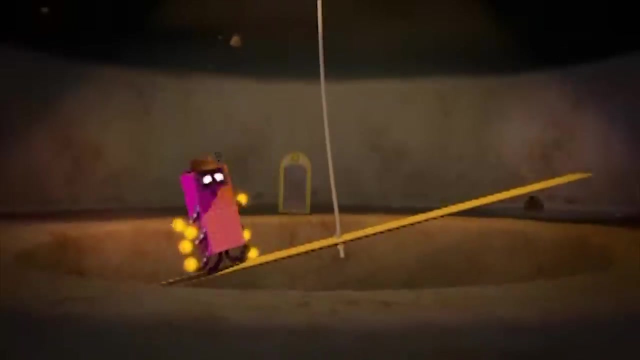 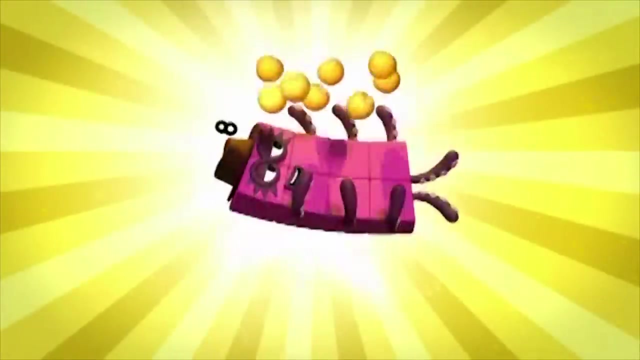 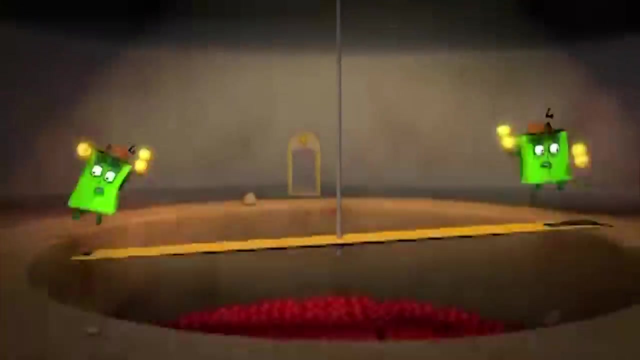 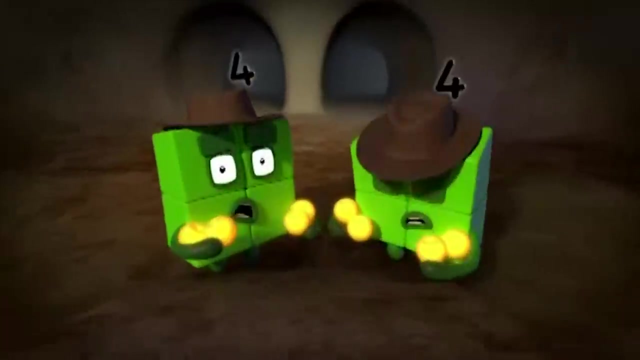 Mmm. One whoops Time for a quick exit. Two, three, Two, three, four, five, six, seven, eight. Octoblock splits in half. Eight equals Four plus four. Giant brown thingamabob. 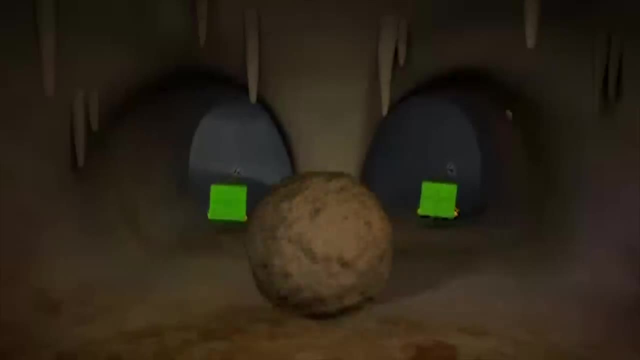 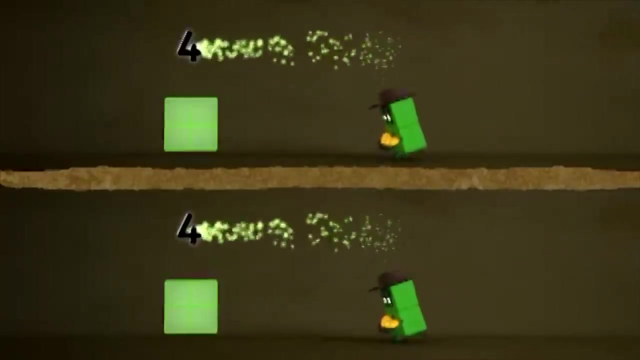 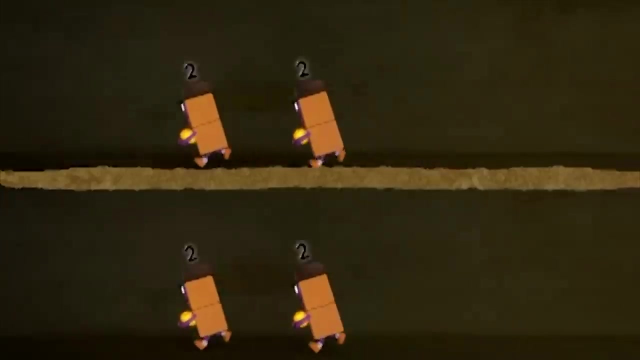 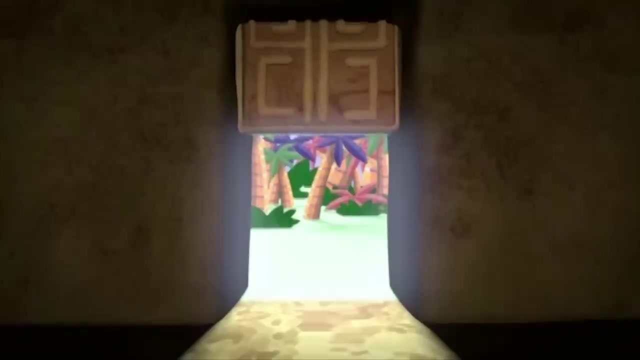 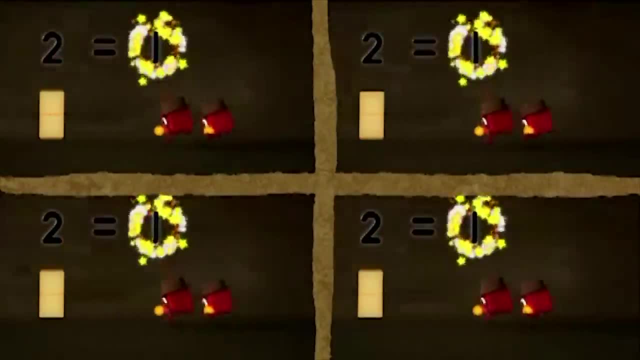 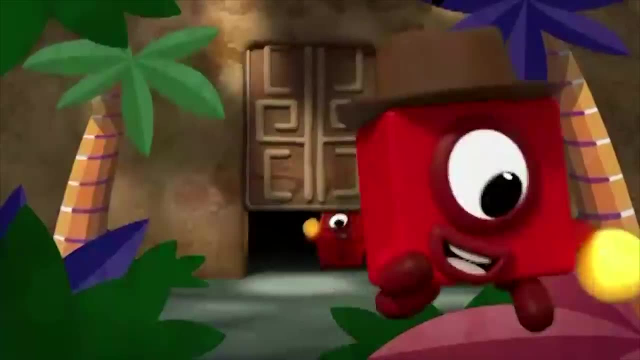 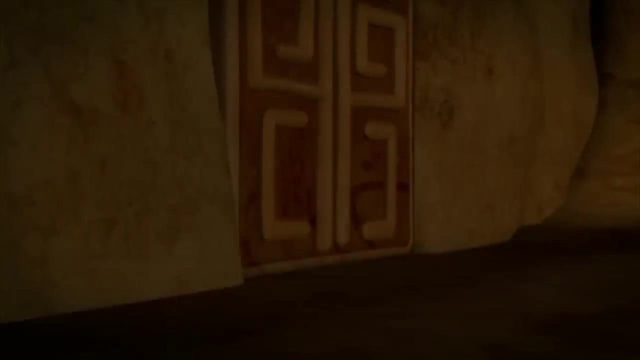 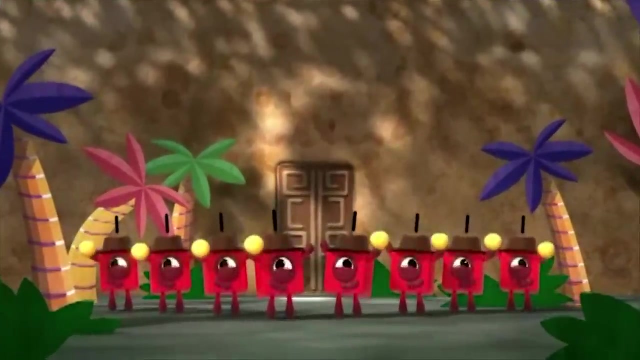 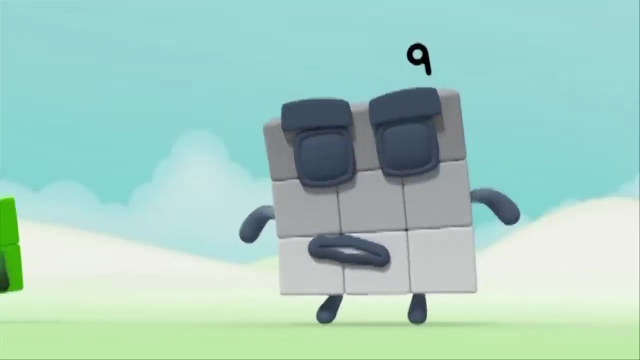 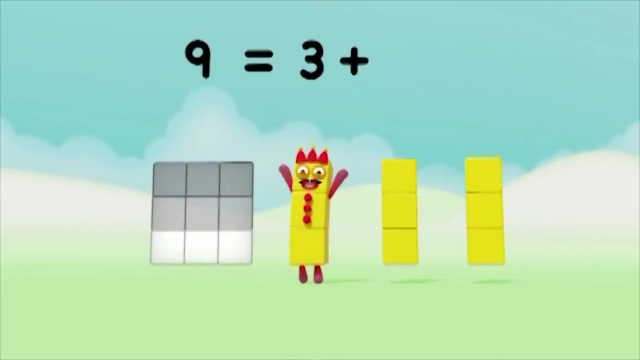 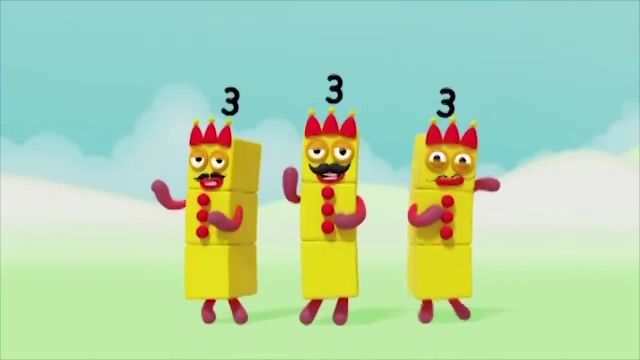 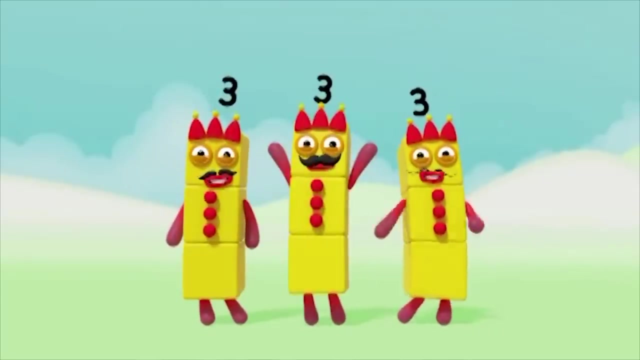 Split it in half. You can count on us. we're the number one. Nine equals three plus three plus three. roll up, roll up, roll up. we three are the three threes The most amazing, the most incredible, the most extraordinary acrobats in Numberland. 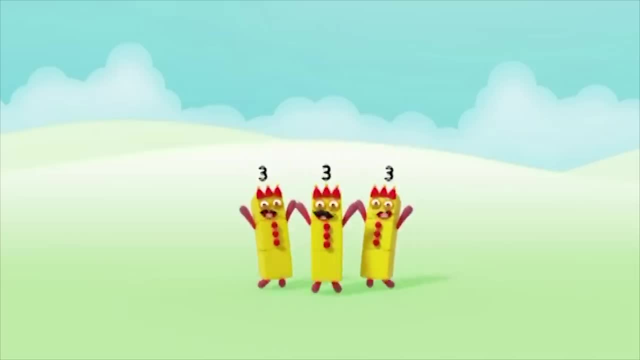 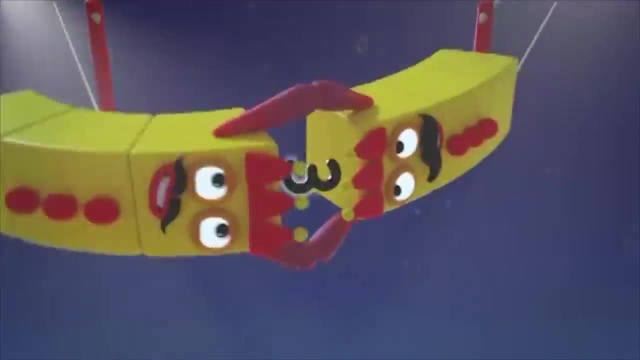 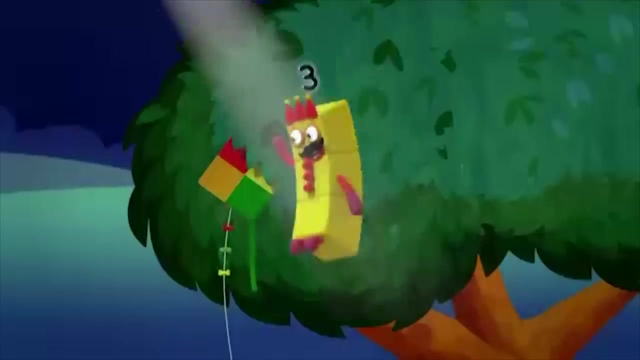 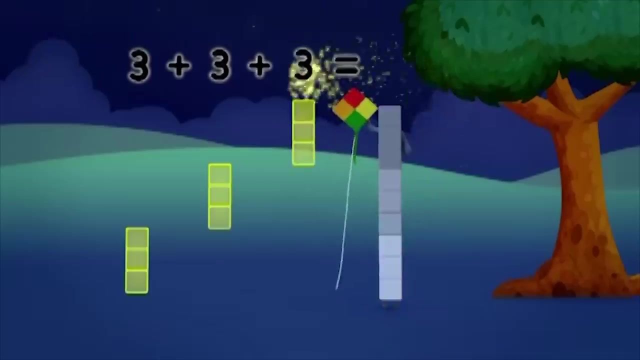 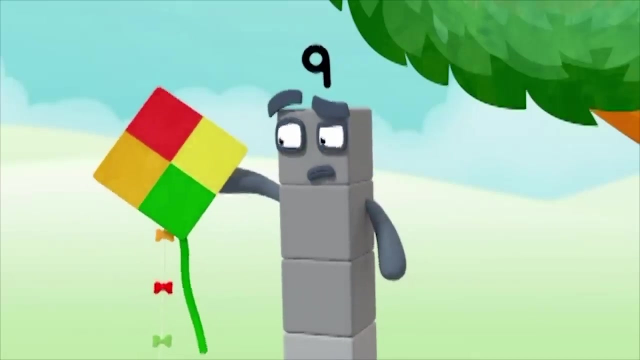 Drum roll please, As we present Number One, The three threes On the Flying Trapeze, Hooray. Three plus three plus three equals Nine, Nine. You did it, Did what? Oh, It was nothing really. 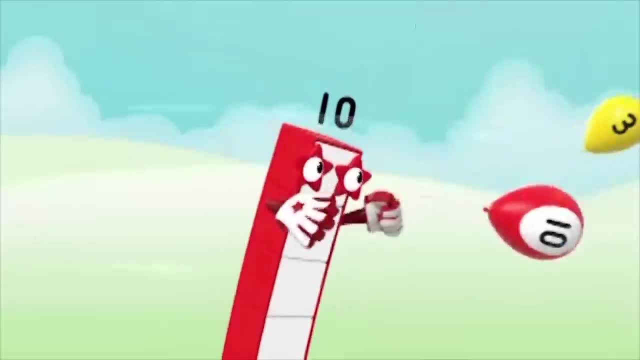 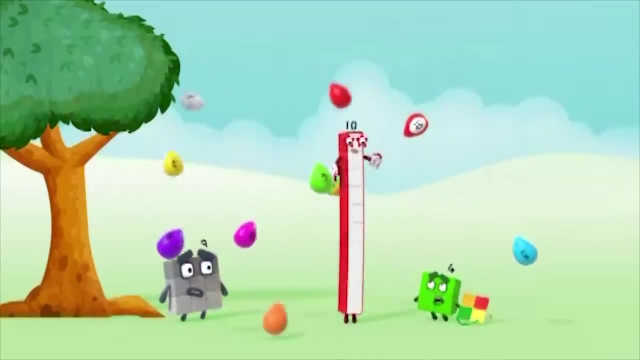 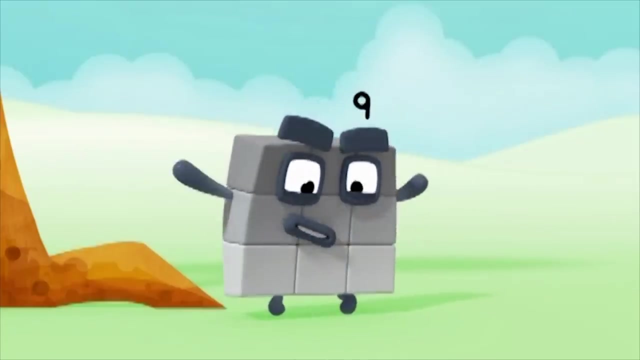 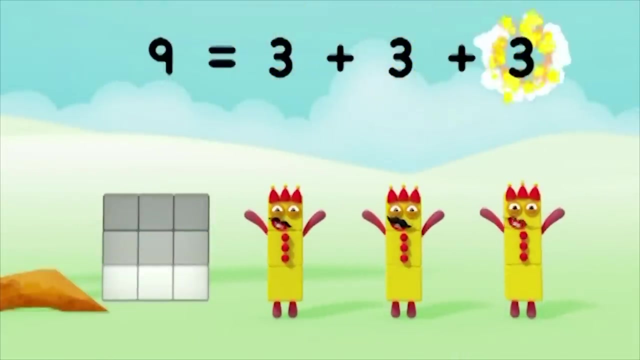 Quick stop them. Oh, There are too many. We need help. Help, I can do this myself. Nine equals three. Pull us three, Pull us three. The three threes will seize these with great ease. Drum roll please. 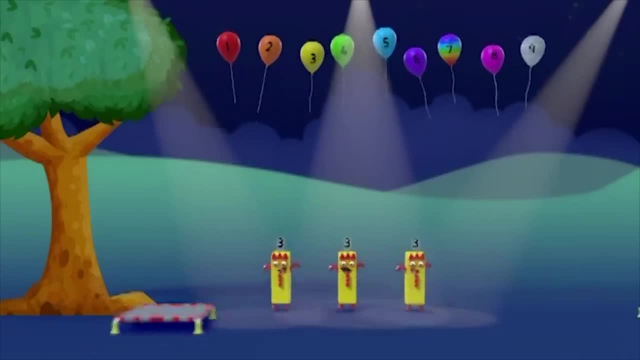 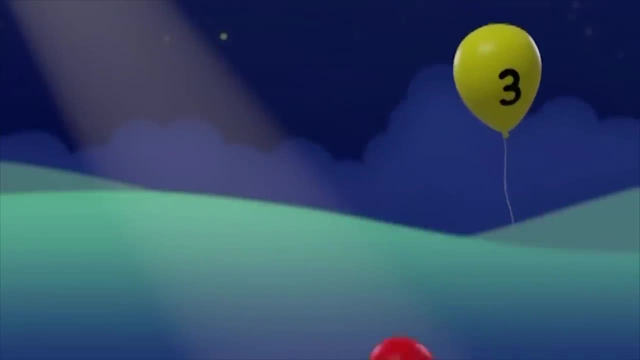 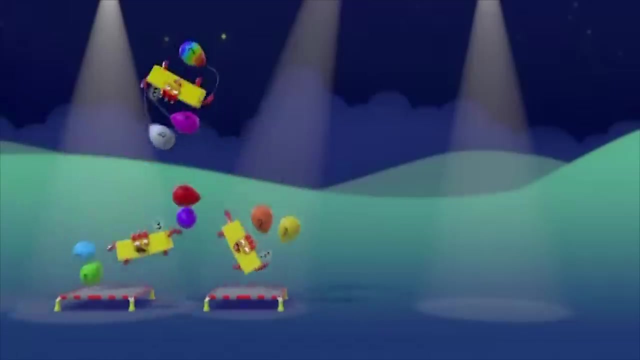 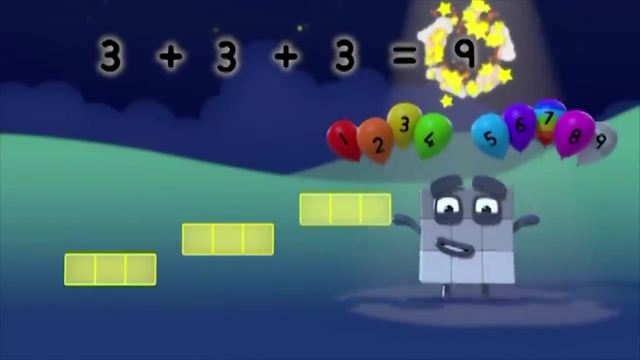 One, Two, Three, Four, Five, Six, Seven, Eight, Nine. One, Two, Three, Four, Five, Six, Seven, Eight Nine. One, Two, Three, Pull us three. Pull us three, Equals nine. 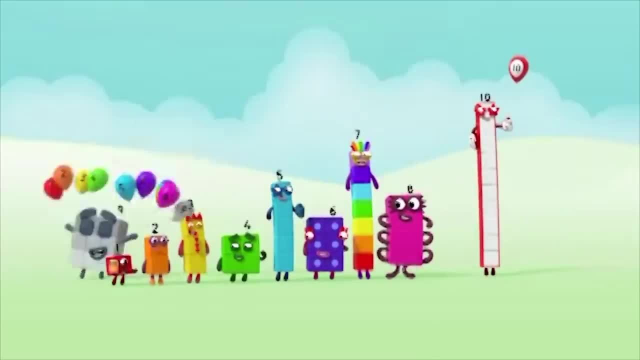 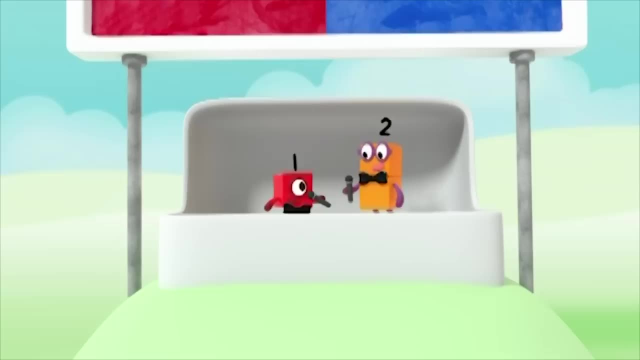 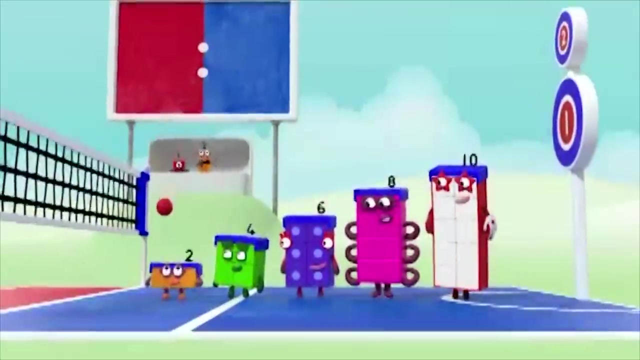 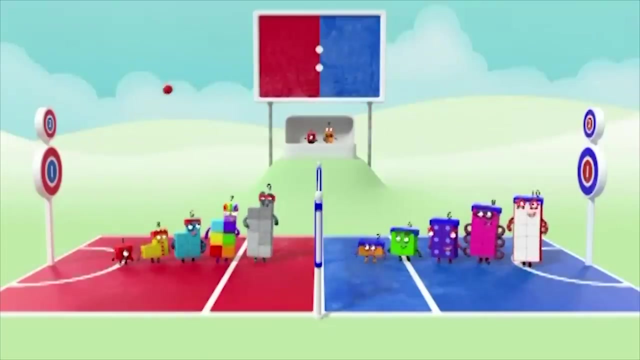 You did it again. I did, Of course I did. Let's play basketball. After a great start, the ball is with the even tops And it's two, four, six, eight, ten. A great shot, my ten. 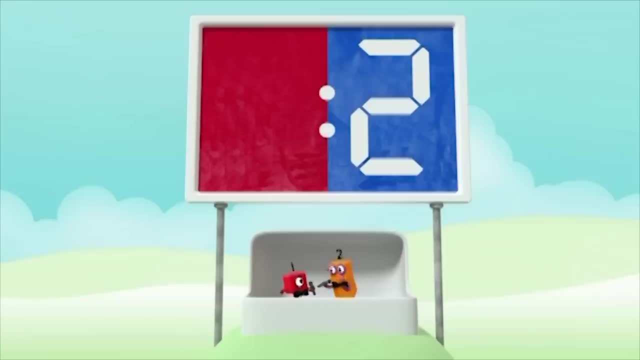 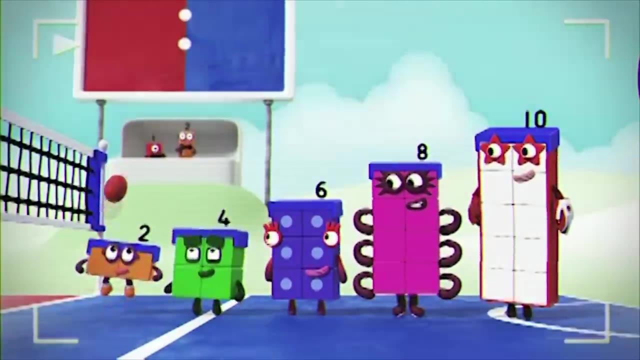 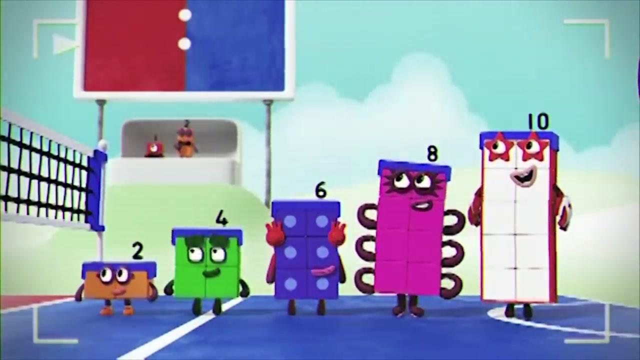 Two points to the evens. Now let's see that again in slow motion MUSIC. Look at that. Two, Two, lots of two, Three, lots of two. In fact, each of the evens is two more than the one before. Let's see what the odd box can do. 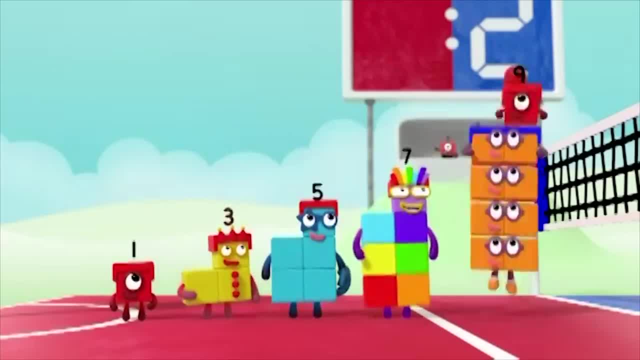 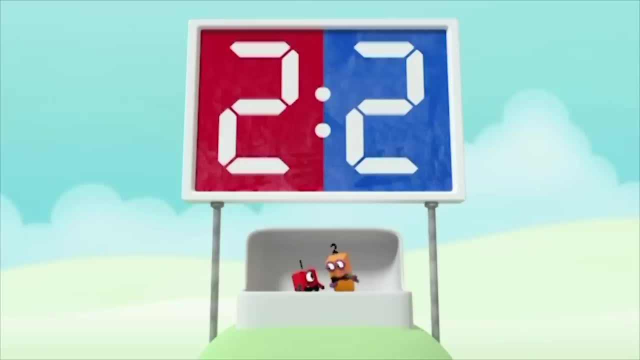 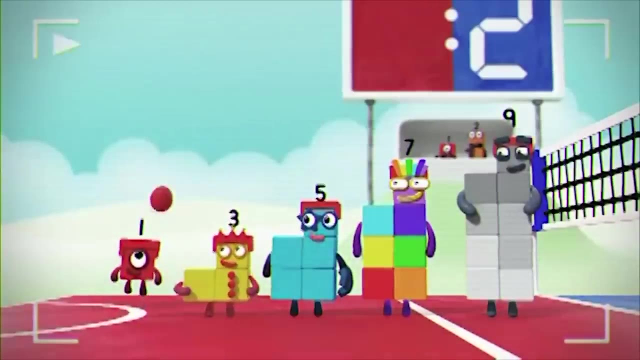 One, Three, Five, Seven, Nine, Amazing Two points to the odds. That makes the score two. all It started with one And there she is again on top of two, Making three, And again on two, twos. 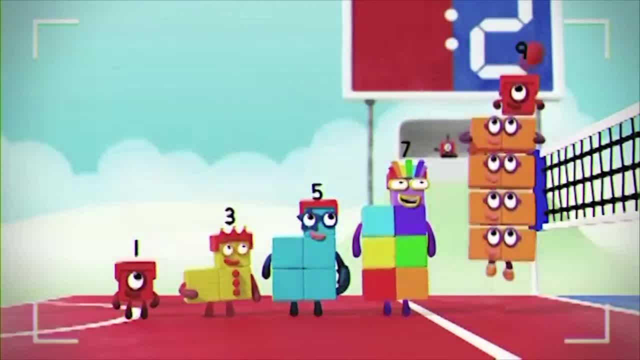 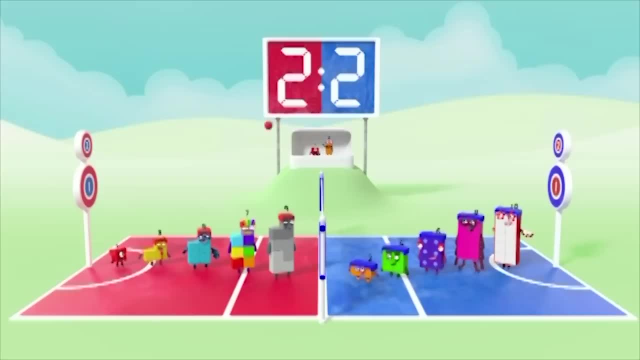 Look Each of the odds. The odds is two more than the one before, with an odd one sticking out on top With the score level. it's all to play for. What can they do now? Two, four, six, eight, ten. 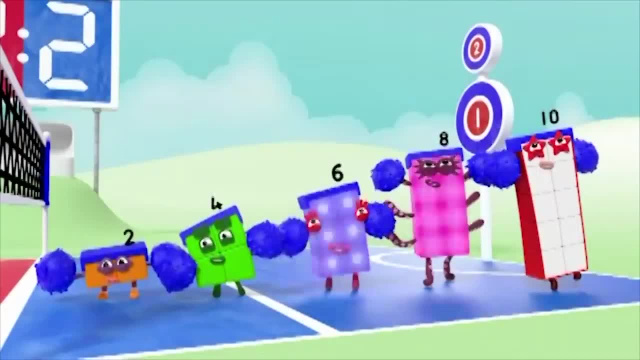 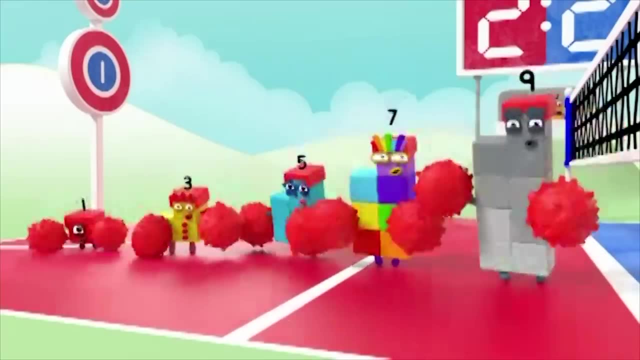 Come on, even score again. Ten, eight, six, four, two. That's what even numbers do. One, three, five, seven, nine. We are odd and we feel fine. Five, nine, seven, five, three, one. 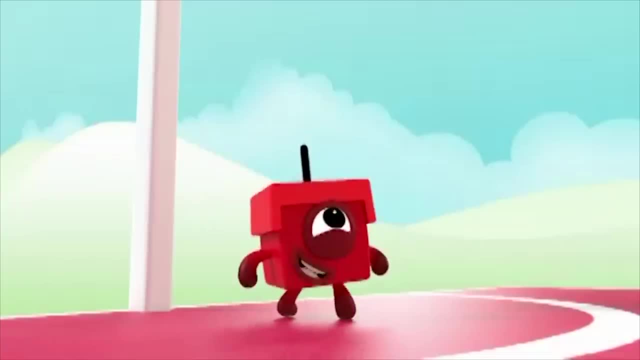 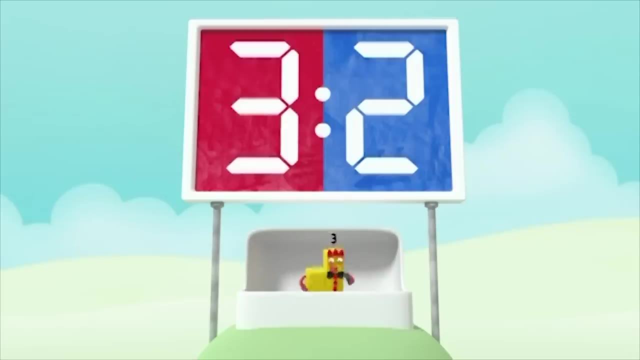 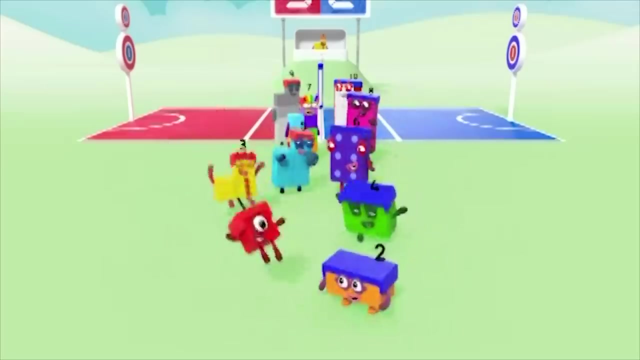 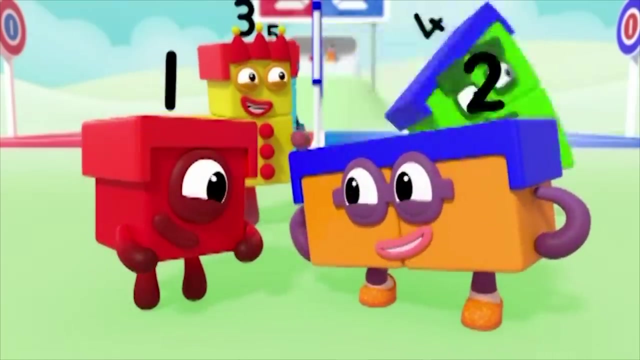 Odds are having so much fun. The odd blocks beat the even tops by a magnificent three points to two. Yay, What can I say? Even we couldn't beat the odds. Well, if you can't beat them, Join them, Join them. 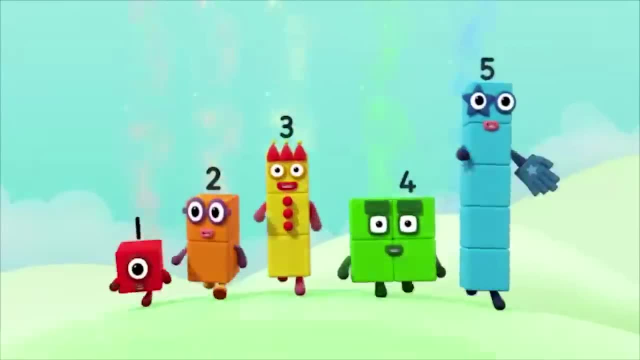 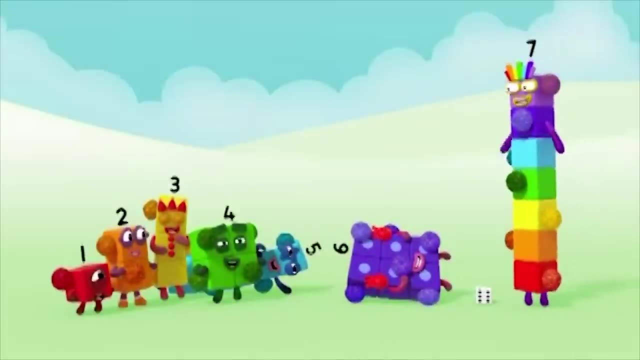 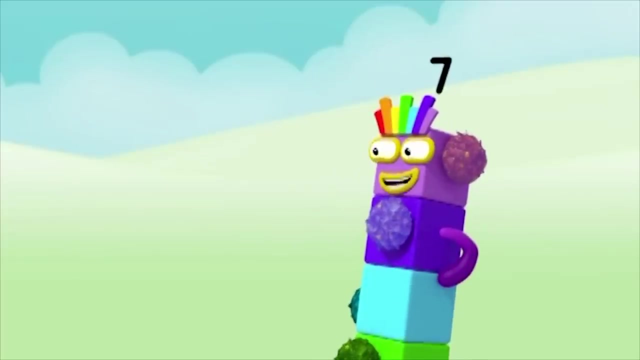 You can count on us, we're the Nodderblocks. Sevens are not ticklish. How lucky is that. Oh, have you all had enough tickling? Why don't you just make sevens? then How I'll show you. 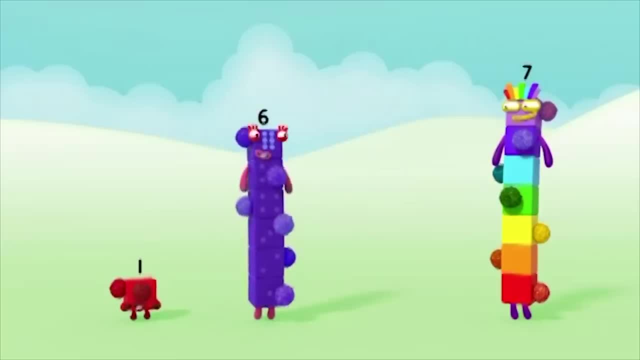 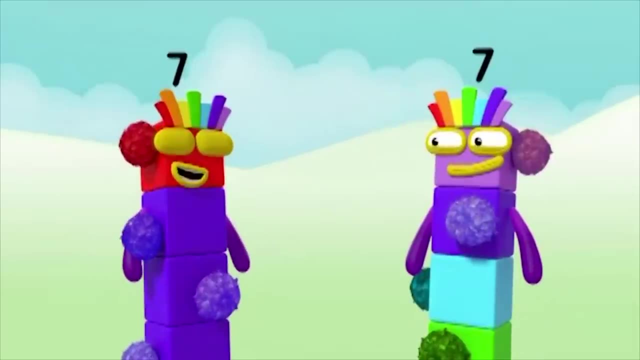 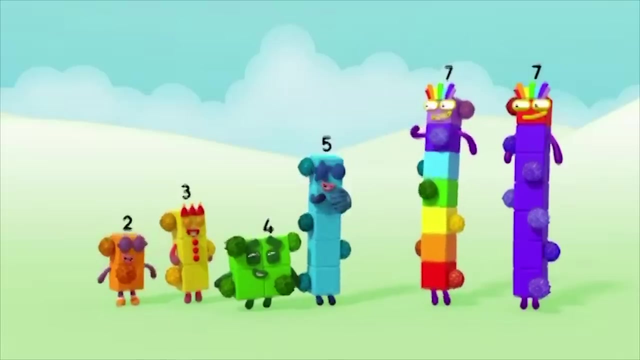 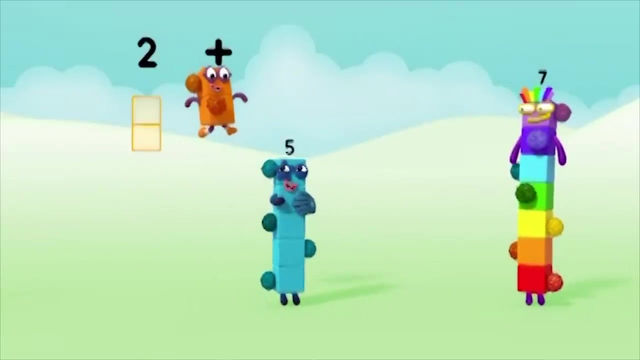 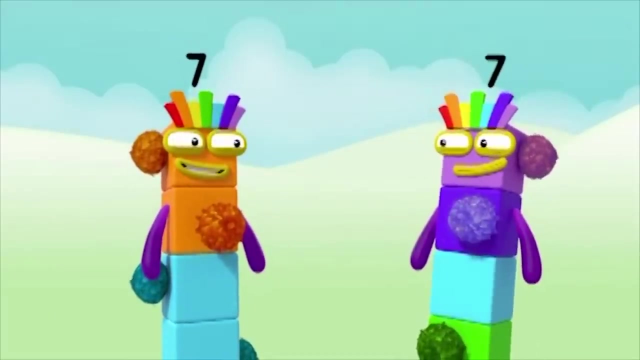 One and six. One plus six. One plus six Equals seven. Oh, That's better, Pick me Blue blue, blue, blue blue. Two and five. Two plus five Equals seven. That's better. Three and four. 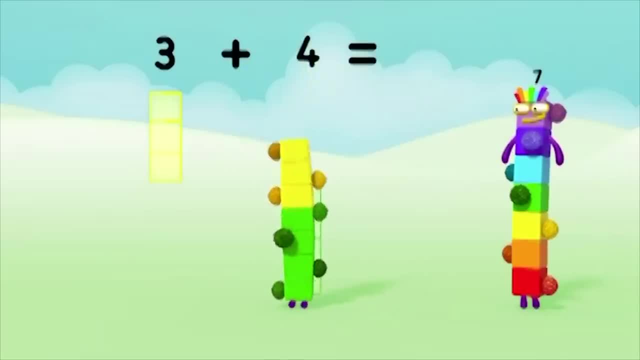 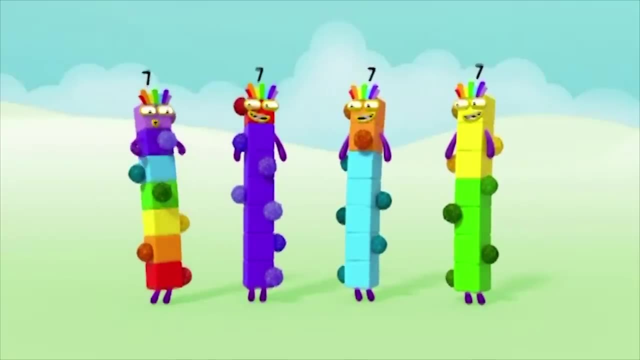 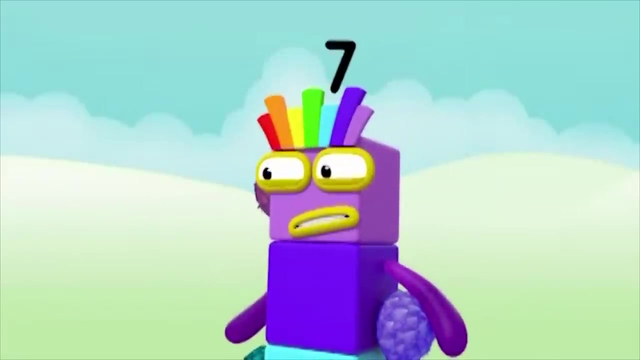 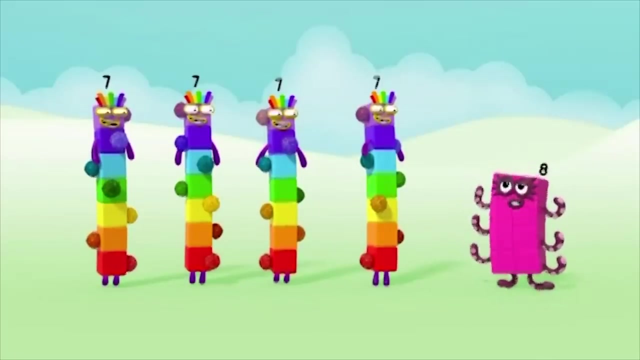 Three plus four equals seven. They've all stopped. We're so lucky. What do we do now? Oh Eight, Have no fear, Octoblock is here, Octoblock tickled. One, two, three, four, five, six, seven, eight. 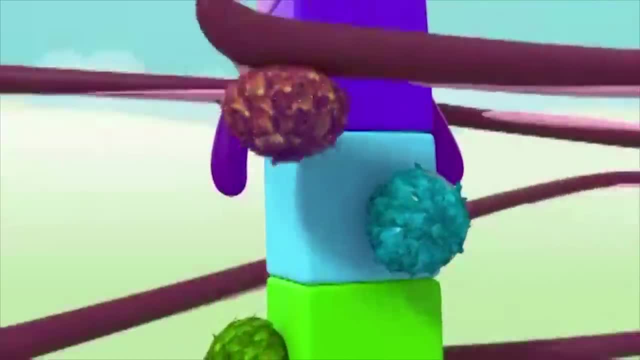 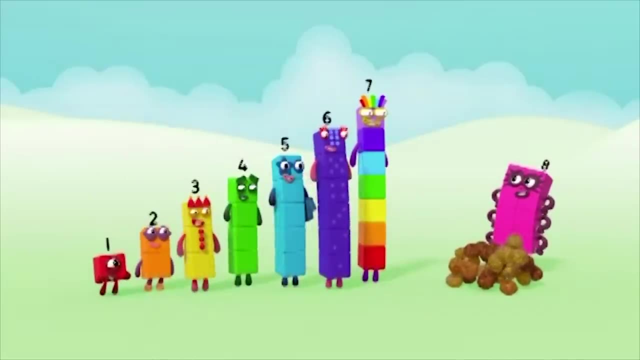 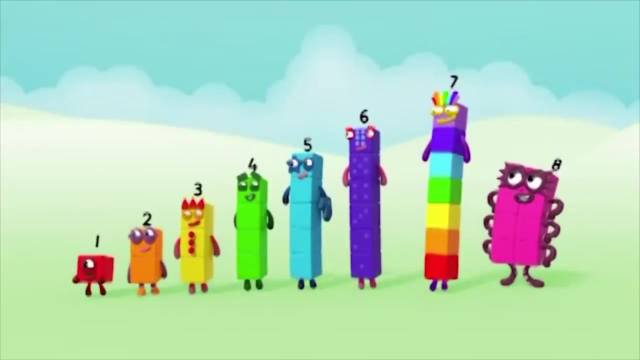 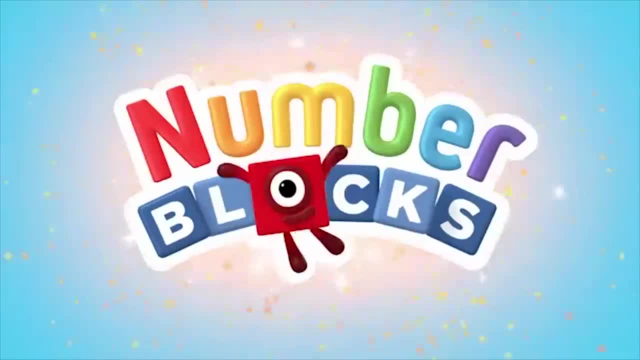 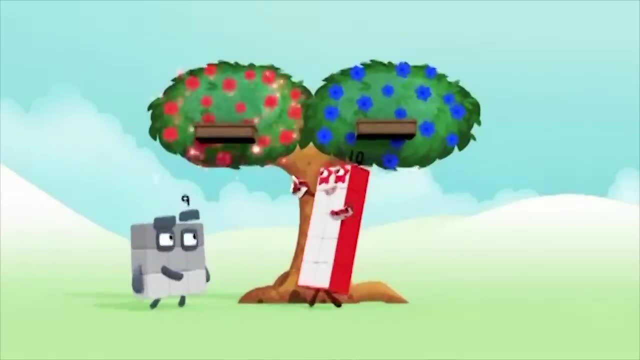 Ha, ha, ha, ha, ha ha ha. You can count on us with an Octoblock. Fancy a game of throwing twos. You be reds, I'll be blues. Sounds like fun. I'll draw a line. 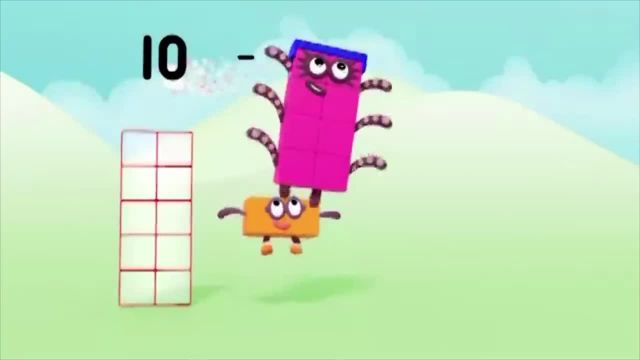 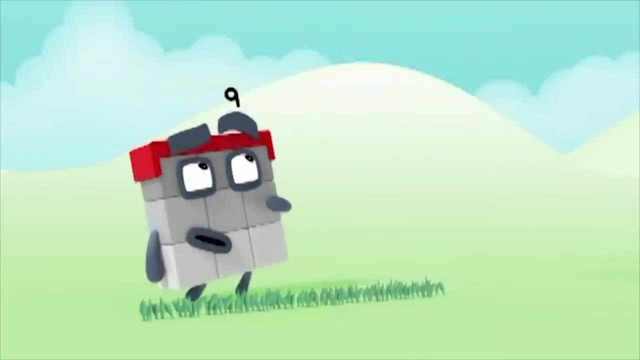 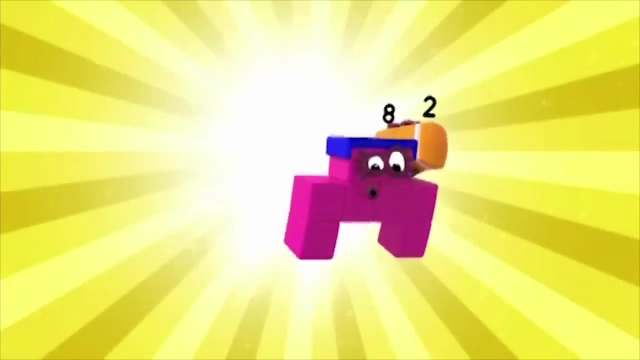 I'm bigger, so I'll start. Ten minus two equals eight. Ha ha, ha, ha, ha ha. Game on. Ready go Octoblock. play One, two, three, four, five, six, seven, eight. 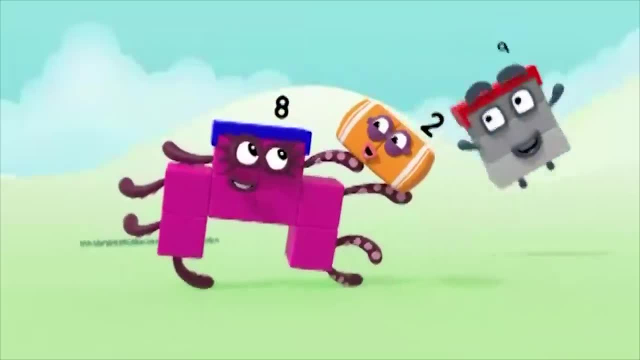 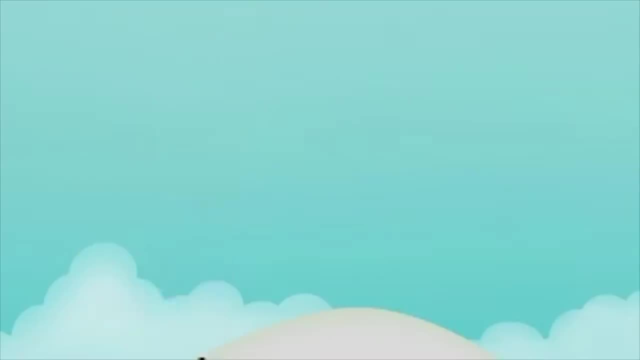 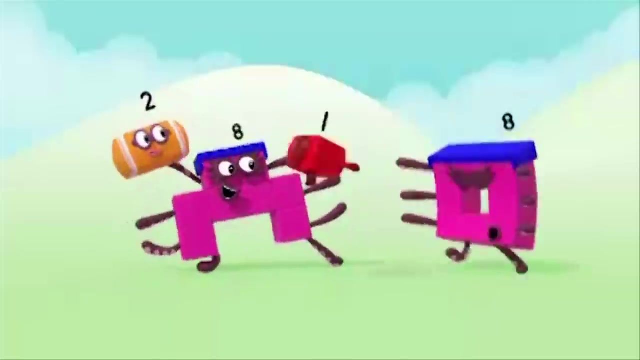 Play. He's on the left And now the right. He's on my head Now out of sight. Woo-hoo: Up high, Down low, Too slow. Ha ha, ha, ha, Achoo Whee. 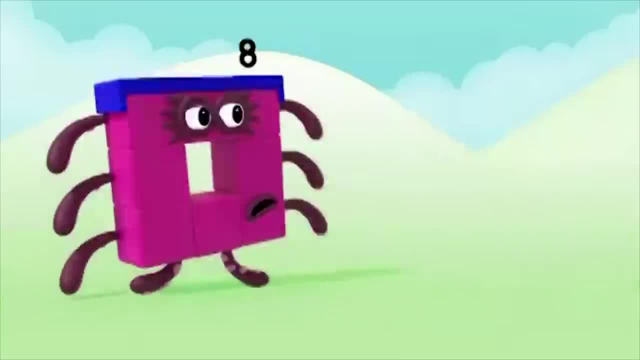 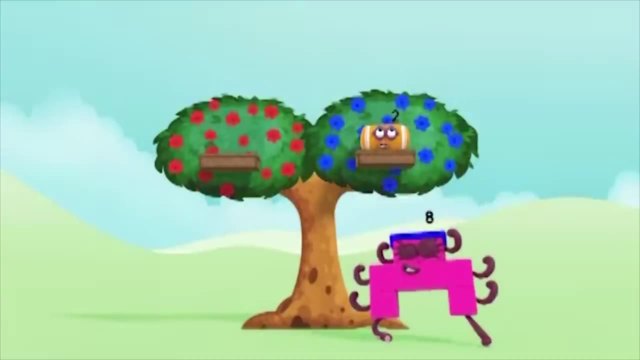 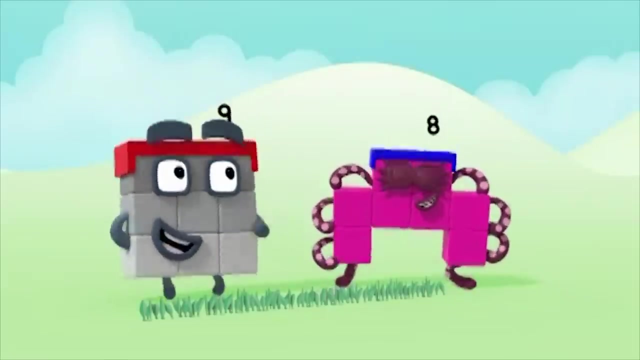 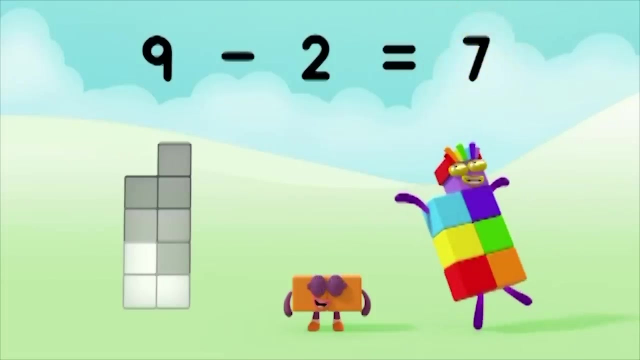 Whee, Hey, Huh Ha ha. Octoblock jump, Woo-hoo, Score Two points to blues. I'm bigger now, so it's my turn. Nine minus two equals seven. Ready go, Ha ha, ha ha ha. 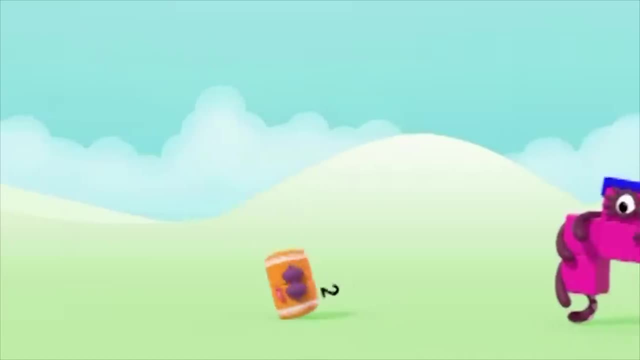 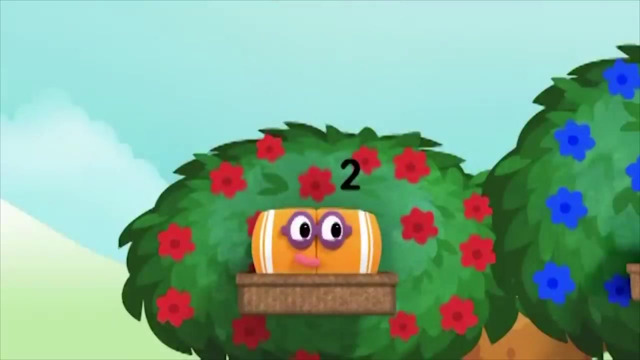 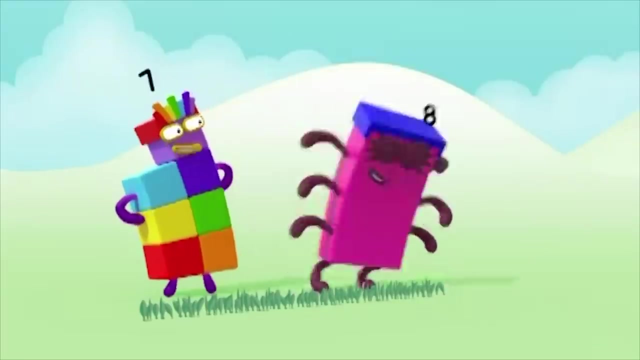 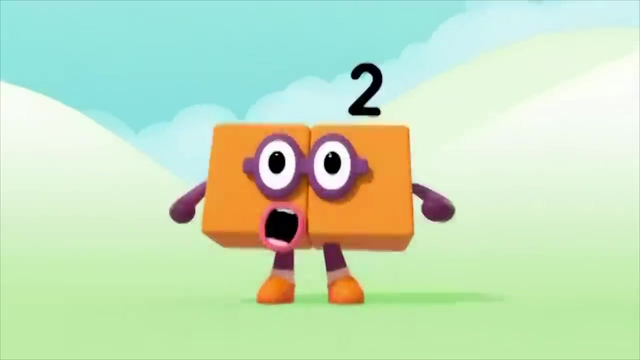 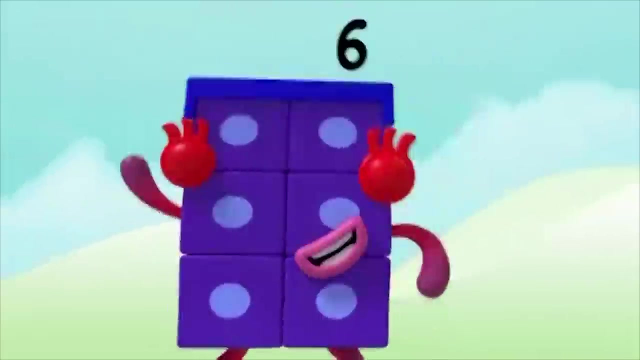 Ho, Two points each Beginner's luck. You're bigger, You start. Eight minus two Equals six. This game is nice. Let's roll the dice When it leaves my hand. how will it land? Um on six. 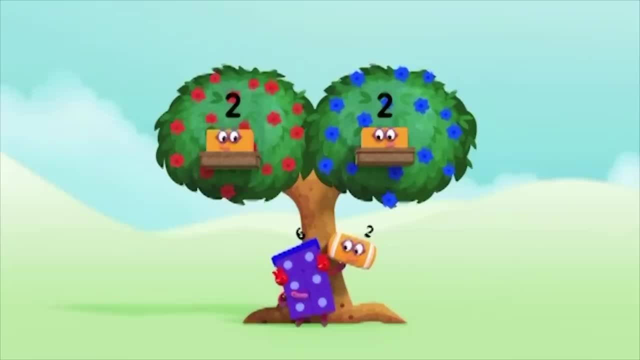 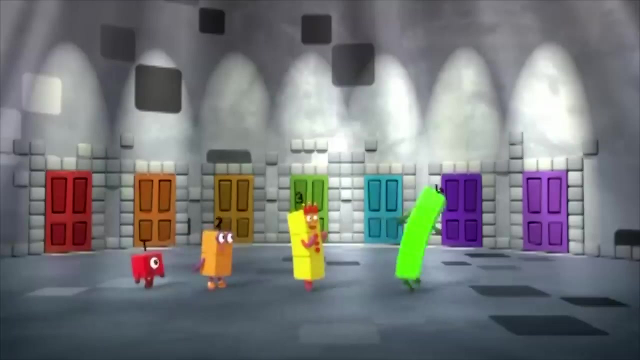 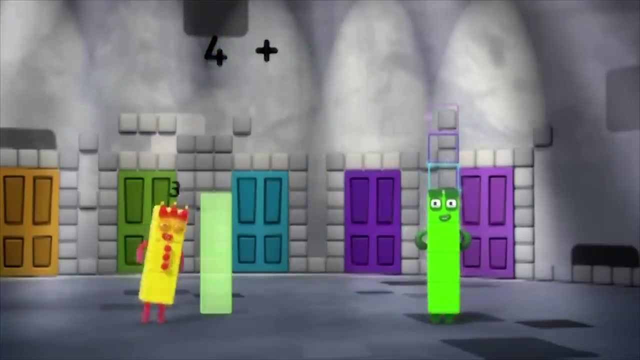 Oh, lucky me, Lucky me. Penalty, unfair distraction, Which means Four, two. You can count on us with another box, Seven doors. Which door is right? Maybe seven can help. How do we get seven? Four Plus three? 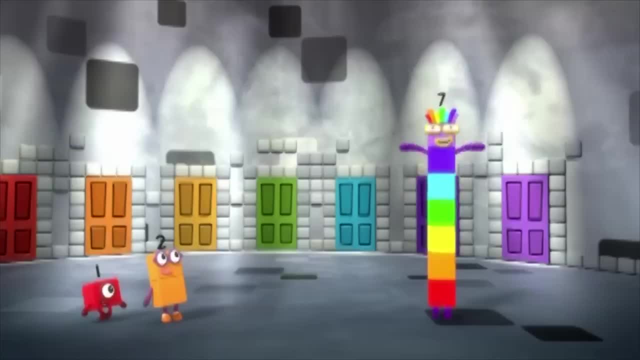 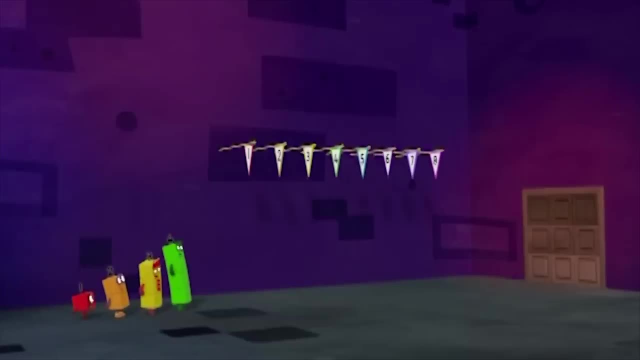 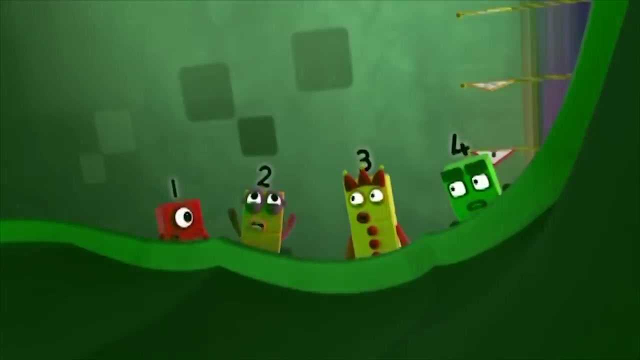 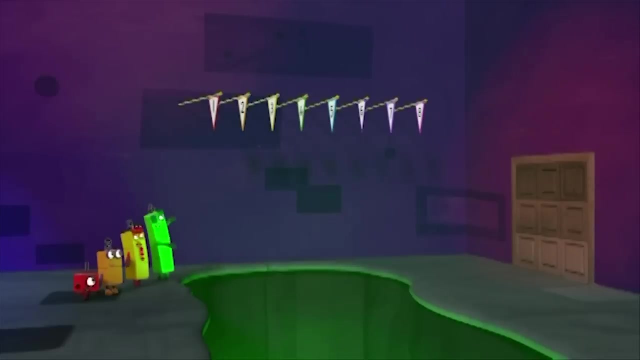 Equals Seven. Oh, I feel lucky This way. Easy-peasy, Look-a-measy, We're stuck. No, we're not. We could swing from the flagpoles. We'd need someone with very long arms to stretch that high. 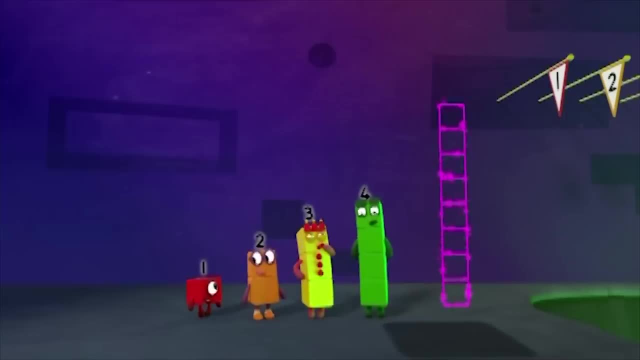 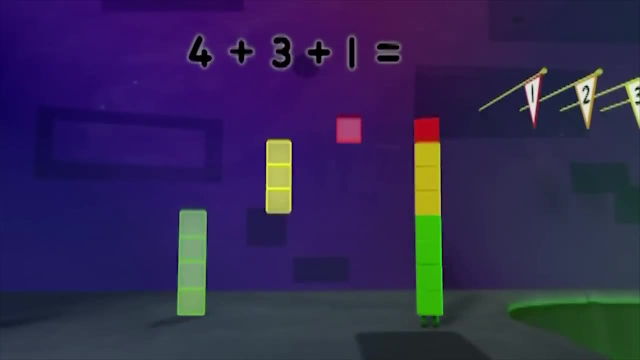 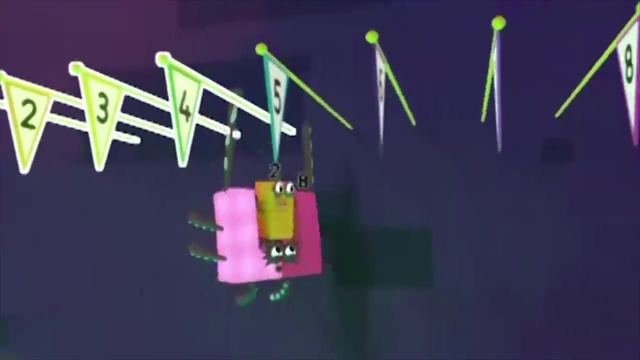 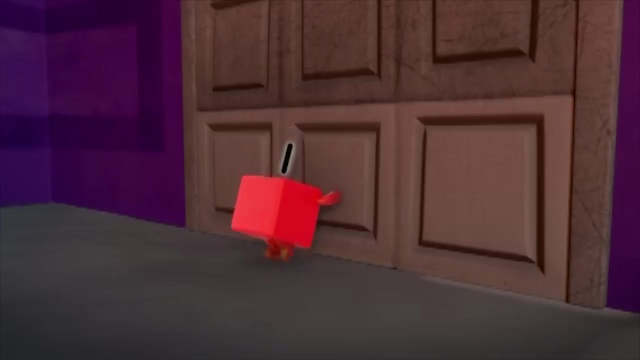 Eight. How do we get eight? Four Plus three Plus one Equals Eight. Octoblock swing Hooray. One, two, three, four, five, six, seven, eight Swing, It's stuck. 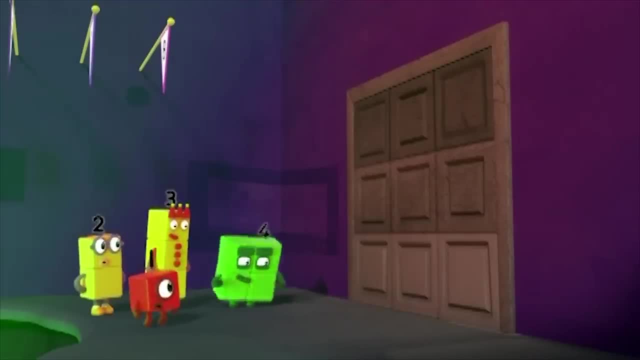 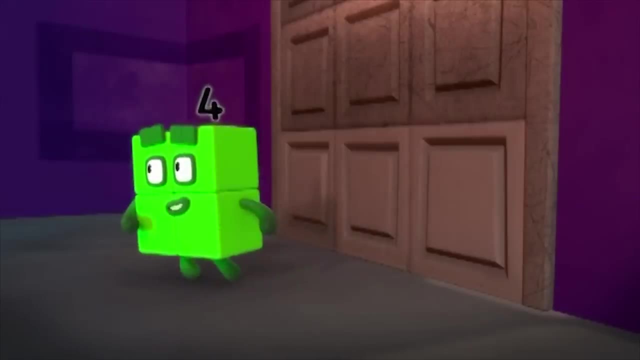 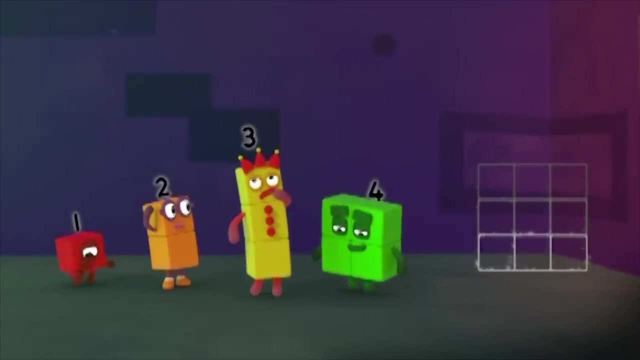 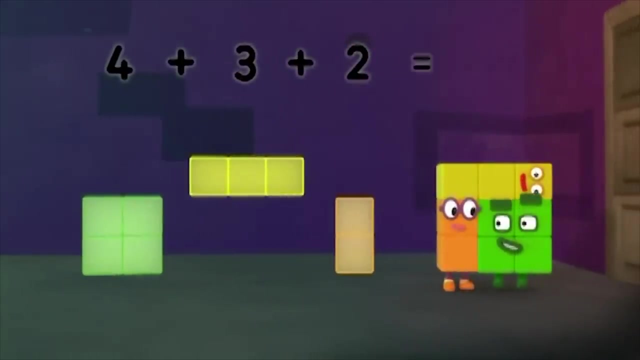 Squares are strong. Let me try. We need a bigger square. Nine: How do we get nine? Four Plus three Plus one Equals Seven. Four. Four Plus three Plus two Equals Two, Nine. 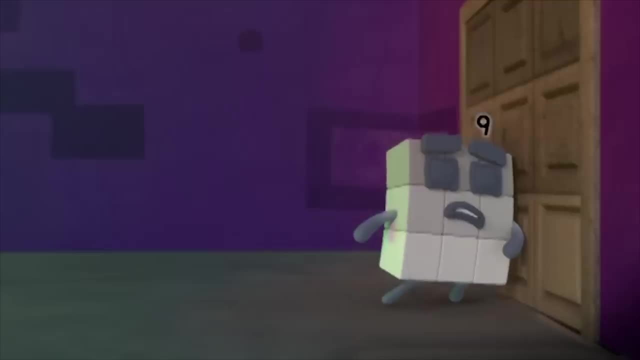 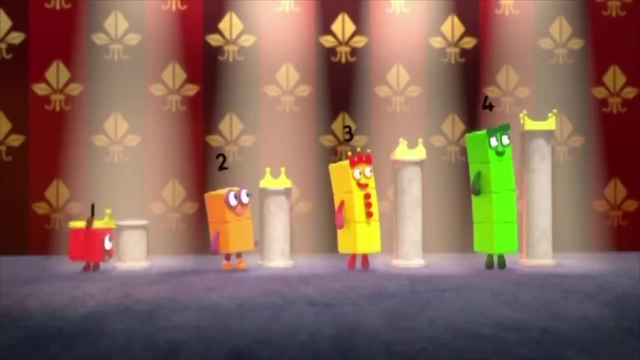 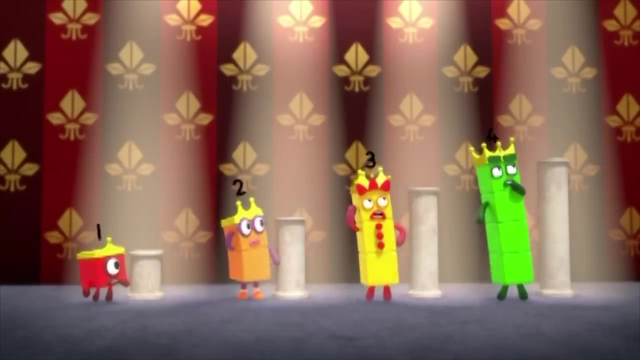 Yes, How do we get nine, Four Plus three Plus two Equals Nine. Thanks, Four. One, Two, Three, Four, Four crowns Crow. How are we going to get out One, two, three, four, five, six, seven, eight, nine, ten? 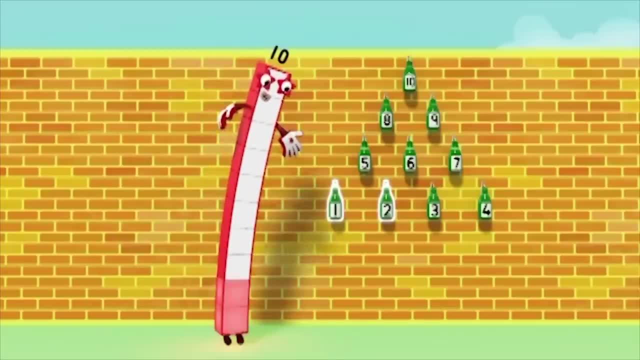 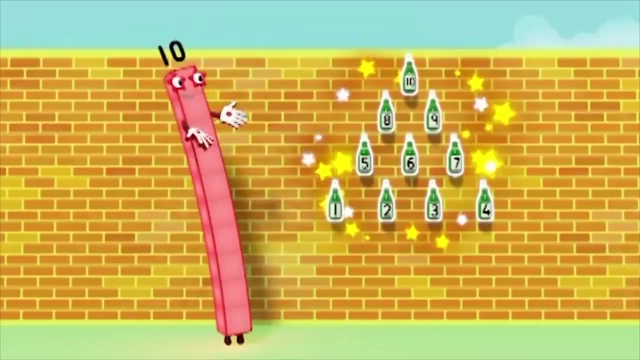 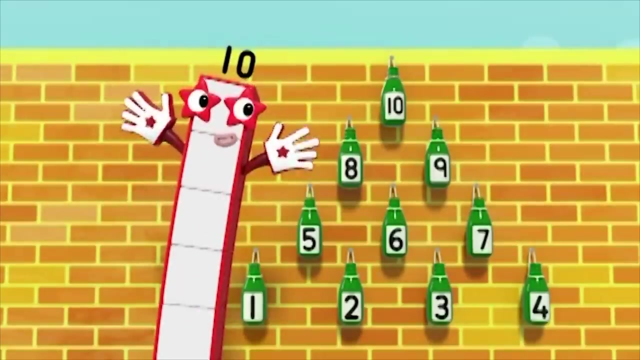 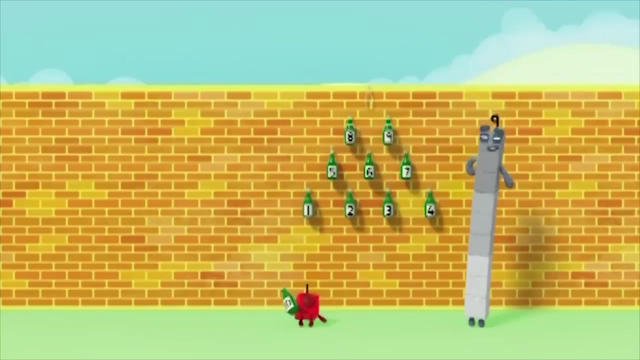 Ten green bottles. Ten green bottles: One, two, three, four, five, six, seven, eight, nine, ten. Ten green bottles hanging on the wall. Ten green bottles hanging on the wall. But if one green bottle should accidentally fall, 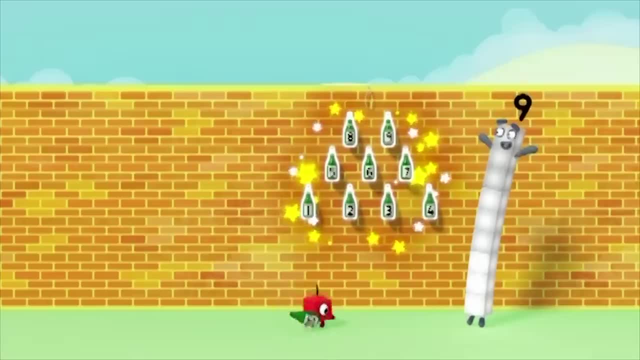 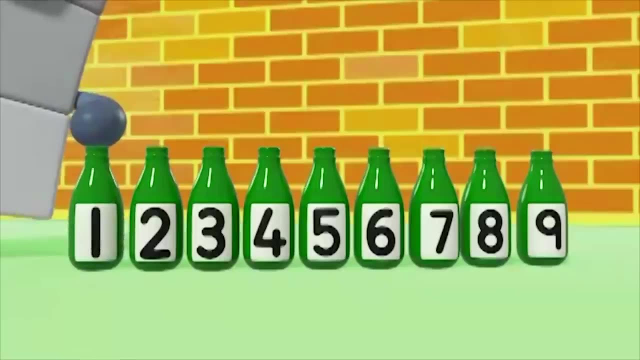 There'll be one, two, three, four, five, six, seven, eight, nine, Nine green bottles hanging on the wall. Better move these nine before they fall. They're not safe up there. Nine green bottles safely on the floor. 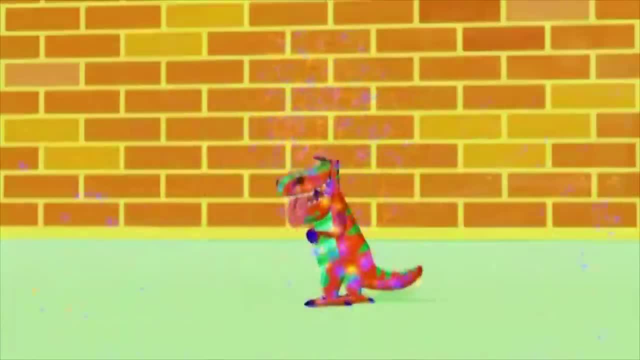 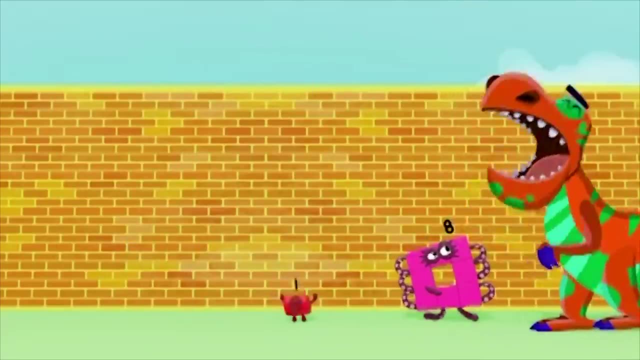 Nine green bottles safely on the floor, Oh Achoo. But if one green bottle becomes a dinosaur, There'll be one, two, three, four, five, six, seven, eight, Eight green bottles not safe on the floor.